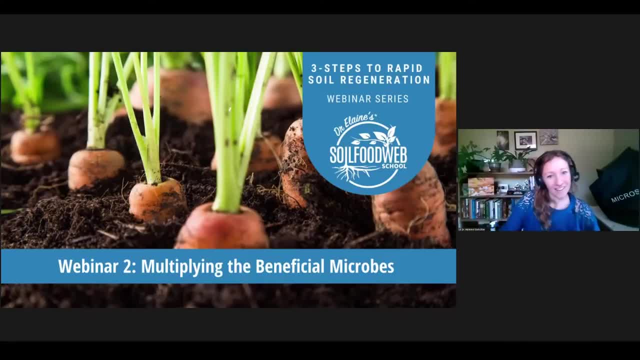 Hungary- Wonderful. This is awesome. Mexico Got some Aussies joining us. Thank you, Thanks for making the time zone work. Nice, Ireland- Oh, South Africa- Awesome. Thank you all for joining us Again. today we are doing webinar two: multiplying the beneficial microbes. 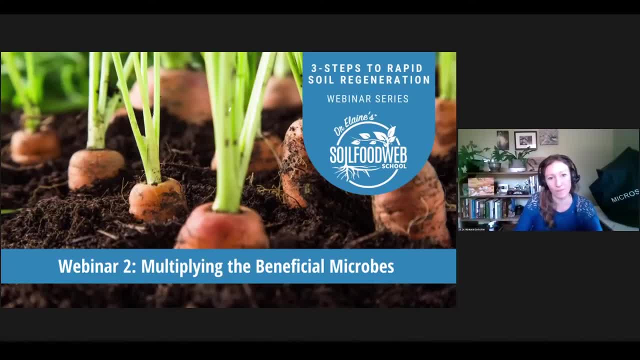 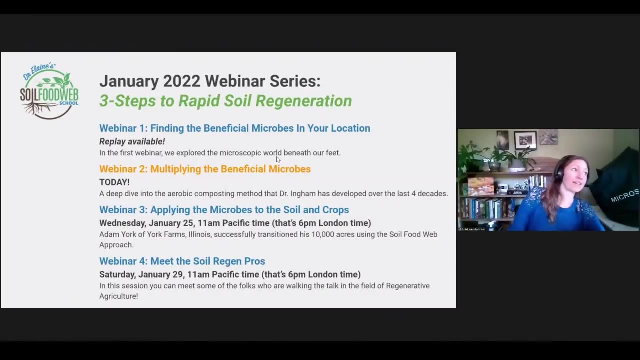 So keep introducing yourself. Where are you coming from? There's some from the Philippines, Indiana, South Africa, Very exciting. So, as an overview for our entire webinar series this month, we have already done webinar one: finding the beneficial microbes in your location. 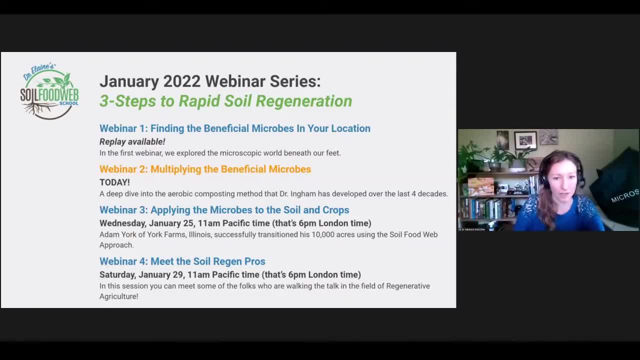 which we have a replay available. So if you missed that one, it's still possible to go and get to meet all of those fun organisms. We had a great discussion, So feel free to find that webinar replay. Today we are multiplying the beneficial microbes. 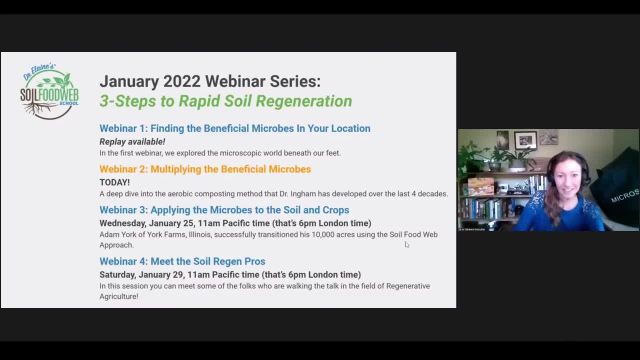 which I will tell you a little bit more about what that's about. But basically over the last four decades, Dr Elaine Ingham has perfected and worked with multiplying beneficial microbes in an aerobic composting method, And we'll talk more about that. 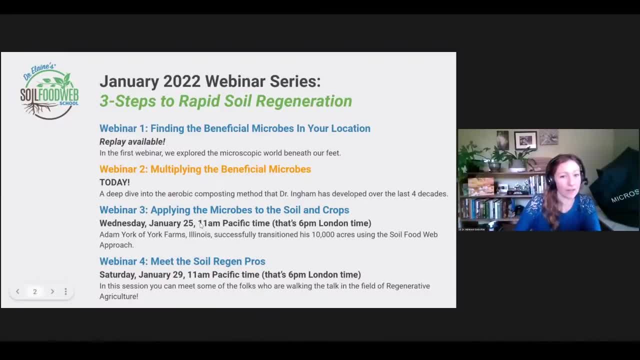 And January 25th we have webinar number three, which is going to be very exciting. It's called applying the microbes to soil And this is going to be Adam York joining us with Todd Harrington talking about the project in which they successfully transitioned 10,000 acres using the Soil Food Web. So that will be on January 25th. 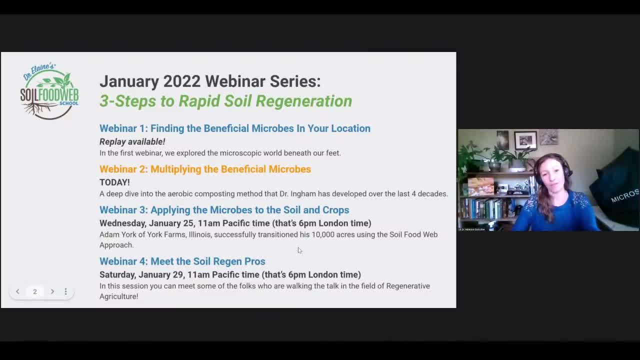 On January 29th we have our final webinar of this series called Meet the Soil Regen Pros. So come meet more of the folks who are doing this great work of getting soil regenerated into biological systems. All right, Thank you all for joining us. Let's see we have some more from Germany. 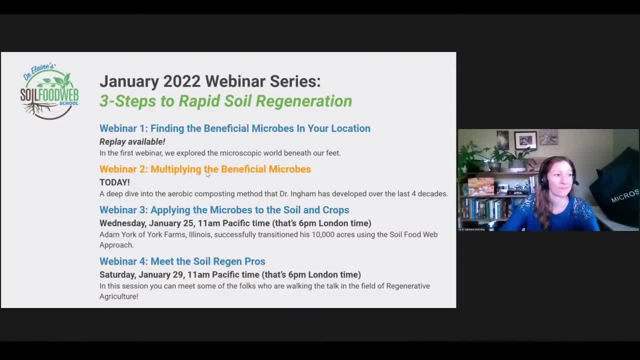 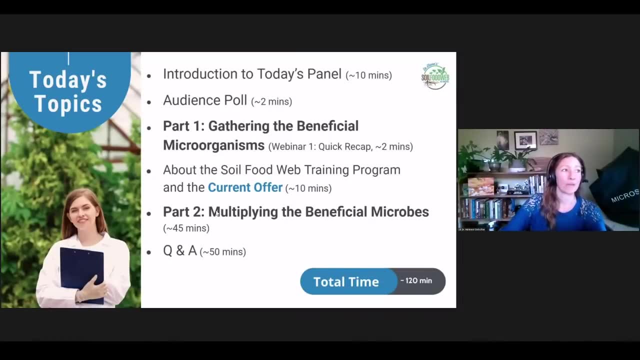 from Canada. I love our global reach, So today we're going to start by introducing everyone. We have a brief poll And then we'll start. Part one is going to be a recap of how to gather and bring together the beneficial microbes. We'll have a brief session to talk about our current 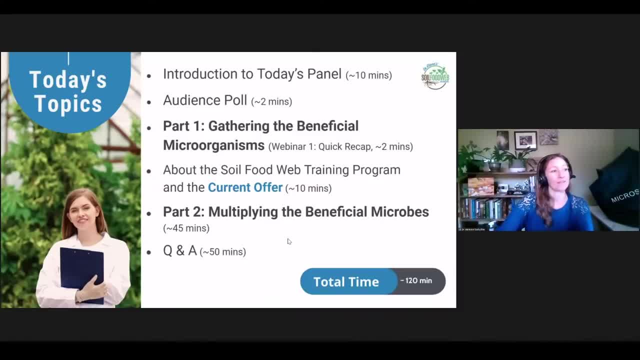 offer that we have, And then part two is going to be multiplying the beneficial microbes, And then we'll get into some Q&A. So, speaking of Q&A, if you have questions there's a separate Q&A option. I have another slide that'll show you exactly where that is, But the chat is where you're. 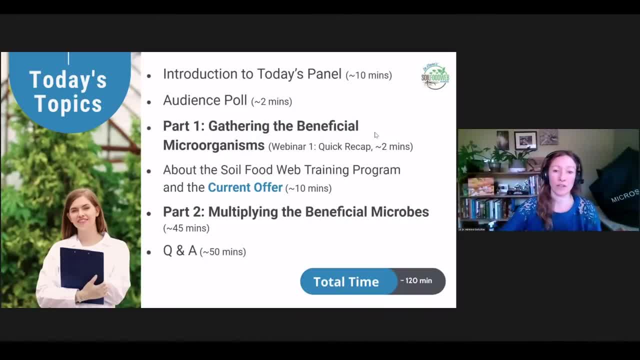 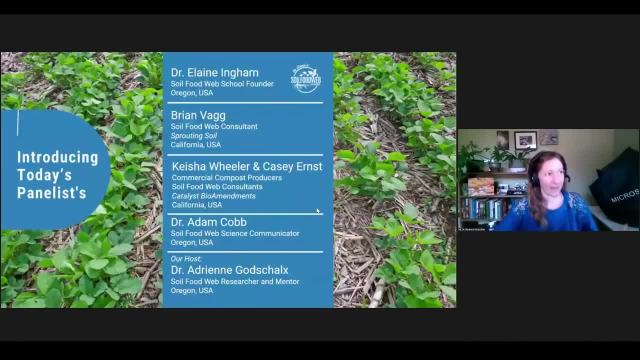 all saying hello right now, And the Q&A is where the questions for us to consider for our webinar today. That's where those will go. Let's get started. Okay, So we have Dr Elaine Ingham herself joining us once again. She is the founder of the Soil Food Web. 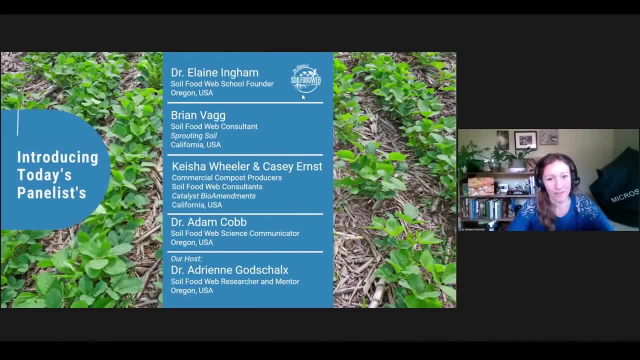 School and a brilliant scientist, brilliant woman, And I'm so excited to learn more from her. today We have Brian Begg, who is a Soil Food Web consultant, who has his own company called Sprouting Soil. He has been based in California but has recently relocated up. 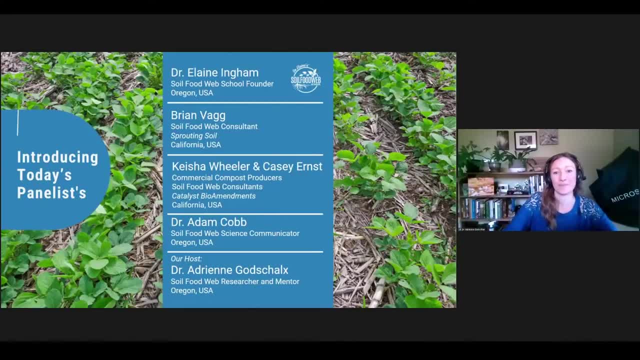 here to Oregon by Newport. So if you're excited about having him regenerate some soil, he's now up in the area and you're in Oregon. We have Keisha Wheeler and Casey Ernst, who are both commercial compost producers and officially Soil Food Web consultants. 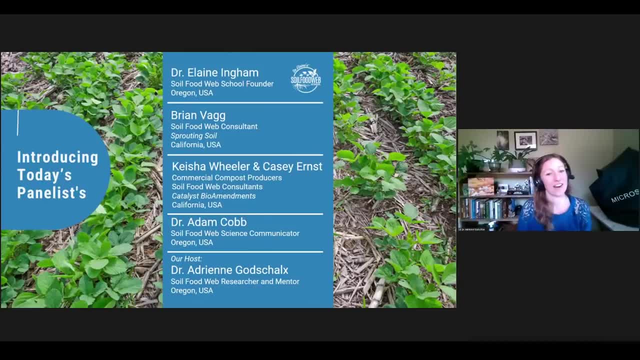 Congratulations. So great to have our graduates out there and doing good work in the world. We have Dr Adam Cobb, who will be joining us too. He is one of our resident mycologists but also a brilliant science communicator, So always a pleasure to speak with Dr Adam. 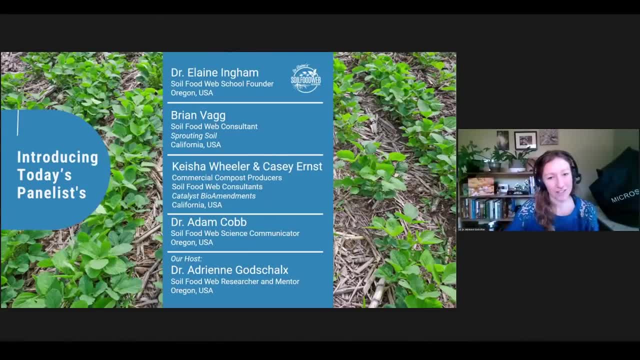 Cobb And myself. I am Dr Adrienne Gottschalks. I am here as your host today And I'm sure I won't be able to keep myself from talking about the compost as we're going, as I am also a Soil Food Web School mentor and researcher. Let's get going. 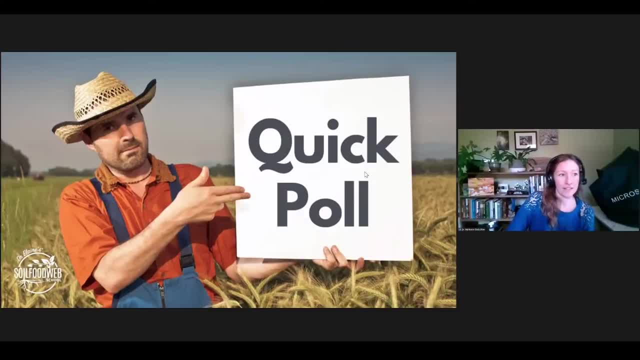 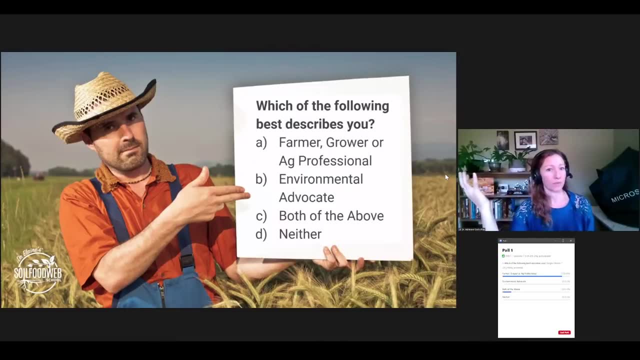 So our quick poll in the webinar today is this question: You should have a window pop up that asks which of the following best describes you: Brewer or ag, professional Environmental advocate. Both of the above or neither, And this is partly helpful so we can steer our conversations. 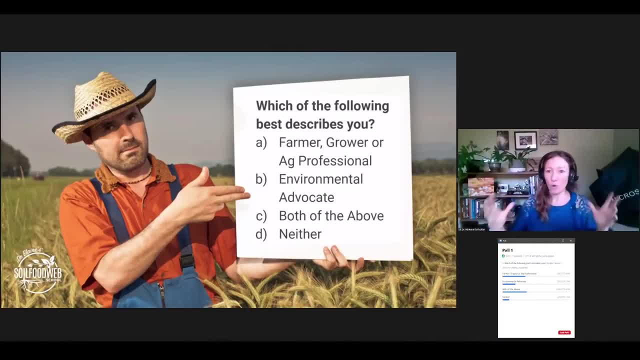 in the direction geared more towards folks who are thinking about larger swaths of land or more folks who are considering going out there into the world and communicating these concepts, Or if you know it's both in tandem, or if you come from a totally different. 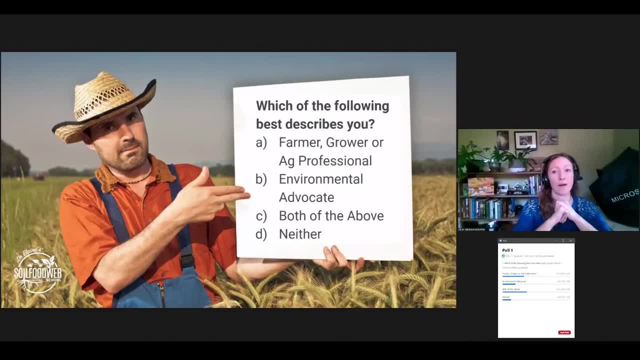 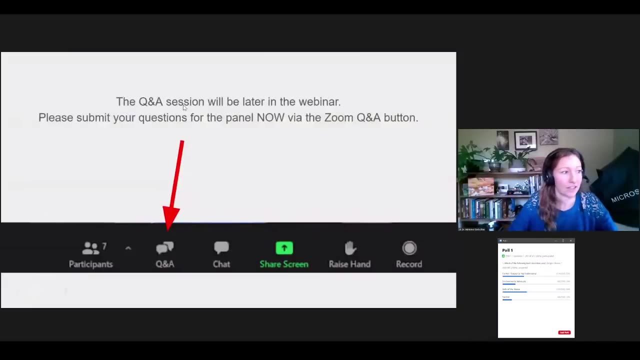 perspective. It's all good for us to understand, as we're talking about how to multiply microbes. So fill out this poll and we'll get some results here in a moment. Speaking of Zoom, the Q&A button looks like this. So the chat where you're filling out your 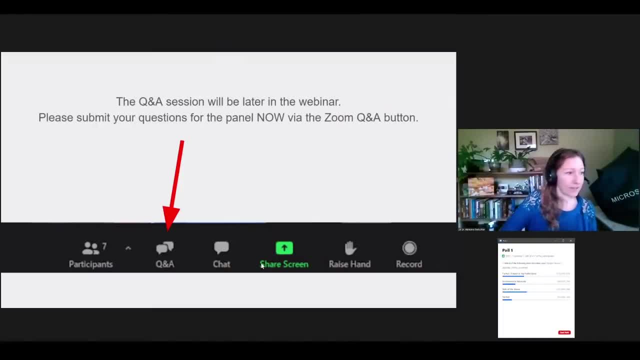 initial welcome is the main chat feature, The Q&A. if you have a question that you would like our panelists to discuss today, feel free to enter that into the Q&A. This is where we will pull from at the end. All right, so let's first hear about the three steps to rapid soil regeneration. 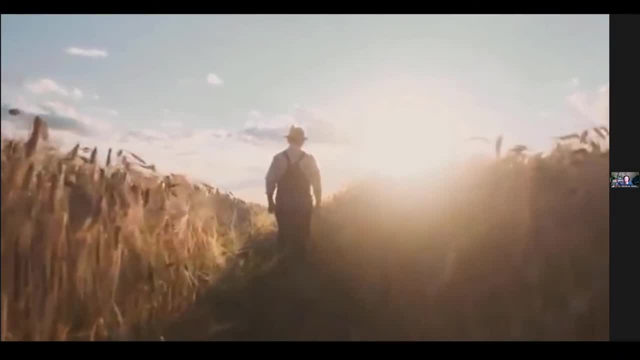 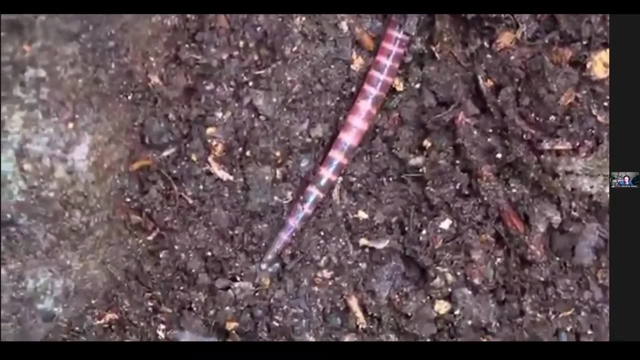 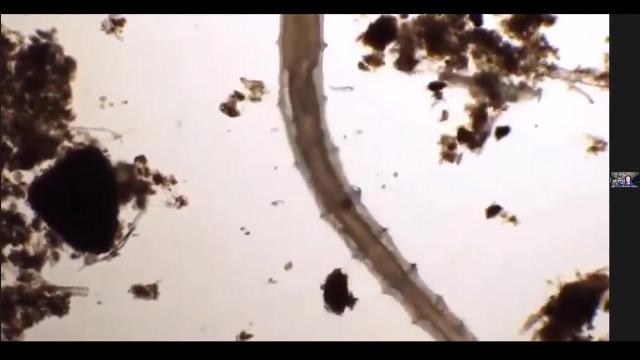 There are many people experimenting with soil regeneration practices around the world, and different techniques can be effective in improving soil health. The essence of soil regeneration remains the same no matter where you are: It's driven by the soil microorganisms. They are at the bottom of the soil food chain or the soil food web, so the rest of the 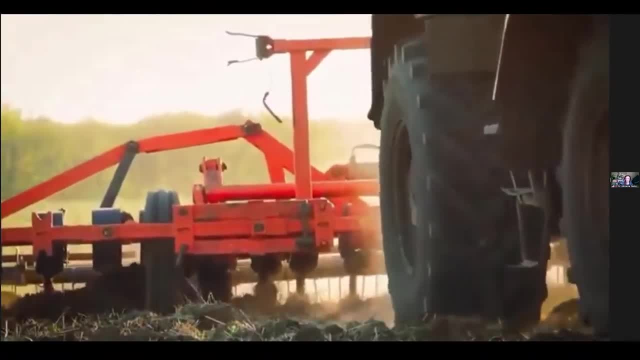 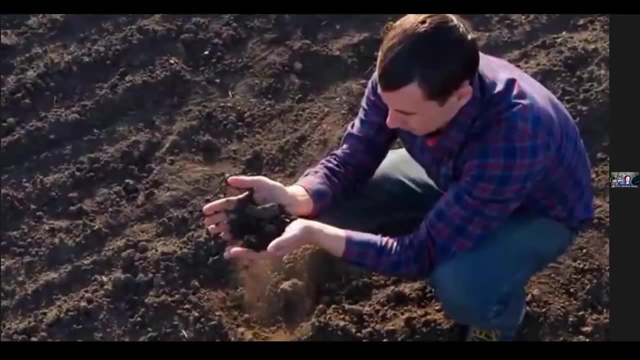 ecosystem depends on them. Intensive agricultural practices, such as tillage and the use of chemicals, have a devastating effect on the fragile microorganisms that make things function in a healthy soil. So how can you restore this delicate ecosystem to your soils And how do you ensure 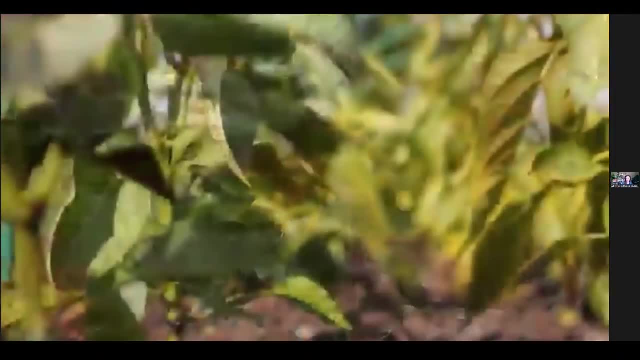 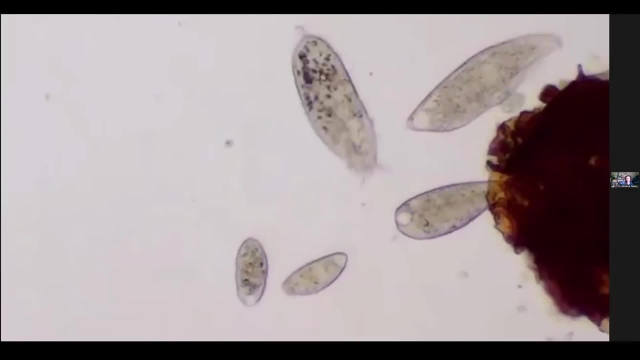 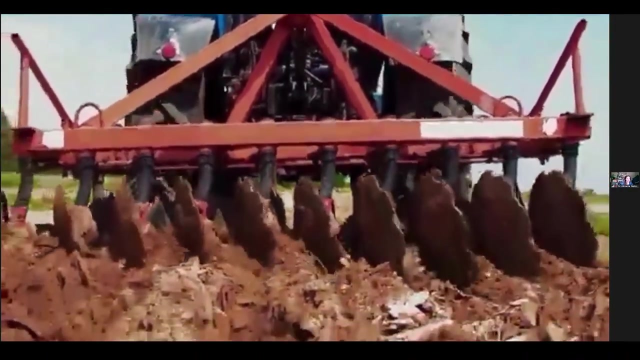 that it remains protected over time. The process is probably a lot less complex than you think. Beneficial microbes are out there on the land all around you, but the ecosystem is out of balance due to modern agricultural practices. So how do we put things right? Step one is collecting a wide 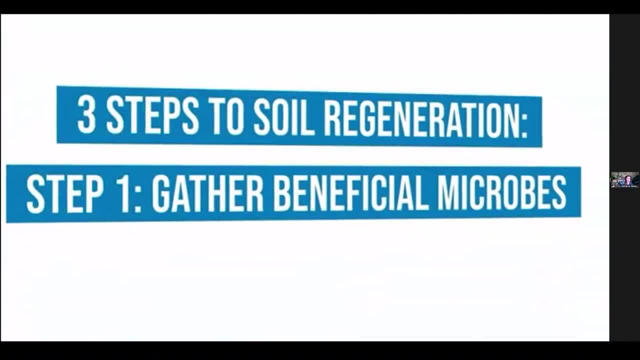 diversity of organic matter that hasn't been sprayed with chemicals. There will be beneficial bacteria and fungi and other microbes on the surface of this organic matter, as it is their main food source. Step two is collecting a wide diversity of organic matter that hasn't been 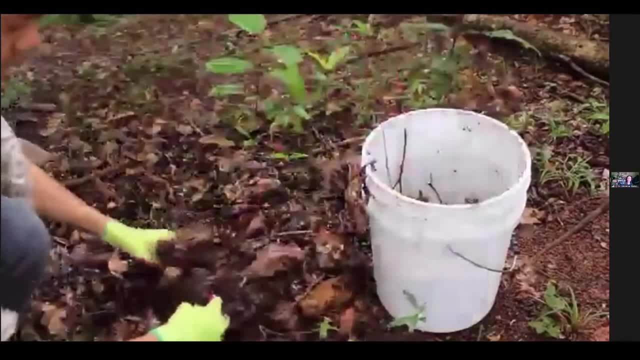 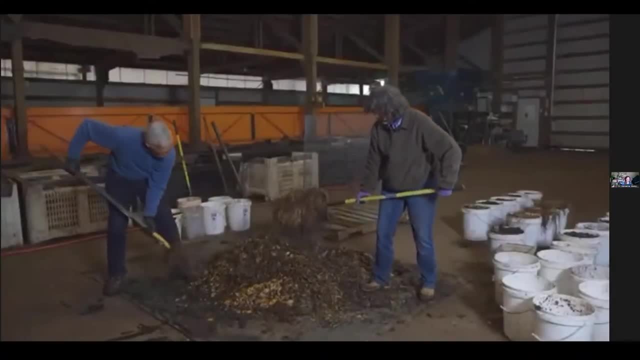 sprayed with chemicals, There will be beneficial bacteria and fungi and other microbes on the surface of this organic matter, as it is their main food source. Once we have collected our critters, it's time to multiply them in step two of the process, Using the close control composting method that Dr Elaine Ingham has developed over the last. 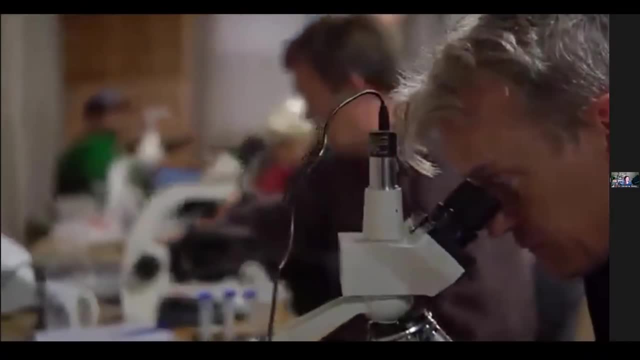 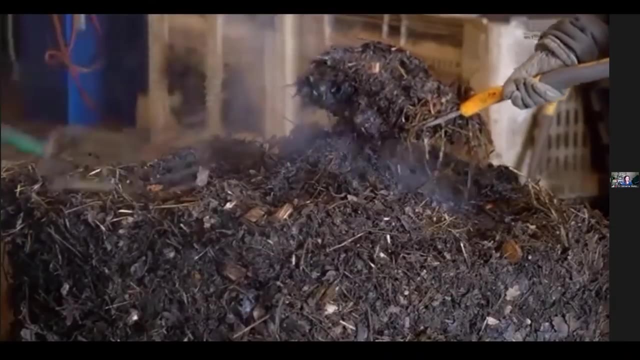 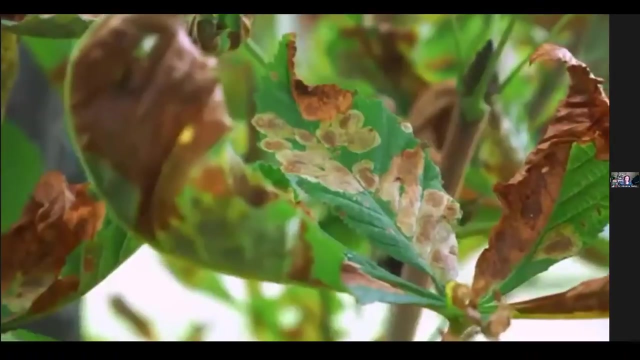 four decades. we monitor the biology using the microscope and we take steps to ensure that the moisture, oxygen and temperature levels in the compost are kept within the limits that favor beneficial microorganisms. This ensures that, while the desirable microbes are feeding on organic matter and multiplying, disease-causing microorganisms are being 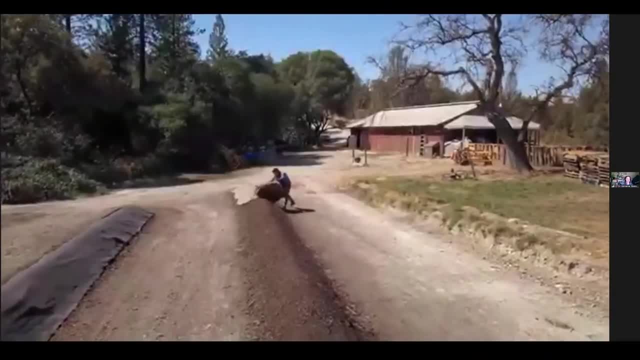 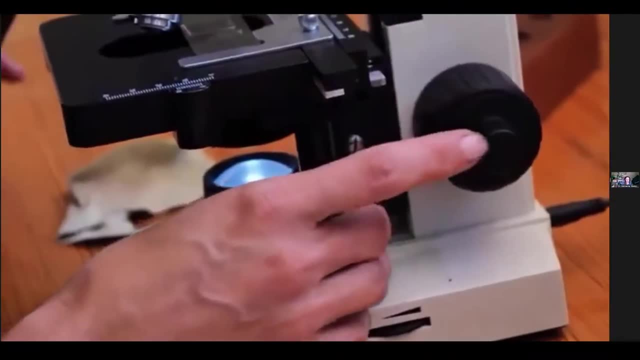 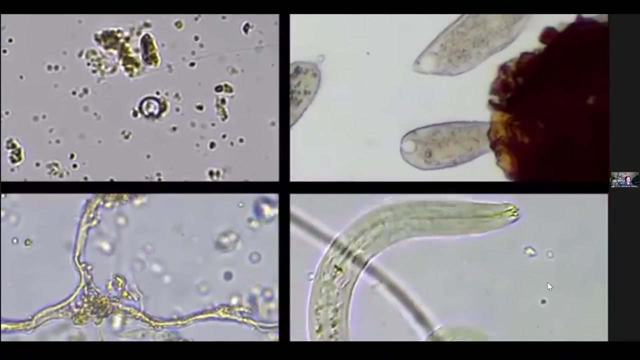 destroyed or going dormant. Once the composting process is finished, after about 28 days, we assess it with the microscope and then use certain techniques as required to balance the four major groups of beneficial microbes of a healthy ecosystem: Bacteria, fungi, protozoa and nematodes. 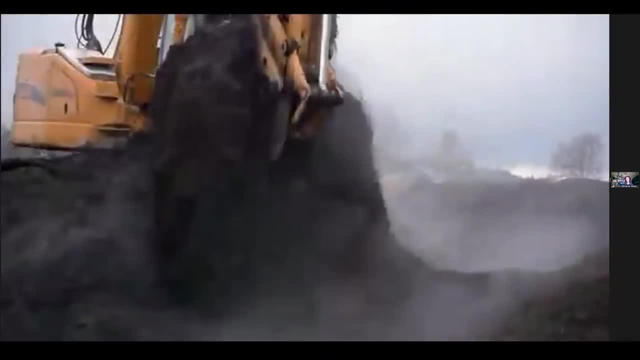 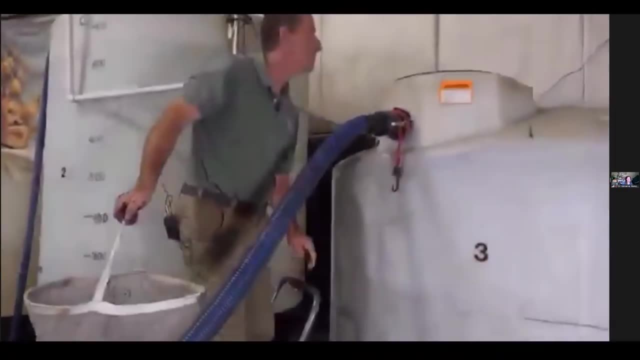 need to be represented in certain proportions in the compost in order for it to be considered biologically complete and to ensure the successful inoculation of your soil. We then make liquid inoculants called extracts, and tea leaves into the composting process. The composting process is 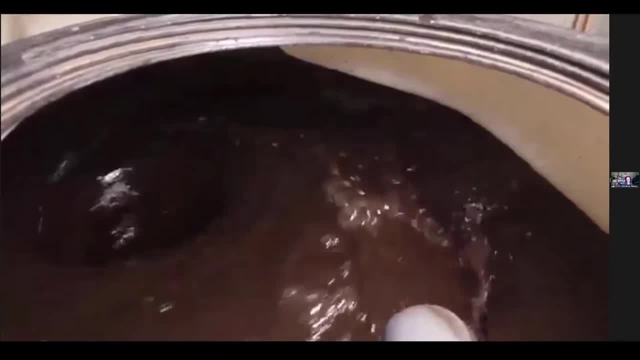 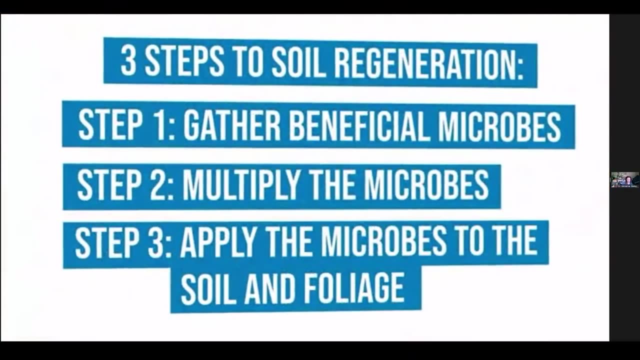 a process in which we extract extracts and teas from the compost, which can make it easier to treat the soil and plants in many circumstances. In step 3, we inoculate the soil and foliage with microorganisms. Soil can be treated with either biological compost or liquid extracts, Using 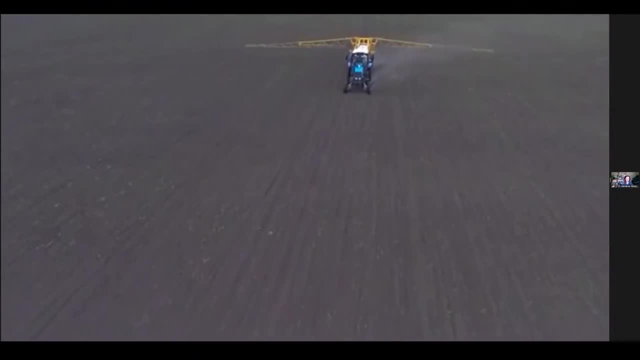 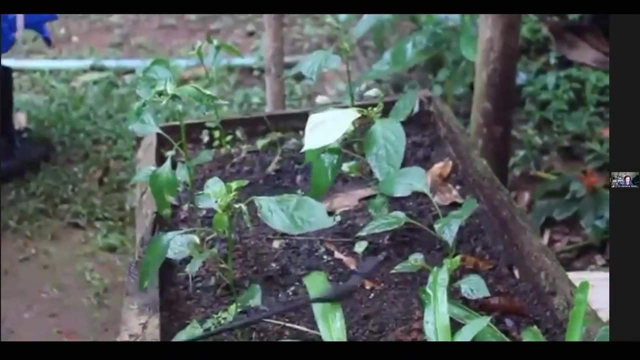 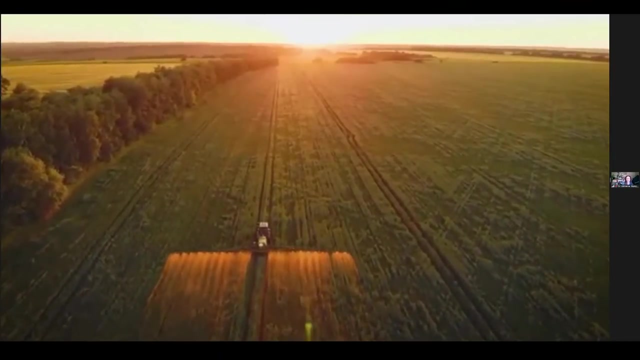 liquids can make application easier on a large scale and can be achieved using conventional spraying equipment. Biological teas are ideal for foliar applications as they contain natural glues which enable the microbes to stick to the above-ground parts of the plant. Coating foliage with beneficial microbes can protect your crops against infection by disease. 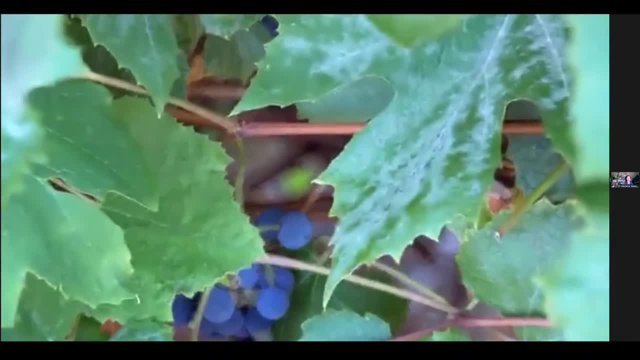 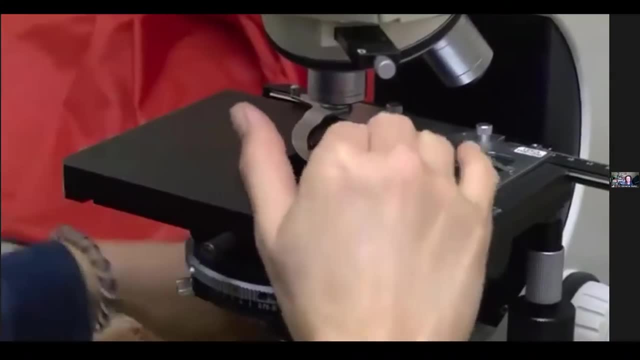 causing organisms like blight, leaf rust and mildew. Once the inoculant has been applied, we can continue to use the microscope to track the progress of the biology in the soil and on the surfaces of the plant. This informs us on when further treatments may be required Generally, 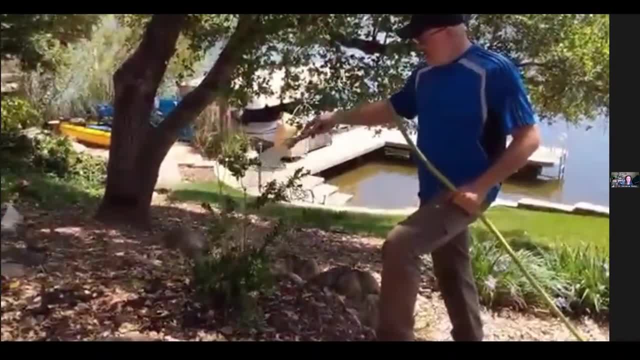 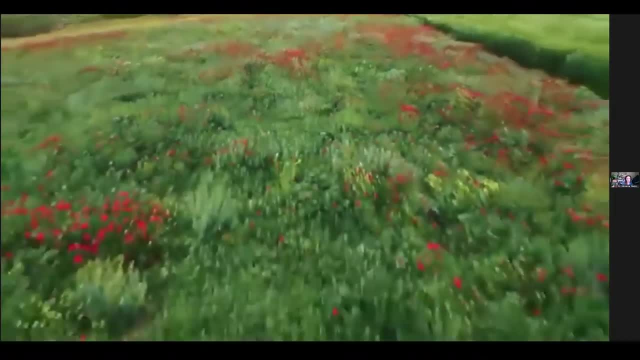 speaking, once inoculated, a soil may not require reapplication for several months or even years. The adoption of regenerative practices like the use of organic fertilizers, or the use of organic fertilizers like no-till and the use of cover plants is very important in ensuring the survival. 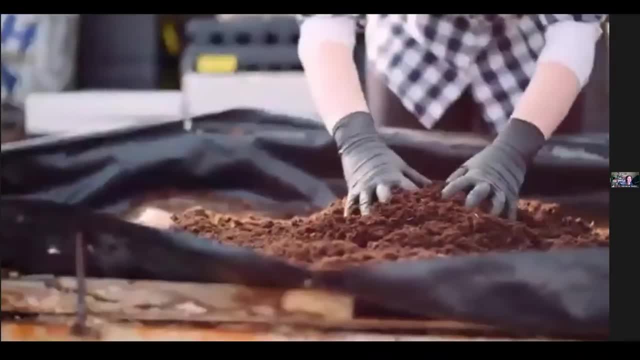 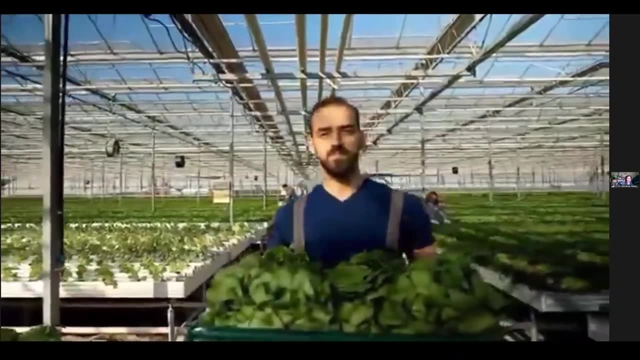 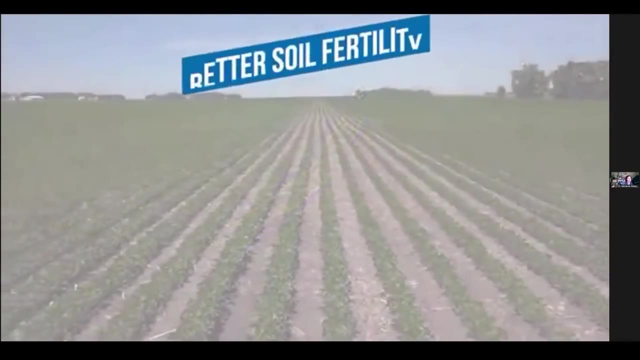 of beneficial microbes in your soil. We train our students how to successfully implement these techniques in many different conditions and on different crop types. Whatever you grow, you can be sure that having a healthy soil microbial community in place will provide several benefits. These include better soil fertility, increased resistance to pests and. 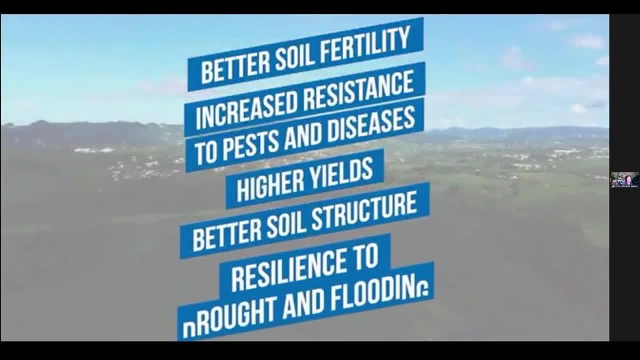 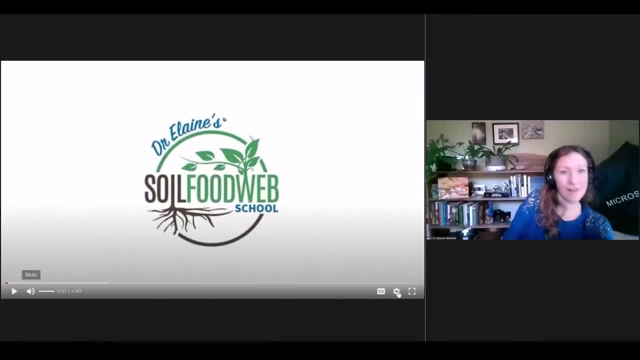 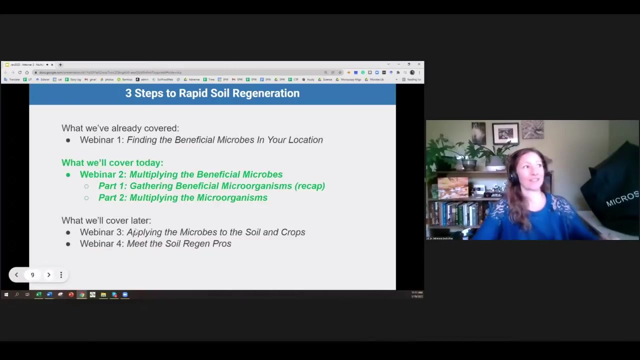 diseases, higher yields, better soil structure and resilience to drought and flooding. We have already covered in our last webinar finding the beneficial microbes in your location And today, now let's jump in. We'll give a brief recap on how to gather and collect those beneficial. 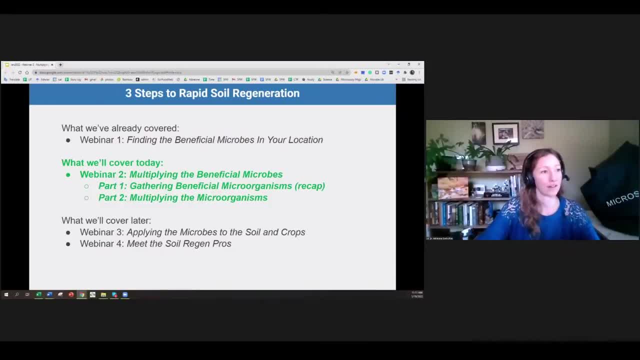 microorganisms from the starting materials that you can find in your area, And then we'll jump into multiplying the microorganisms Again. in our future webinars we'll talk about applying the microbes to soil and crops, as well as getting to meet those soil regen pros. 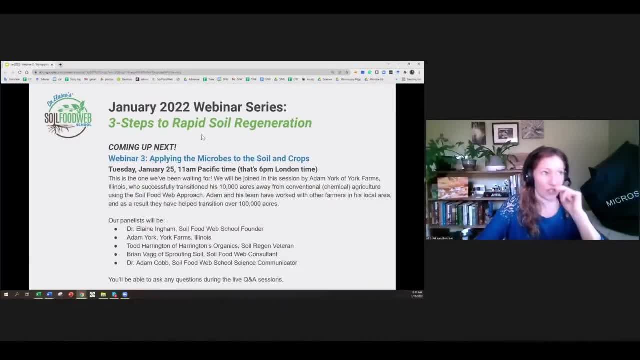 So, just as the next one getting to apply microbes to soil and crops, A little bit more information about that upcoming one. on January 25th We will have Adam York, Todd Harrington, Brian Bagg and Dr Adam Cobb all joining us together to talk about the full transition. 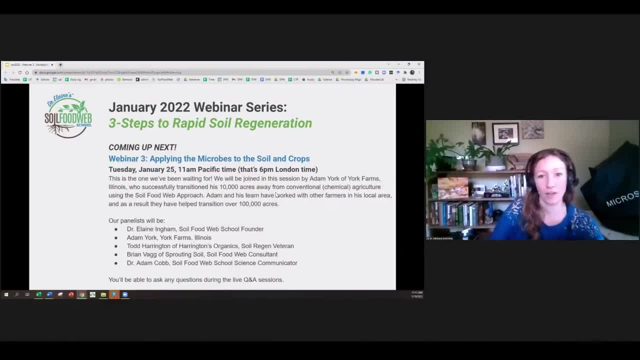 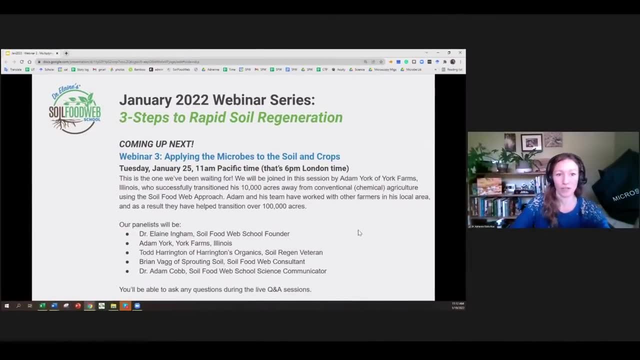 from 10,000 acres, away from conventional agriculture into a biological regenerative agriculture, and show all of the benefits that Adam York has experienced in that transition. So mark your calendars for January 25th, All right? So here's a brief recap, just so that everyone's on the same page. 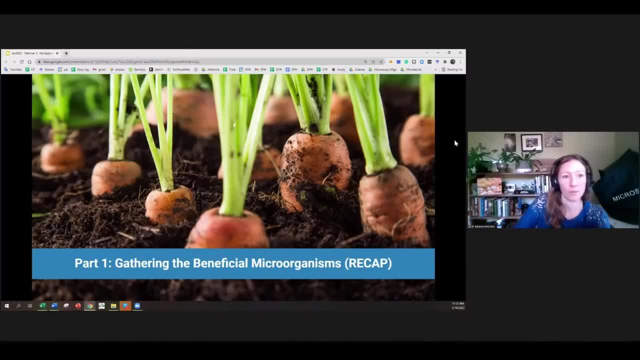 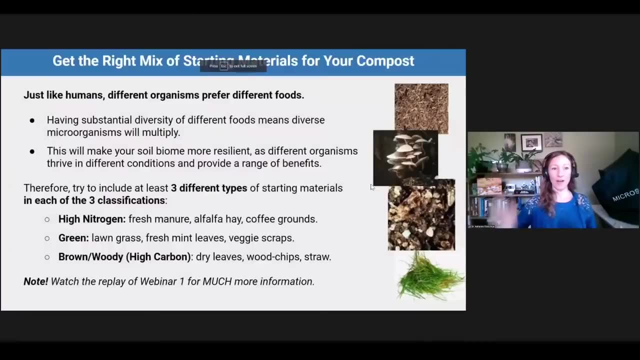 Let's see, And I will pass this off to Dr Adam Cobb. I don't know why my. Here we go, Dr Adam Cobb. Drkeysha Letsya. All right, Thanks, Adrienne. So, as Adrienne has mentioned in the first webinar, that's output to: 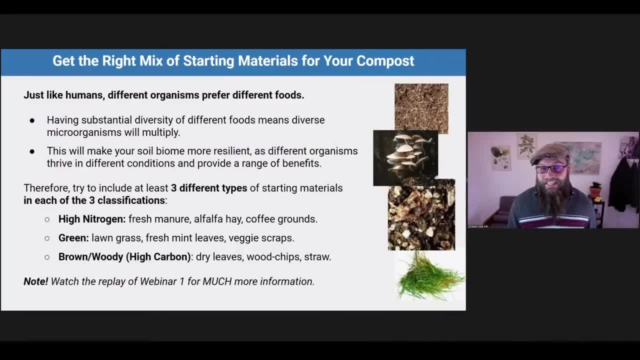 everybody. these topics are covered in a lot more detail. I'm trying to give you boil this down into our key take-home messages, And really what we emphasized is that if you want to get a diversity of microorganisms in your compost pile, you need to think about a diversity of foods for 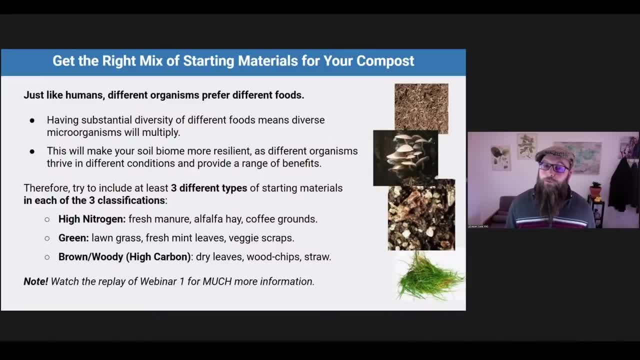 organisms, And so, as you collect these things from especially local environments, be thinking about bringing multiple kinds of material into your compost pile, And that will just lead to a more robust and resilient microbiome in your finished product. So we define those materials in three categories. 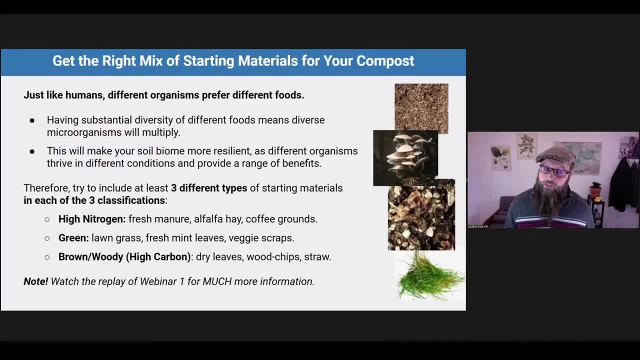 here at soil food web school high nitrogen, green and brown or woody material, And so you see a few examples there from each category And I won't belabor this point, But the information is out there from our previous webinar And I'm 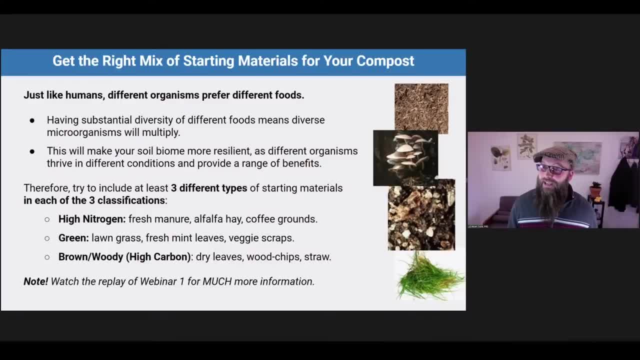 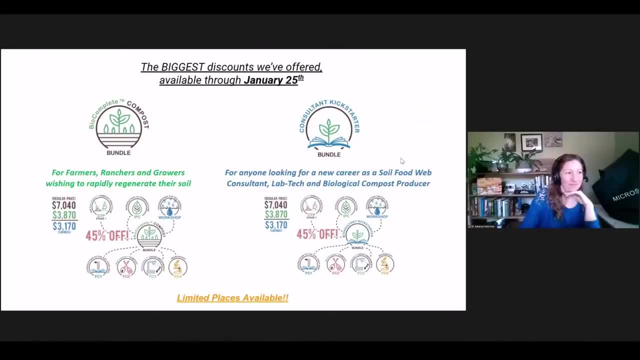 sure Dr Elaine will will cover some more details today. Thanks, Adam. And just as a reminder, we still have a few spaces available in our discounted programs. Awesome savings: up to 40% off on our various programs And this deal ends on January 25.. So if you're, 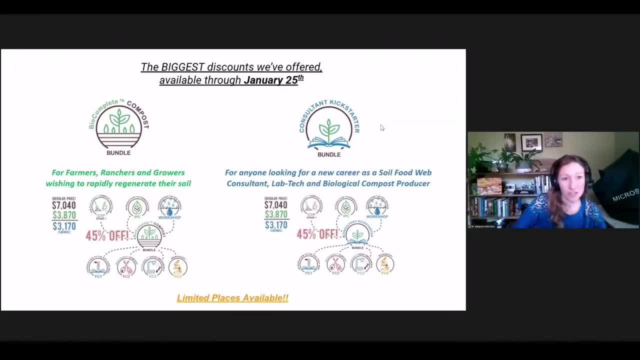 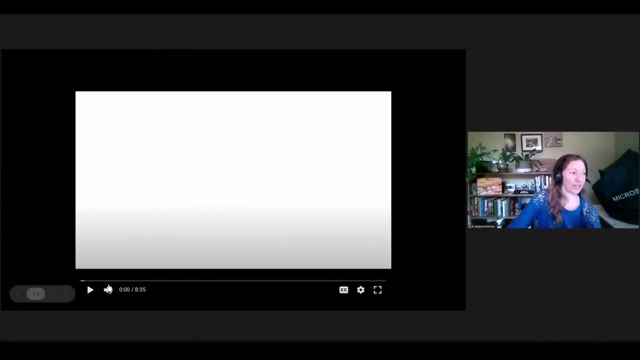 interested you can and you want to ask more questions, feel free to email us at info at soil food webcom, And here's a little bit more about what those programs can allow you to do, And then we'll jump into making compost with Dr Elaine. 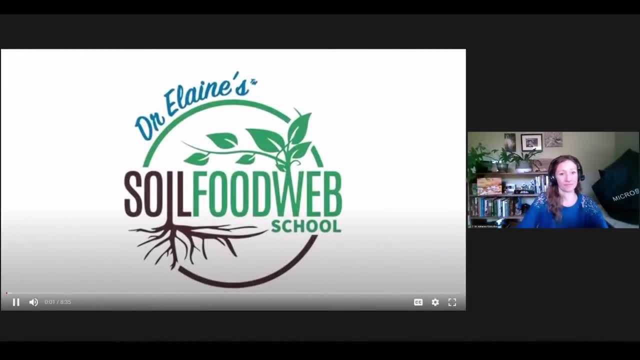 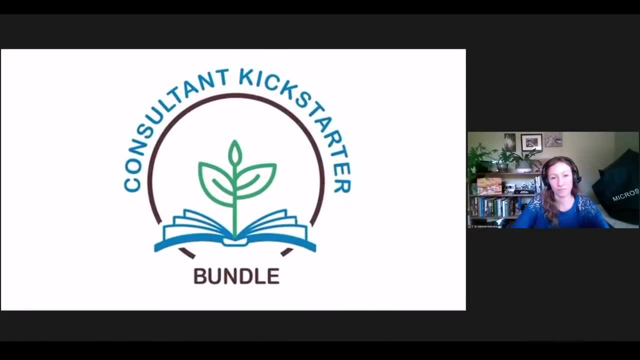 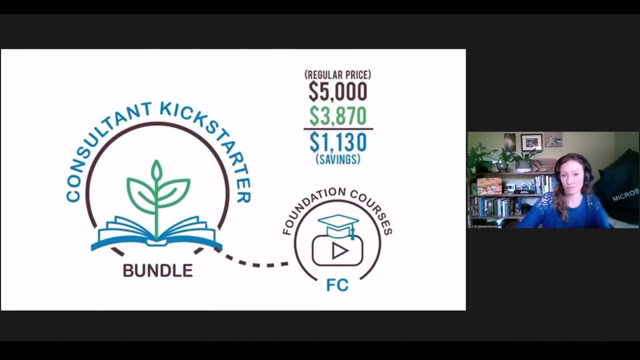 This month we're presenting our biggest bundle with the biggest savings. With the consultant Kickstarter bundle, you can register for the soil food web foundation courses with Dr Elaine Ingham for just 3870, saving over $1,100 through October 21.. You'll also get stage one of the consultant. 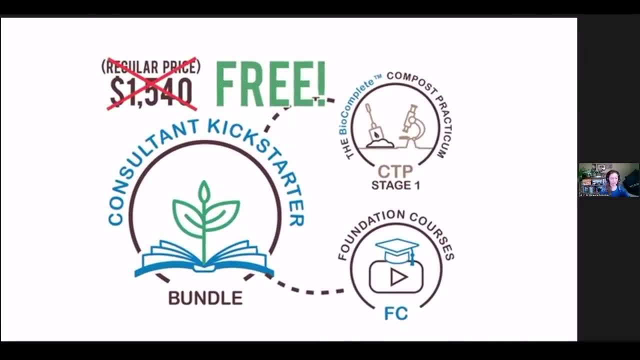 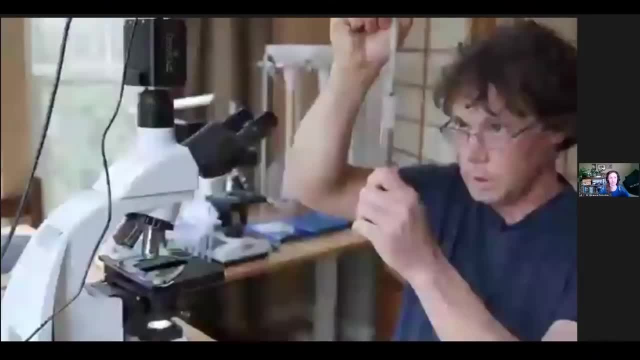 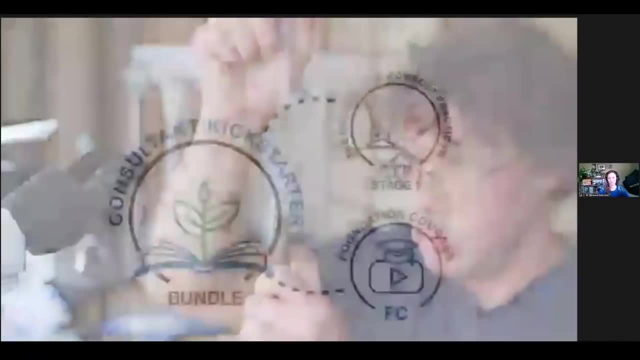 training program totally free, saving a further 1540.. That's 26 hours of mentor time dedicated to helping you make your own biological compost and develop your microscopy skills to the standard required to qualify as a certified soil food web lab technician. You'll also get two free bonuses with this offer: the 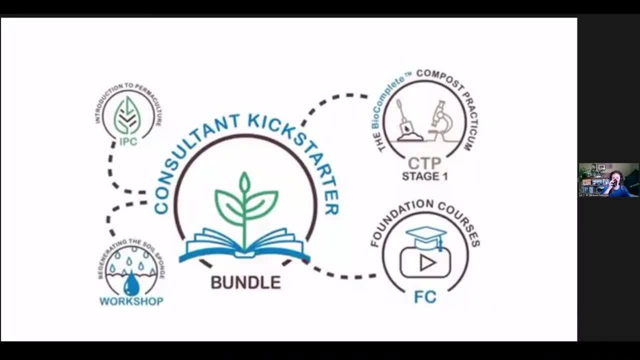 introduction to permaculture course by Graham Bell and the all new soil sponge regeneration workshop with DD Pursehouse, saving a further $500.. This is the biggest discount bundle we've offered, with a total value of over $7,000, for which you'll. 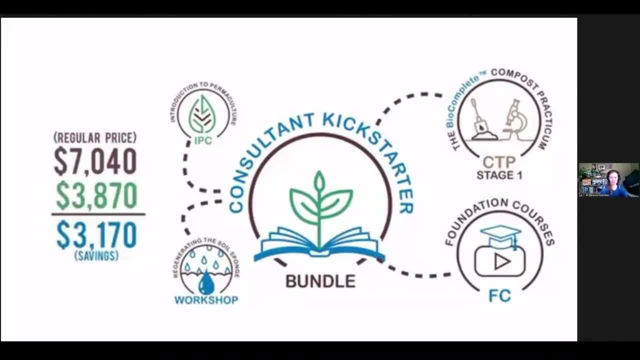 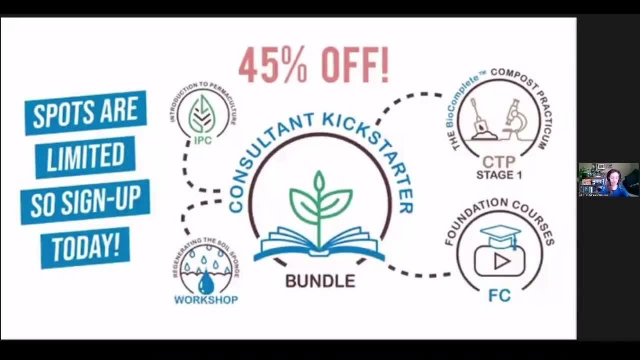 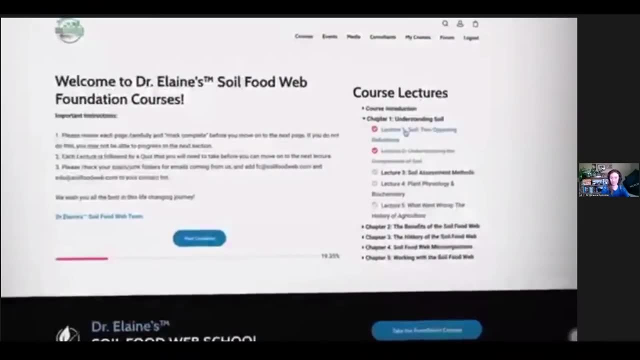 only pay 3870, saving you over $31,000.. That's 45% off. There are limited places available with the consultant Kickstarter bundle, so please don't delay. In foundation course one, you'll take a deep dive into the science and methodology that underpins the soil food web. 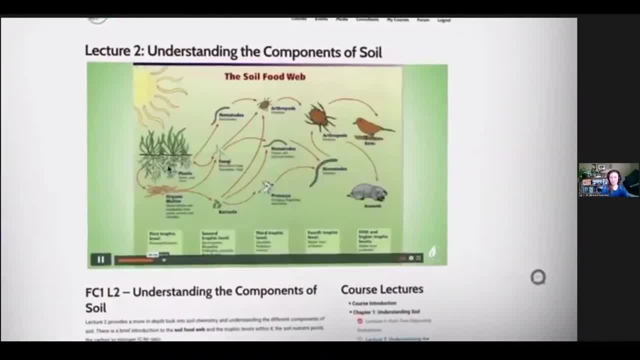 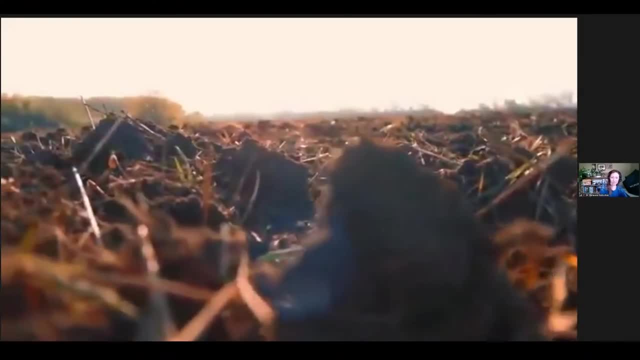 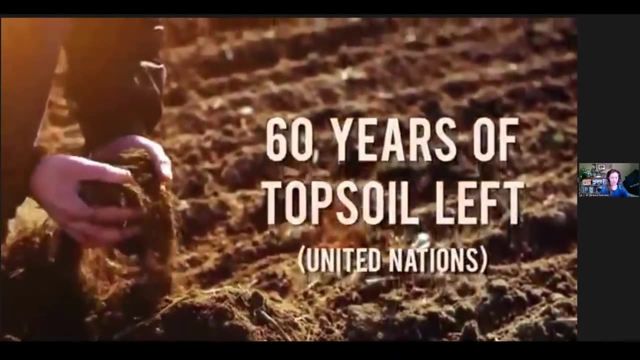 approach which was developed by Dr Elaine Ingham. over the last four decades, You'll study the history of soil on planet Earth and how the agricultural practices we've been using in the last hundred years have degraded our soils to the point where we now only have around 60 harvests left, according to the. 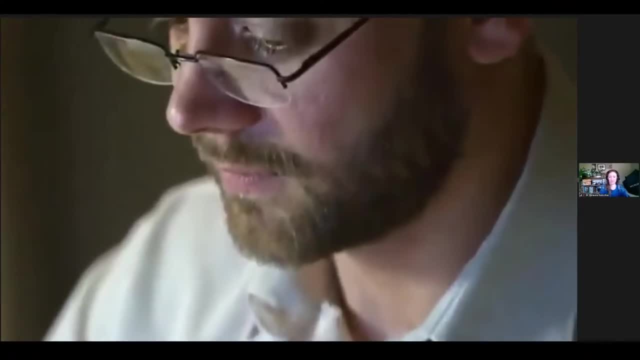 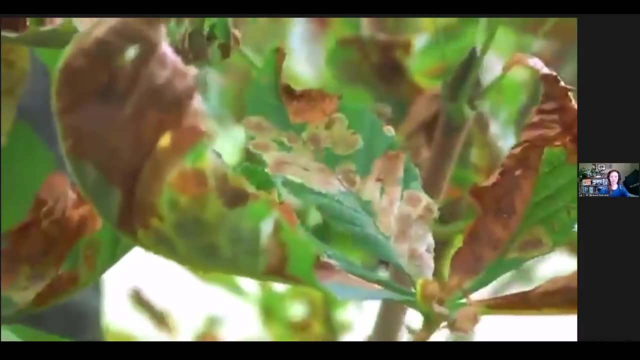 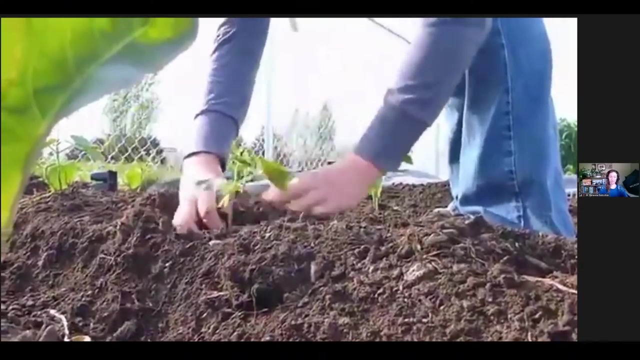 United Nations, You'll learn about the solution to many of the problems that are familiar to farmers all over the world today, Problems like diminishing soil fertility, pest and disease pressure, low crop yields, drought, flooding, compaction and soil erosion. Regenerative agriculture can address all of 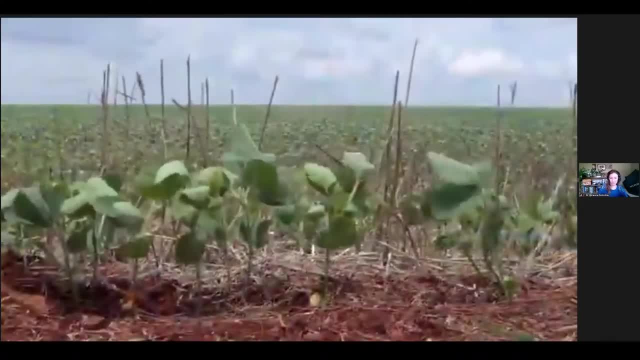 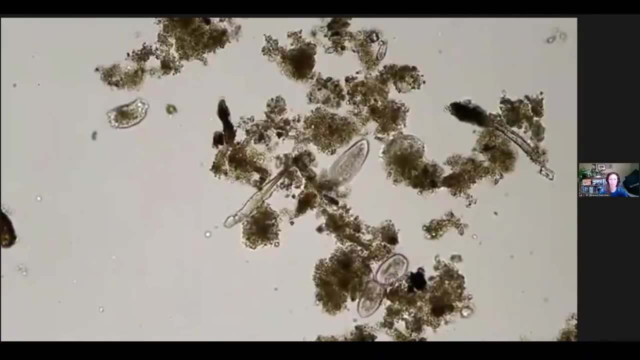 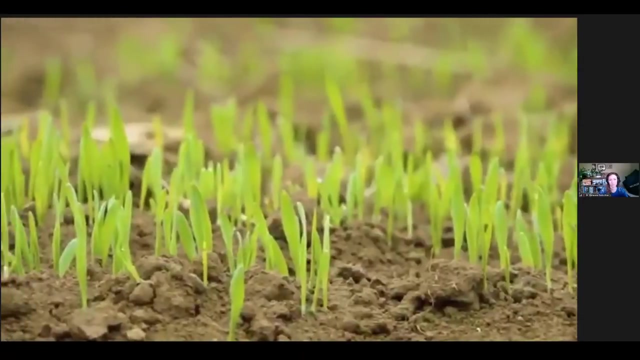 these problems. You'll be introduced to regenerative practices like no till and the use of cover plants. You'll also learn about the four major groups of microorganisms that drive soil regeneration and how the process can be accelerated by restoring the microbial community, or soil food web, to 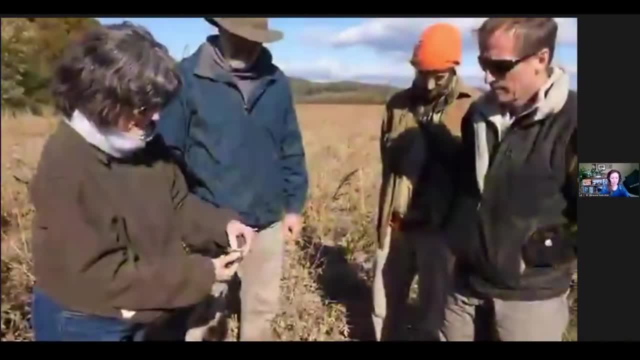 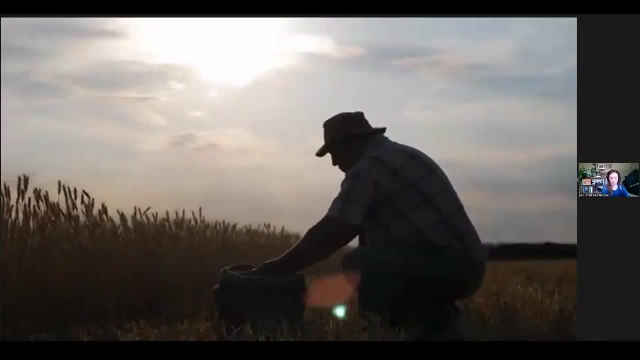 your client soils. Dr Elaine will present a number of case studies from around the world that she has worked on personally. Here you'll see some of the amazing results that have been achieved using the soil food web approach. In foundation course two you will learn all about the importance. 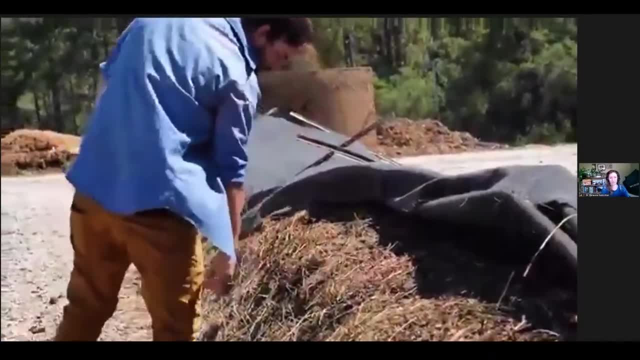 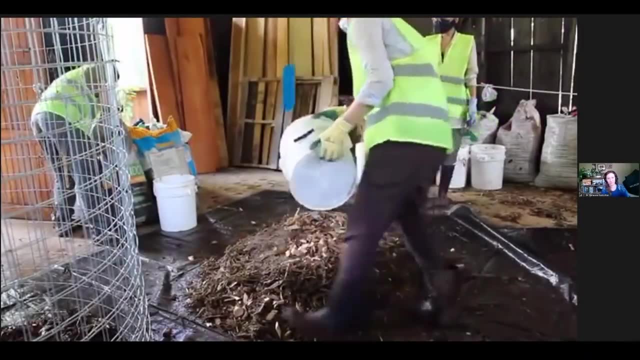 of biological compost and how it's very different from the regular compost. When most people look at compost, they only see a means of delivering nutrients to their plants, So they think about how much nitrogen, potassium, phosphorus and other elements are in the compost When we look at 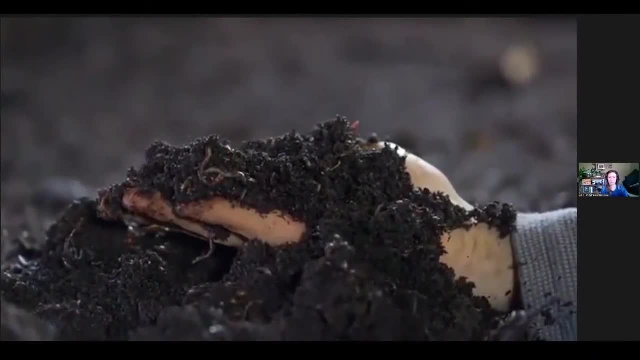 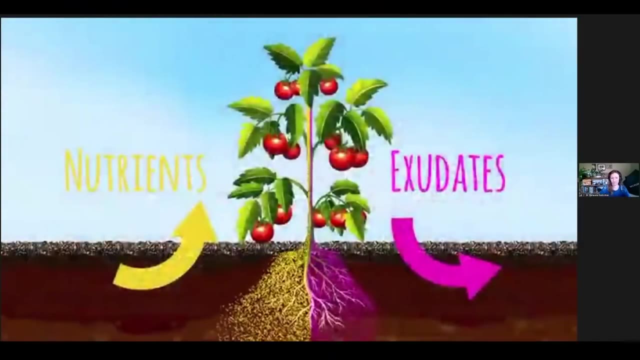 biological compost we see a means of inoculating the soil with beneficial microorganisms so that the soil ecosystem can start to function again, providing plants with a continual supply of nutrients. This is kind of like teaching someone to fish so they can feed themselves for life. 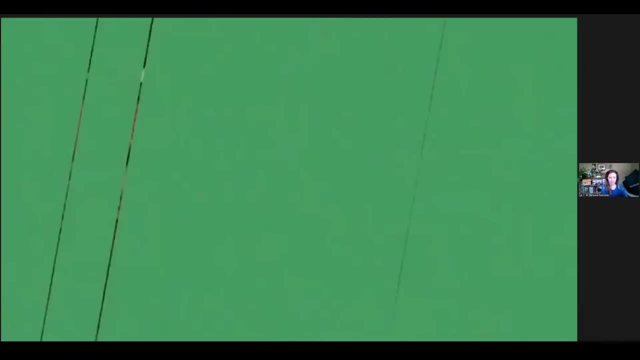 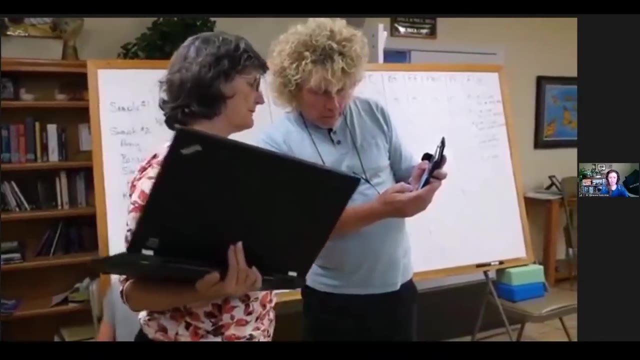 As opposed to just giving them a single meal. In this part of the training, you will learn how to make biological compost using various starting materials to create a recipe that will produce results. You'll learn how to monitor and control moisture levels, aeration and temperature in. 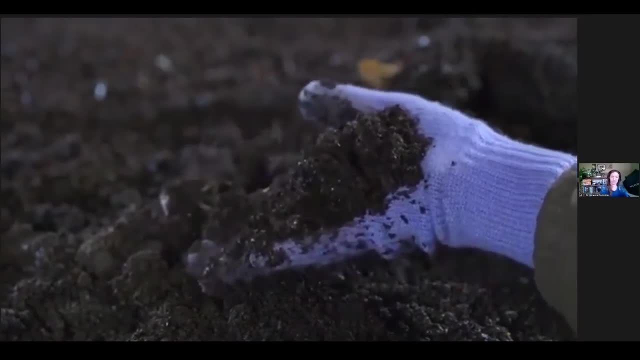 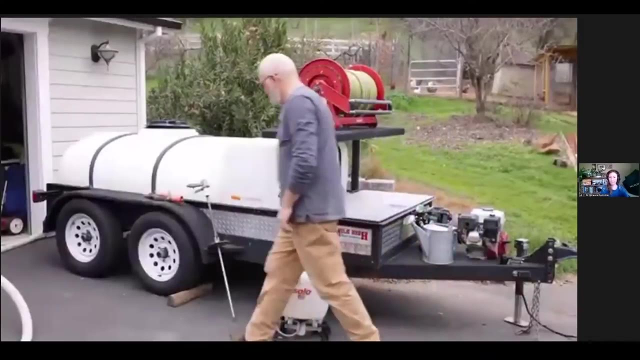 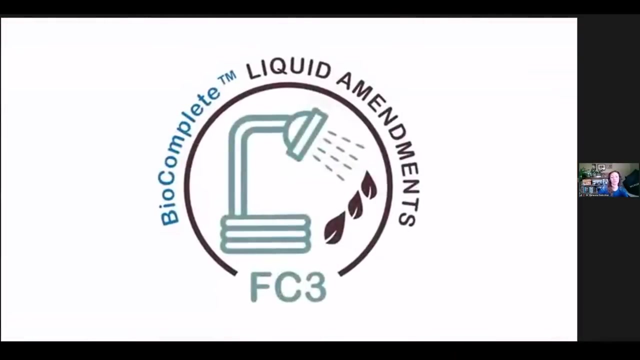 order to ensure that beneficial microorganisms are multiplied while disease-causing organisms are destroyed or become dormant. You'll also learn about the various types of equipment that can be used at different scales, and you'll learn about the different ways in which biological compost can be applied to the soil. In Foundation Course 3,, you'll 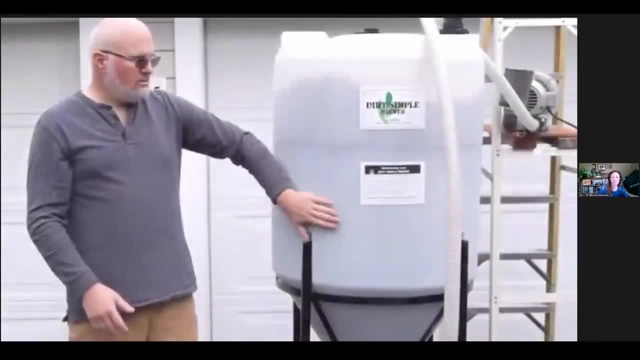 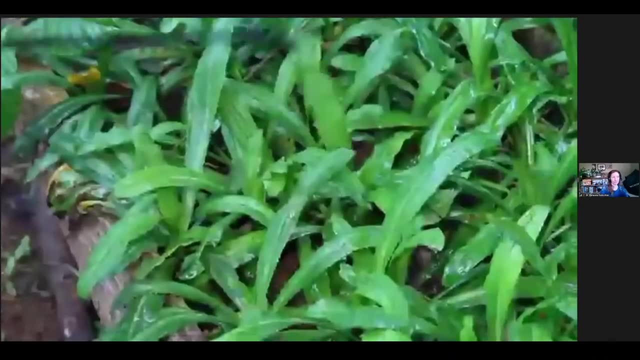 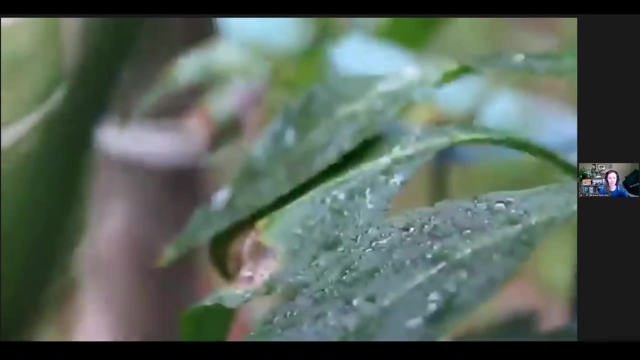 study Dr Elaine's methods for making liquid biological soil amendments. Compost extracts are used as a soil drench, delivering microbes deep into the soil profile where they can interact with the plant's root system. Compost teas are applied to the plant's foliage where they form a protective. 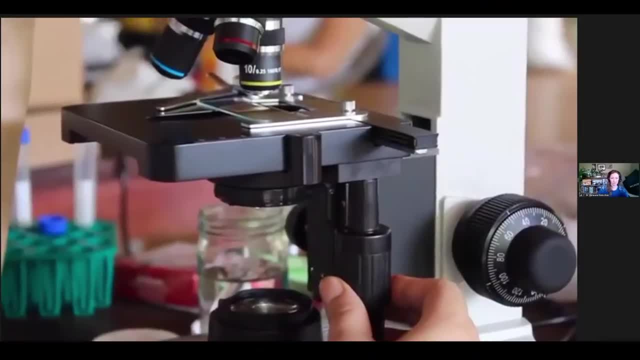 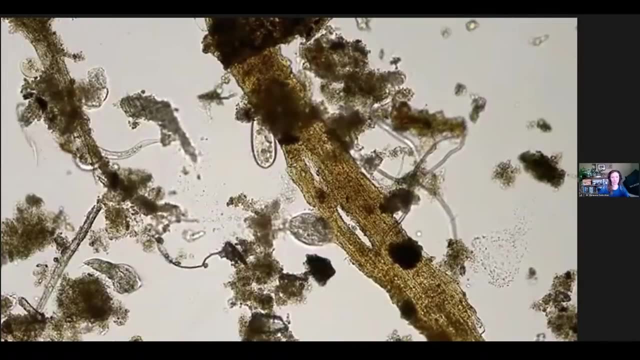 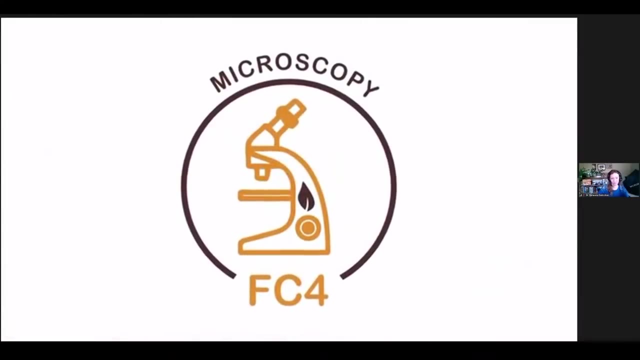 barrier against foliar diseases. In time, as your soil biome becomes more diverse and vigorous, your plants and trees may be entirely covered with beneficial microbes without having to continually apply them. In Foundation Course 4, you'll focus on four major groups of microorganisms in the soil: food, web, Bacteria, fungi. 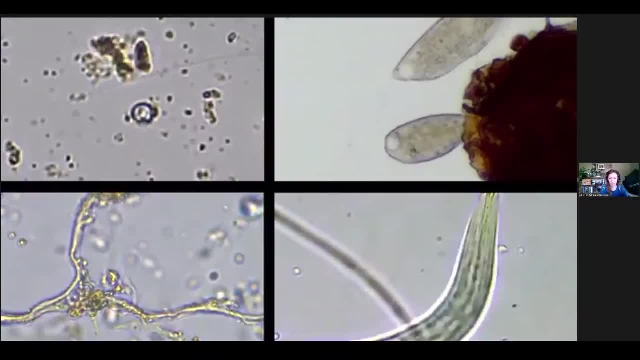 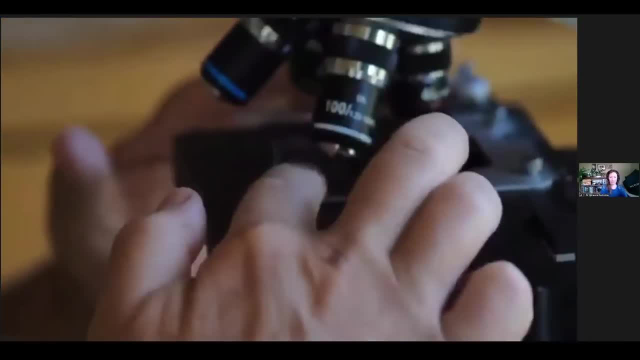 protozoa and nematodes. You'll learn how to use a compound microscope to identify and quantify these microbes so that you can really see what's going on in your compost and in the soil. This will give you the ability to assess the quality. 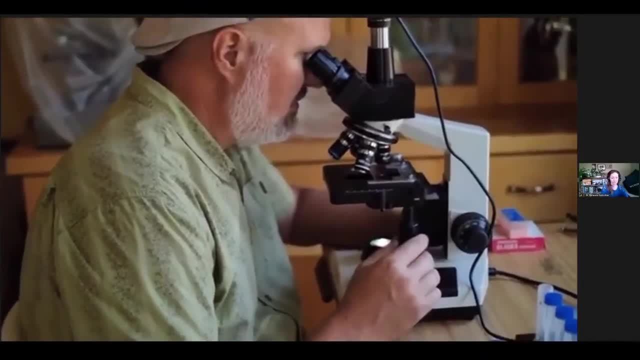 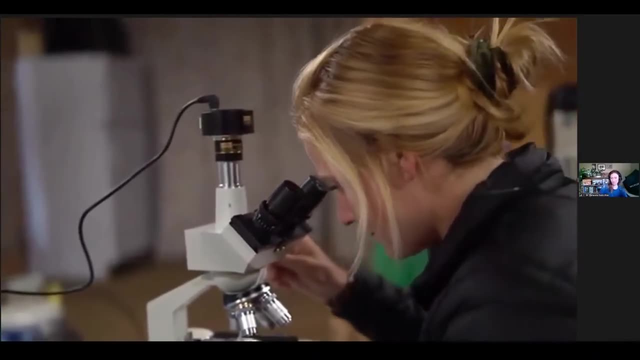 of your compost and liquid amendments before you invest all the time and effort that is required to apply them to the soil. You will also be able to monitor the progress of the microbial community in your soil over time, So if something is going wrong, you will know about it before the plants. 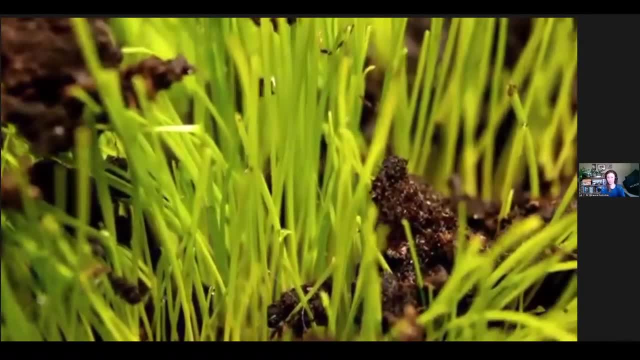 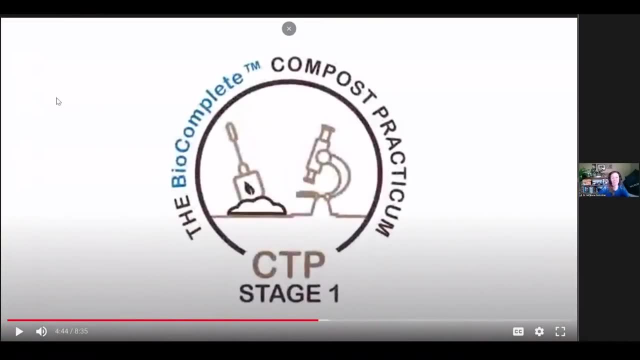 start to suffer. This gives you the opportunity to take remedial action early on in the growing season. Okay, it's always great to get to see the composting process so that y'all can really be in it as we start to talk about it. 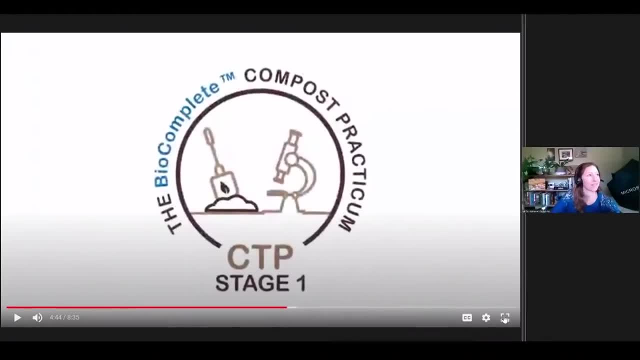 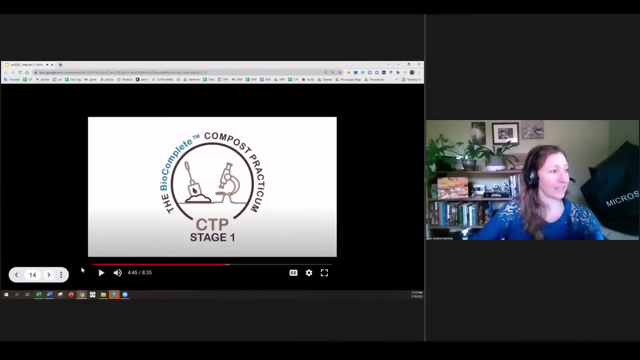 with Dr Elaine, So I'm going to try to escape my video What's going on And that's why I had to switch to the slides on my slide earlier, Just so you know once again each one of the consultation. 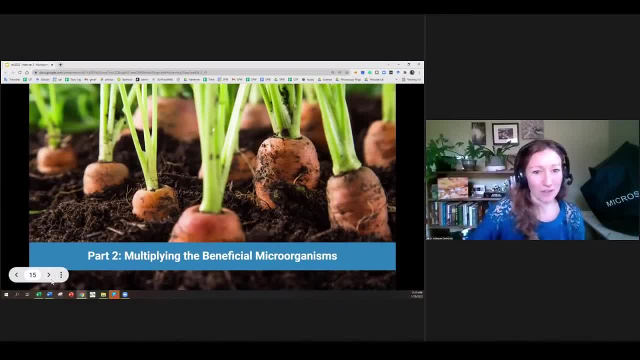 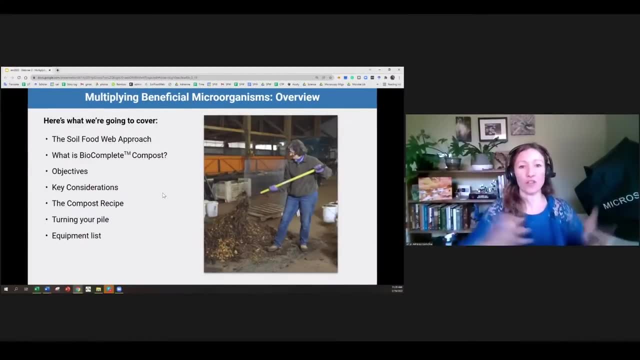 But bear with me. and then we get to hear part two, multiplying the beneficial microorganisms. All right, so the overview of what we're going to talk about today. it's going to be our general philosophies and approach. What even is what we call biocomplete compost? How is that different? 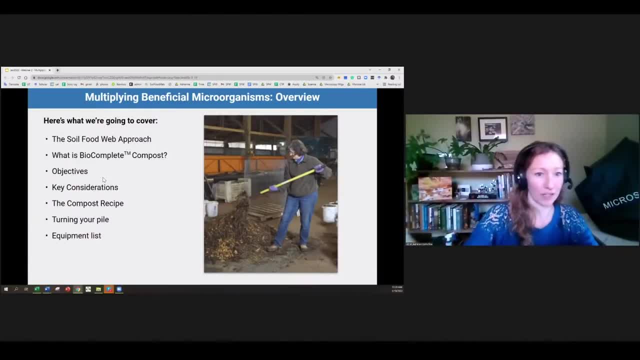 from other forms of compost. How is that different from rotting organic Lei matter or banana peels on your countertop? Um, what are our objectives when it comes to making compost? some key considerations and a good way to make the compost recipe so that you are set up. 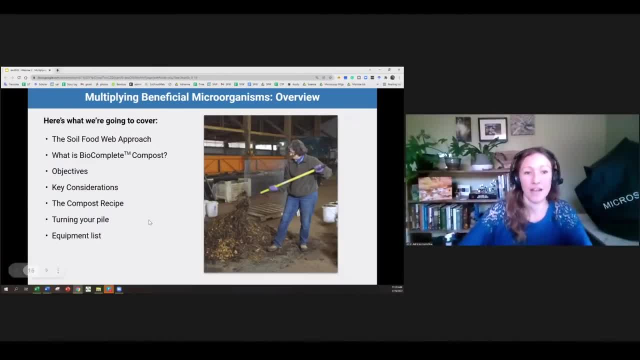 to succeed in any size or scale um, and how to adapt that to your region and then how to turn the pile. So we're really going to go over every aspect of composting um, because it's one of the best things that we can do, that any of us can do, in order to really make our soils healthy again. 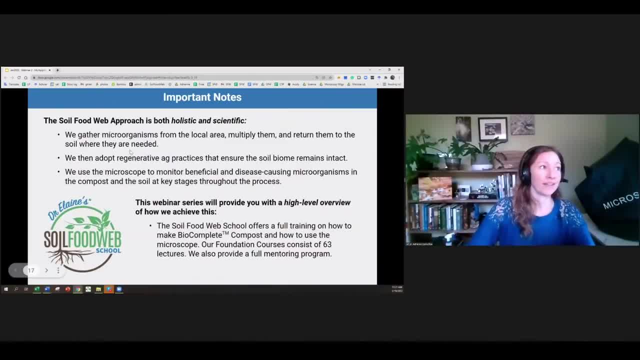 Uh. so a few important notes is that the soil food web approach is both holistic and scientific. We take a big picture view, but we are also basing everything that we do based on scientific studies and the data that Dr Lane Ingham has collected over four decades Um. 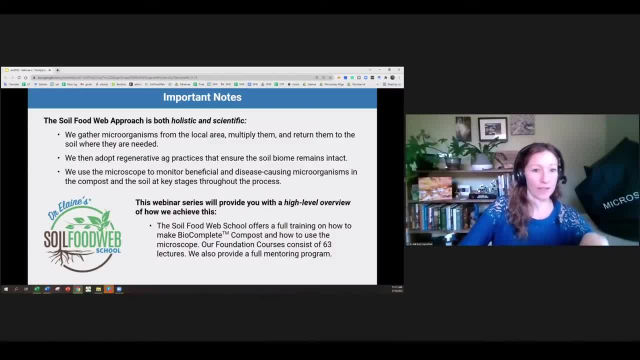 and because of that, and because of her connections with both farmers and scientists, she's been able to put together a method that really works. We gather the microorganisms from the local area in the starting materials, um, and we return them to the soil, which we'll learn about in the next webinar. We then adopt regenerative agriculture. 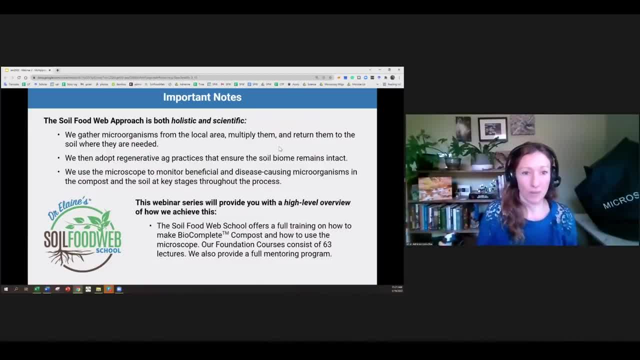 practices that ensure that that soil biome remains intact. So once you get the microbes there, you have to take care of them, which I think we'll talk more about in the next one, the next webinar. Um, we use a microscope in order to monitor and track, So it's we have quantitative methods to 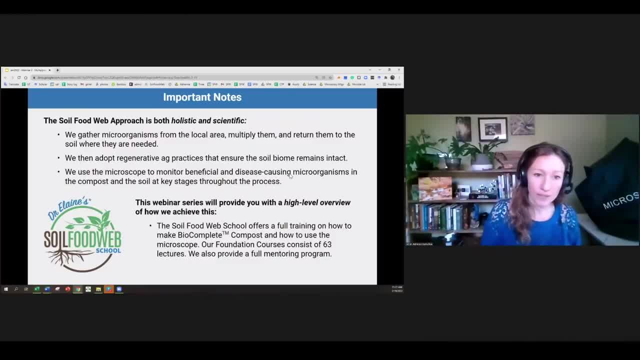 be able to see the progress of a healthy compost as well as how that compost, applied to soil, can increase the soil biology. Um. so we using a microscope is a really key, important part of our process to see which indicator species. So if you didn't get to see those in the last webinar, 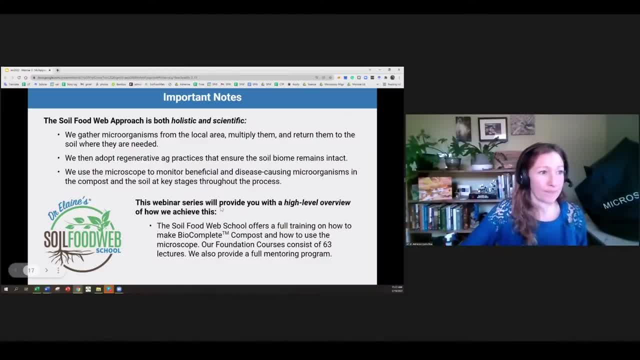 I recommend going back to see that replay. Um, yeah, so, and overall, the goal for us today is to give you a high level overview of all of the things that we tend to think about when it comes to compost. So there might be a few details here and there that we don't go into fully, but it 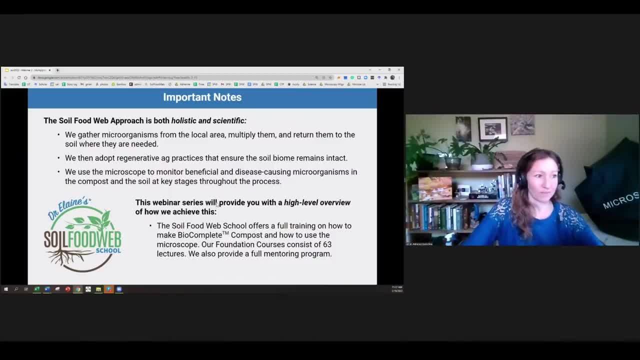 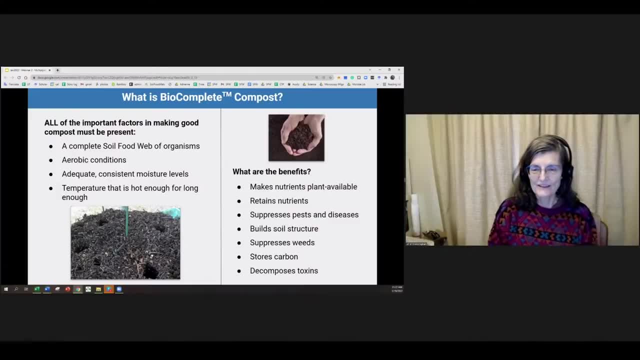 should give you a good picture of how to make compost generally. So with that I will pass it over to Dr Elaine Engen. Okay, Thank you very much. uh, Adrienne, Um, get going on. what is biocomplete compost? 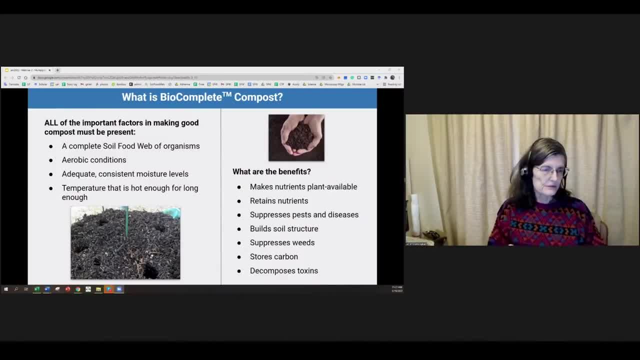 So, when we think about all the important factors, uh, to make good compost, we've got to have a complete soil food web of organisms. So exactly what is that number that we have seen as we're working on lots of different soils, lots of different uh bio uh regions? 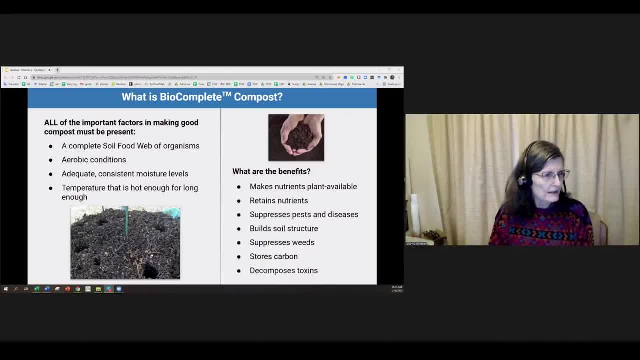 lots of different crops. Um, what we find is the minimum level of the soil food web really needs to be a very high level of biocompost. Um, so that's that's the number that we need to look for, which is the the that goes down the way that we need it to be at about, uh, um, 135. 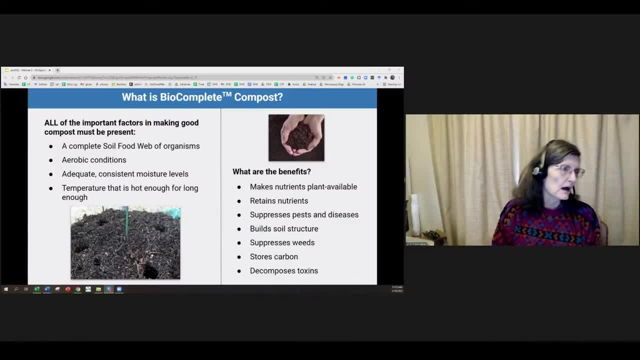 micrograms of fungi, 135 micrograms of bacteria, We've got to have 10,000, uh protozoa and somewhere uh around a hundred um beneficial nematodes. So understanding why we've said it there is because if you're going to be applying this biology into your soil, you've got to have at 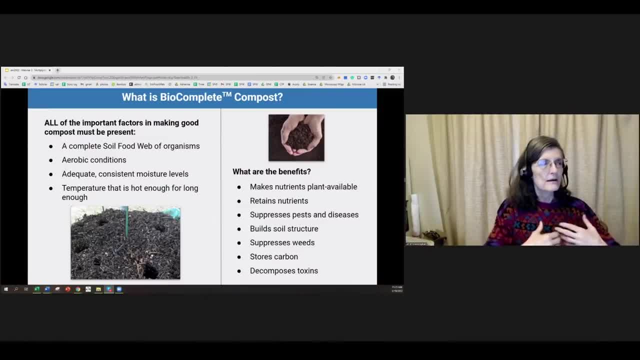 least this number of microbes. So that that's that's a critical element- I think that's a really microorganisms- for there to be a possibility of making a change in that dirt and converting it into soil. We also know that we have to have aerobic conditions. The beneficial organisms are 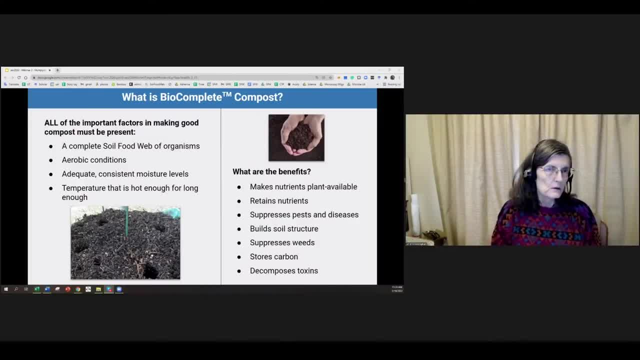 for the most part, aerobic organisms. When you think about roots of plants, they are obligately aerobic. As soon as you get into anaerobic conditions, your roots are going to die back. They're going to be attacked by diseases and pests. You've got inability to access nutrients. 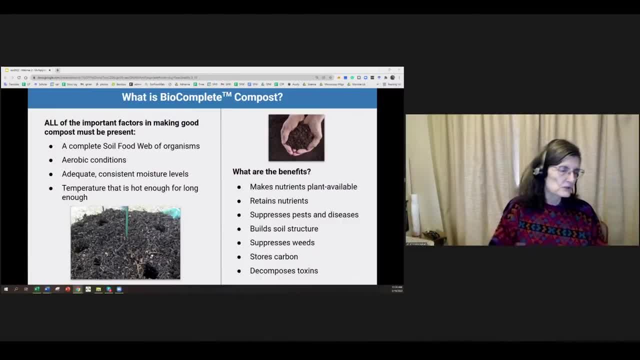 or water in that compacted soil and that soil that's anaerobic doesn't have enough oxygen in it. We know that we need to have adequate, consistent moisture levels when we're making compost. We want to not have too. We don't want to have too much water, We don't want to have too little water. This is a Goldilocks. principle. In general, the organisms should have somewhere between 40 to 50% moisture in the soil. There's enough free water for those microorganisms to be able to grow. It's the growth that composting is all about, because we've got to get the temperature up hot enough, long enough to take. 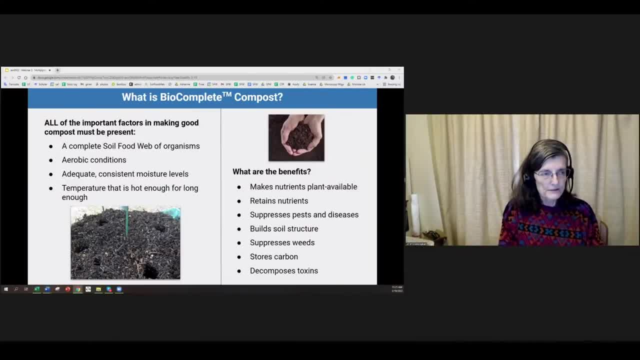 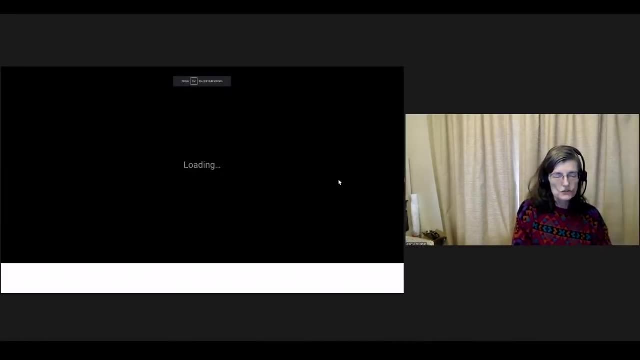 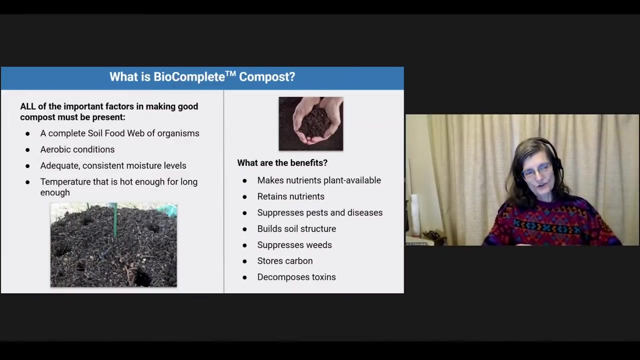 care of the disease causing organisms, The pests, the problem organisms need to make certain that those are not going to be left in your compost. We've got to get the temperature hot enough, long enough. The way you do that is to. The way you do that is to make sure that the microorganisms are growing in that compost pile. 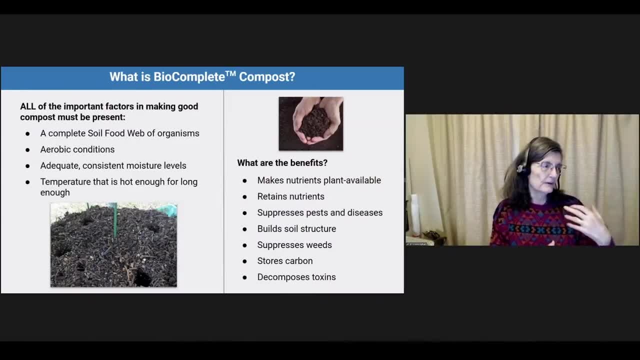 We have to have enough high nitrogen. we have to have enough green material, enough woody, so that we can get all of the different kinds of organisms growing in that compost pile. They've got to be growing rapidly enough to make the temperature to kill the diseases and pests and problem organisms. 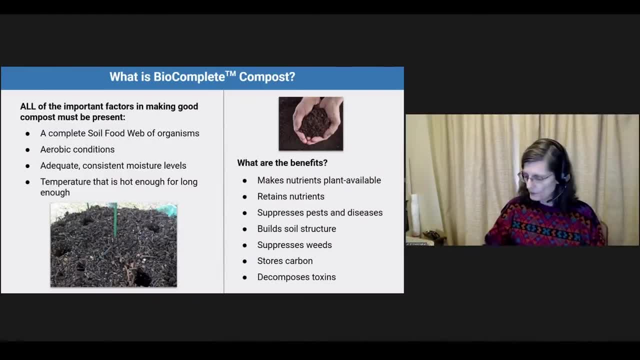 When we manage all of that, and I like to point in this picture to a particular factor that we've been working with. when you look at these- I'm going to have to go back up here to view components- get my, let's see if that there we go, You can see these, basically holes that we've punched. 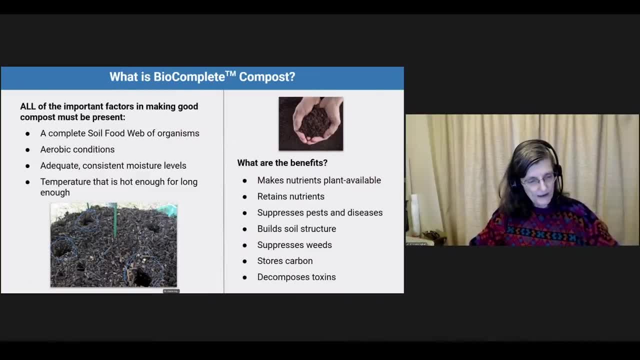 into the depths of that compost pile. So this was a compost pile that was getting too hot too fast. You're starting to approach the 175 degrees Fahrenheit threshold where we're going to be going to anaerobic and just starting to grow. any of the disease causing spores perhaps might. 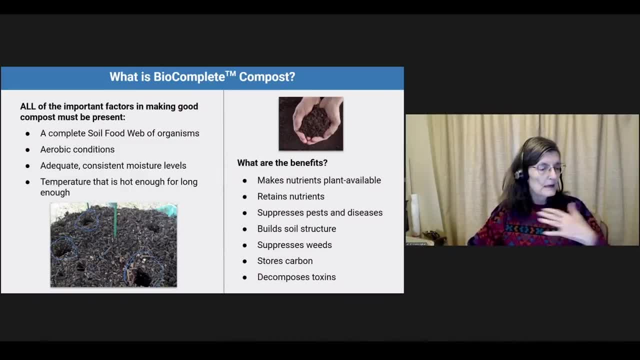 wake up and start to grow. So we want it to remain aerobic to prevent those not beneficial organisms from starting to grow. So we're going to punch, basically, a PVC pipe, punch that down through the compost So you leave open this chimney, so that oxygen 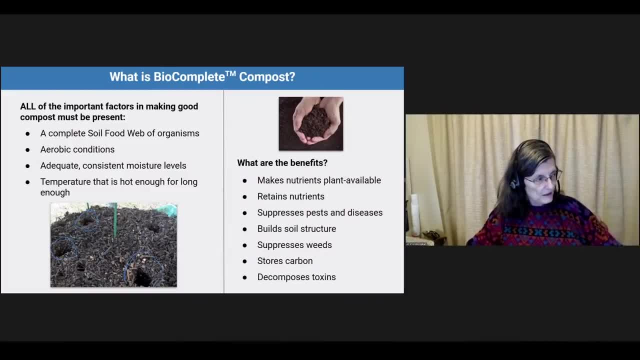 from the atmosphere can move down into that hole. Hot air rises, of course. So the hot air is going to be piped off while the cooler air get down into that pile. So we're going to maintain the temperature. We're going to maintain the aerobic conditions as well. So 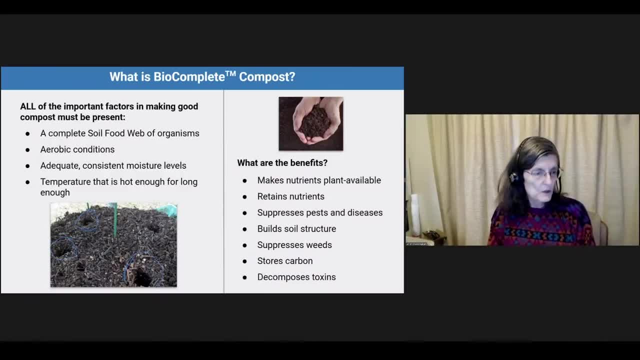 it might have to be recipes for angry井 в. Can you see, because we rub our hand, maybe this one down to here so everybody can see? Absolutely, You got to do that. well, I see it's working, Tim. I saw that it's working and that's great. 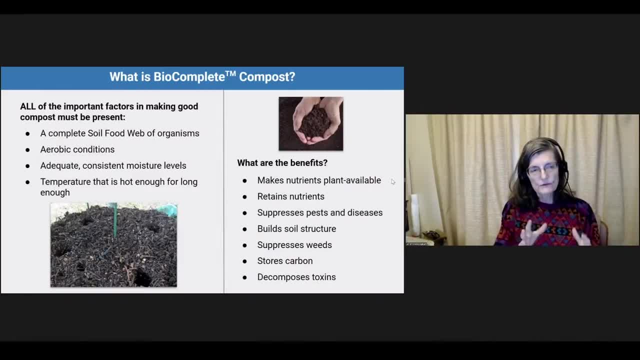 Okay that we talk about in the first foundation course, about making certain that the foods for the bacteria and fungi are plentiful So they can be producing the enzymes. that pulls those nutrients out of the silica bilayer of the sand, silt and clay. 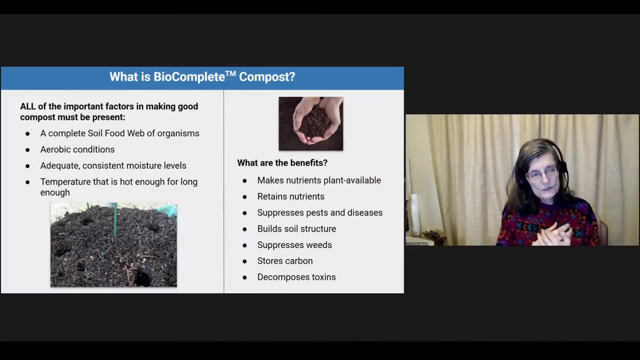 also out of the organic matter. So for as long as you have sand, silt and clay in your soil, you shouldn't have to put on inorganic fertilizers if you've got the biology that will do this nutrient cycling Well, of course, the first step is to have enough food. 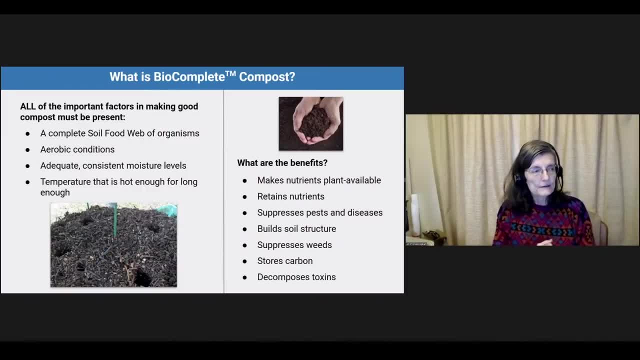 So we want roots or really good organic matter in the compost pile to allow these microorganisms to grow, to make the enzymes, to pull the nutrients from plant unavailable sources and tie them up in the bacteria and fungal biomass. Then when we put that composting, 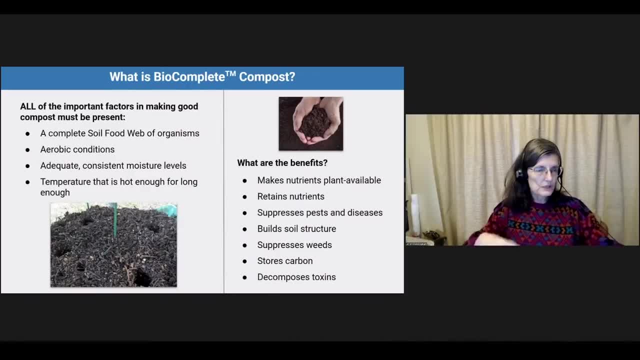 compost out on the ground, protozoa and nematodes will start to grow nicely. They will eat their predator, their prey, And that releases the excess of the mineral nutrients that were in an organic form inside those bacteria and fungi, And so those nutrients are released. 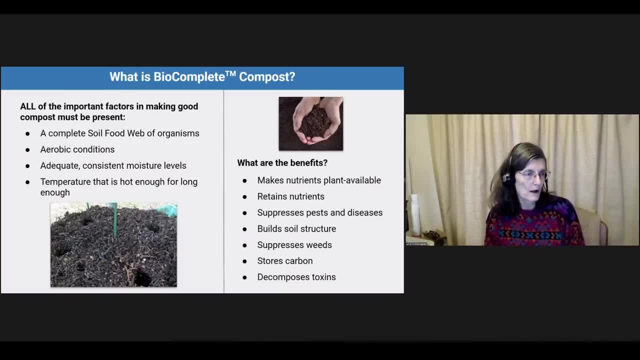 right in the root zone of your plant that you want to have growing. And so no, there is no soil. There is no soil that lacks the nutrients to grow plants if you've got the biology in that soil- the bacteria, the fungi, the protozoa, the nematodes. 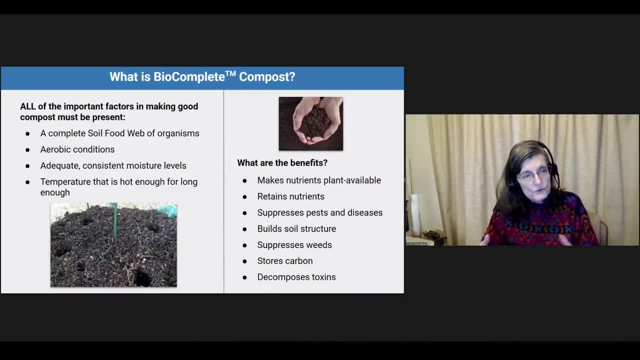 they must be present to get to those sources of plant not available nutrients and make them available to your plants. Now there are two other methods for getting nutrients into the plant: mycorrhizal fungi and the process of rhizophagia. I just don't have time to talk about it. 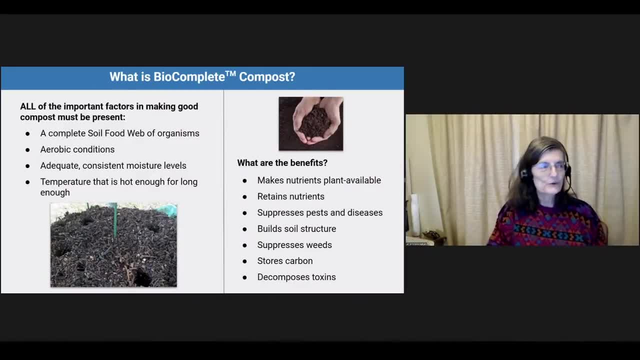 So you really need to get signed up for the courses. We need to retain nutrients in the soil, And of course it's the bacteria and fungi who do the majority of that kind of process. We want those microorganisms, growing very rapidly, get to the high levels that we require. 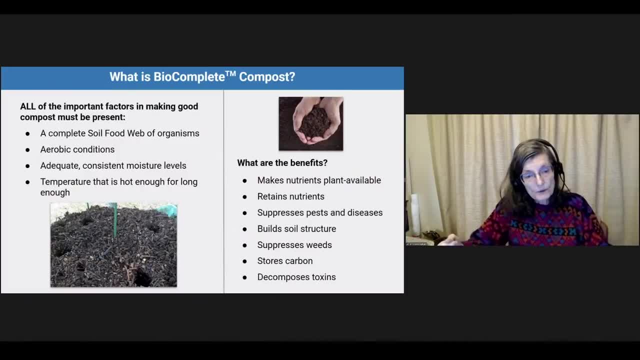 So all the nutrients will be retained. They won't be made available until the predators come after those prey species and you can get them back. So that's the first step, And then the second step is to get the nutrients and chow down on them. 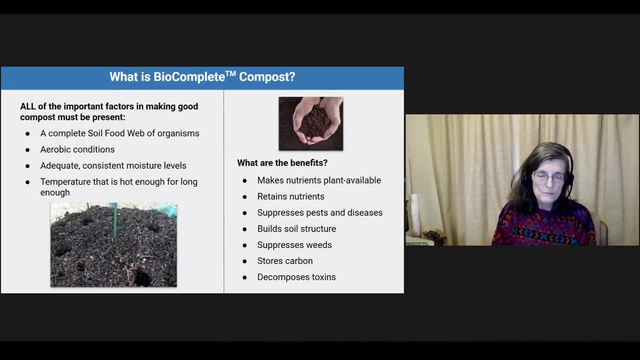 releasing those nutrients in a plant available form. But you won't have leaching losses, You won't be losing your soil through erosion. We're going to suppress diseases and pest organisms, because if a plant is getting all the nutrient it needs into its biomass, that means it's got the energy. 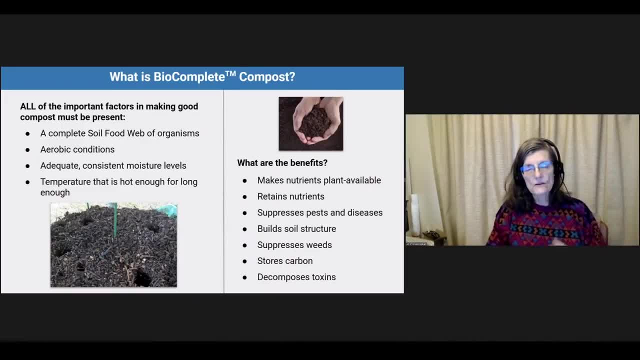 it has the nutrients to be able to make those compounds that prevent the diseases and pests from being able to attack and get into the internal components of your plant. So diseases and pests are no longer something you have to worry about. Those diseases, the pests, may come wandering. 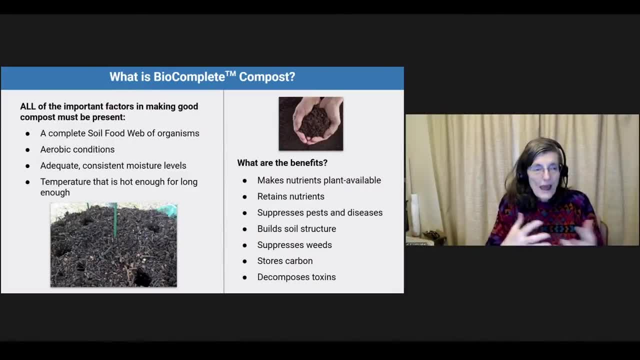 through your garden, but if there's no access to your plant material, they're just going to keep on going. We need to have the nutrients in the soil. We need to have the organisms that build structure. Of course that's bacteria at the smallest level. 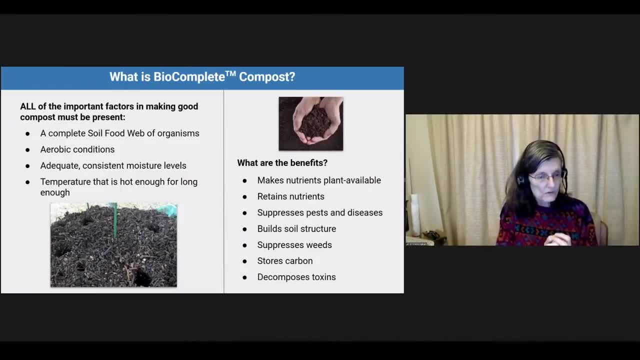 Bacteria and fungi have to make micro aggregates and start forming structures. So now oxygen and water can come down through that soil as the structure is being made, so that your root systems can grow deeper and deeper and access all of those nutrients, all of that stored water. 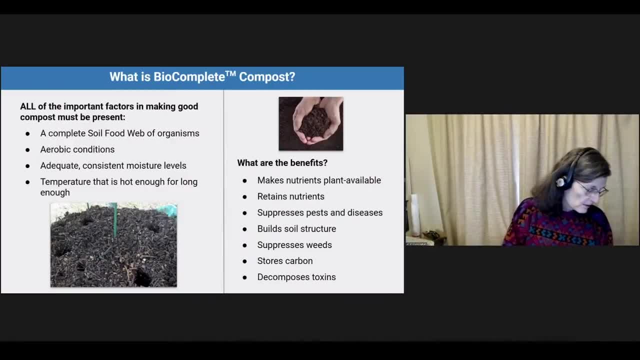 that are in the deeper depths of the soil. We've got to have the structure to store that water in the deeper layers of the soil throughout the whole soil. So we need to build that soil structure so roots can go as deep as they possibly can go. 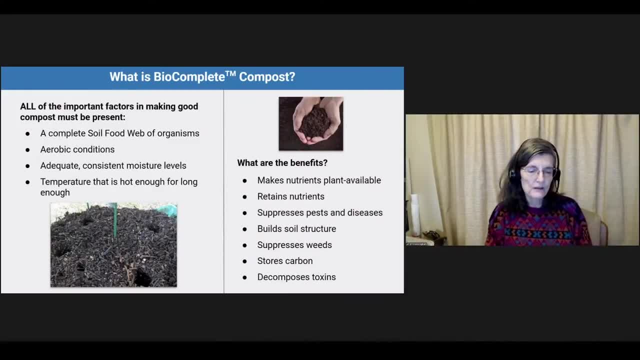 And roots don't go down just a couple of inches. I mean, we're always presented with this idea that here's the soil surface and as you move through that soil, roots only go down a couple of inches and then they go sideways. 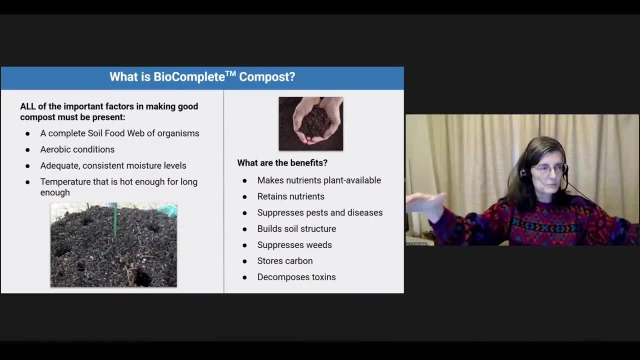 And then they fight and have wars with all the surrounding plant material, Because that's not how soil works. We have this bizarre, this strange attitude about how deep soil goes, Because if you have the structure built by the bacteria and then by the fungi coming along, 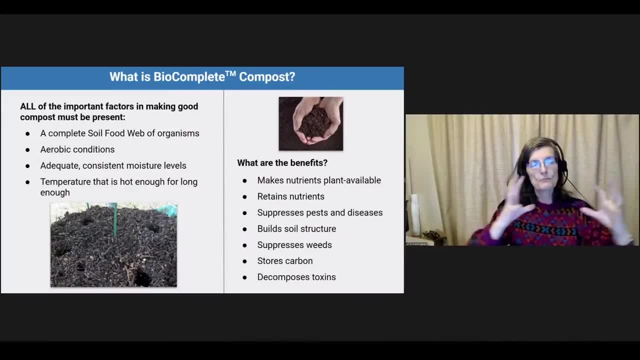 and binding the soil, binding those micro-aggregates together into macro-aggregates, providing even larger air passageways and hallways for oxygen and water and your roots to grow down deeper and deeper, for the water to be stored deeper in your soil. 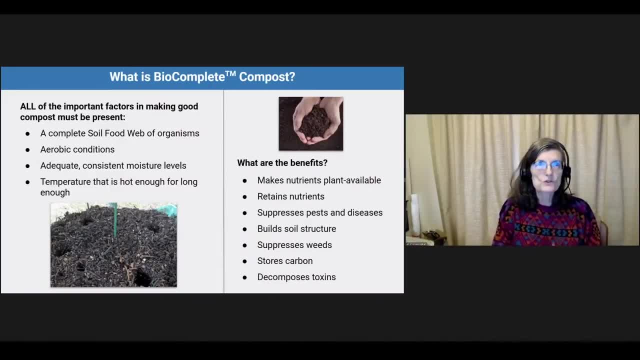 Then we have all the nutrients we need. There is no soil on this planet that lacks the nutrients to grow plants. There is no need for pesticides or herbicides If we get all of this biology back in the proper amounts for the different kinds of plants we're trying to grow. 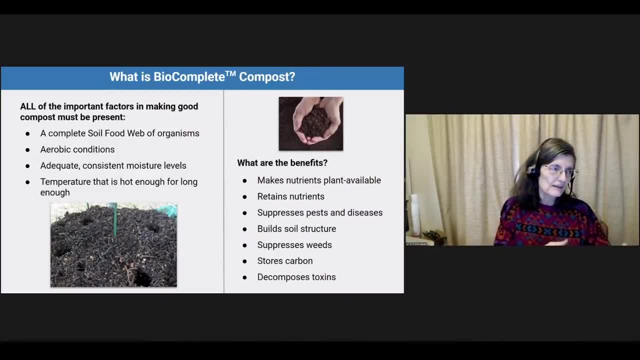 We're, of course, gonna suppress disease. If that soil is promoting the growth of the plants that we want, it means it's not promoting the growth of weeds. Weeds require, just about across the board, only nitrate. That's what weeds require. 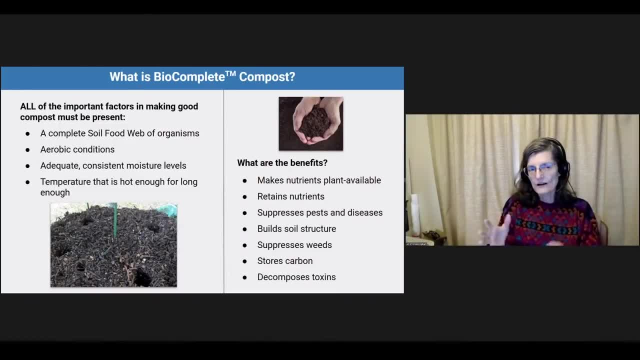 As soon as you move out of the strictly bacterial dominated soil conditions, as you start to get fungi making a greater and greater and greater contribution to that soil biology, to the soil nutrients. now the fungi are going to make certain that the nitrogen- the plant available soluble nitrogen- is now going to be in the form of NH4. Ammonium. ammonium- The emphasis on that last part of that word. The ammonium is used by our crop plants, and the more and more fungal the soil, the more and more we select for shrubs. 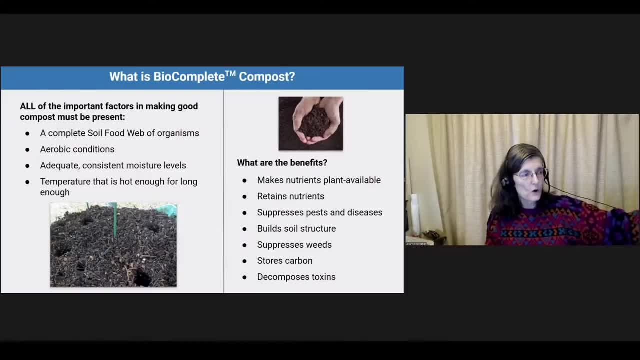 deciduous trees and then conifer trees and old growth forest. So we want to move away from that weedy stage of succession And the way you do that is by getting the proper balance within these soil organisms. Of course we have the fungi storing carbon. 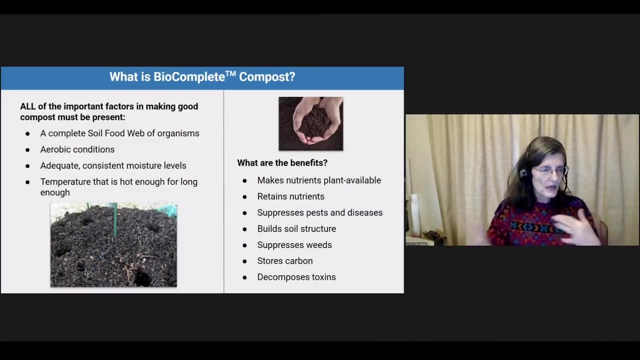 at a huge percentage. When fungi decompose plant material, 80% of that carbon that was in that plant material is going to be put down as an inner lining in the hyphae, Whereas bacteria, of course, don't Don't do that. 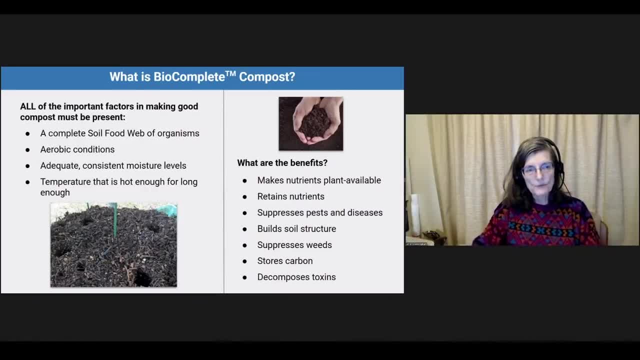 So 80% of the carbon that bacteria decompose blows off as CO2.. With fungi, only 20% of what that fungus is decomposing is being released as CO2.. So we have to understand that, because of course it makes a whole set of the microbiological measurement. 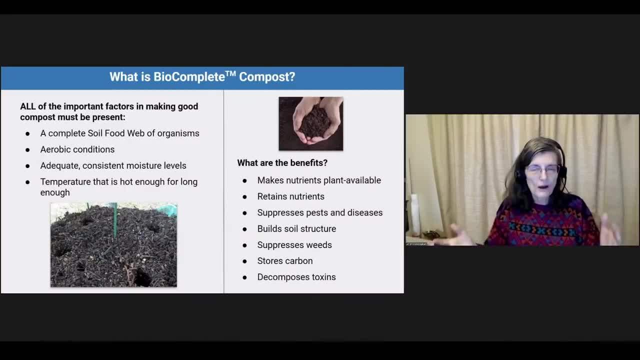 methods completely obsolete once you understand- So we have to understand that, because of course it makes a whole set of the microbiological measurement methods completely obsolete- once you understand How that division of CO2 per laying that material down as organic matter inside their bodies is so, so different. 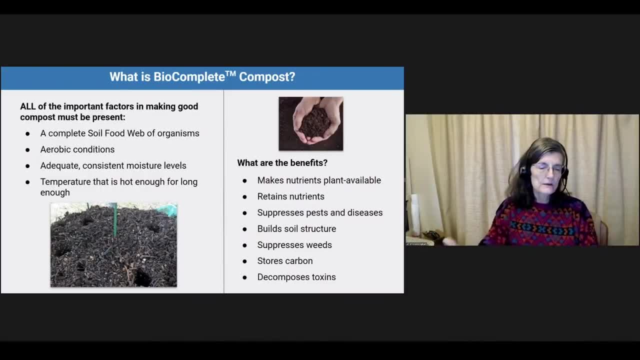 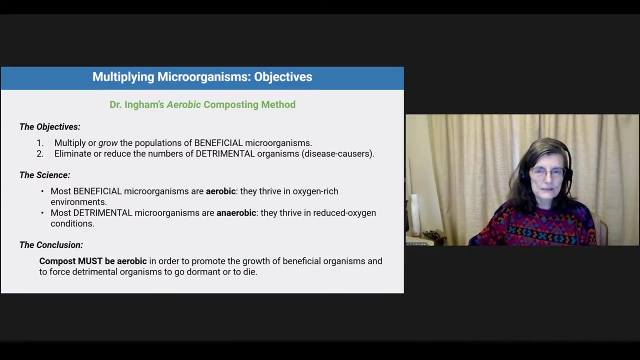 between bacteria and fungi, And then, of course, the decomposition of toxic materials, something that's done by many different microorganisms in that soil. So if I could have the next slide, So for doing aerobic composting, and it, you know, it doesn't. you know, we tend to look at the wire cages. 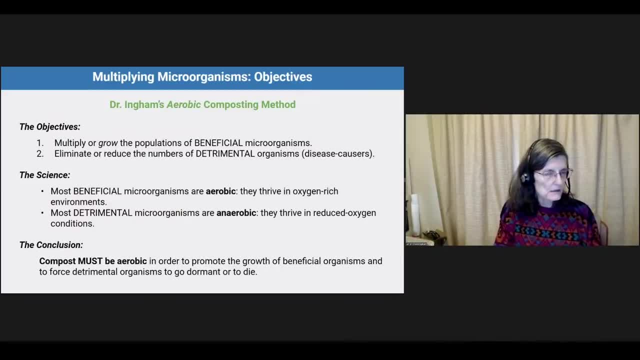 for small size composting processes. You can also have worm compost. You can have the Johnson Sue reactor. All of them follow these guidelines that we're talking about today, The important things in making compost. So the objective, of course, is to grow the beneficial organisms. 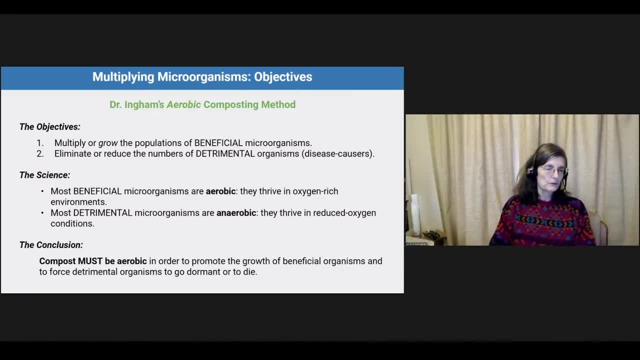 in your compost. You don't want any of the diseases and pests and problem organisms, So how do you eliminate or reduce those bad guys? So a number one: the most important thing is that the greatest number of beneficial microorganisms are produced under aerobic conditions. 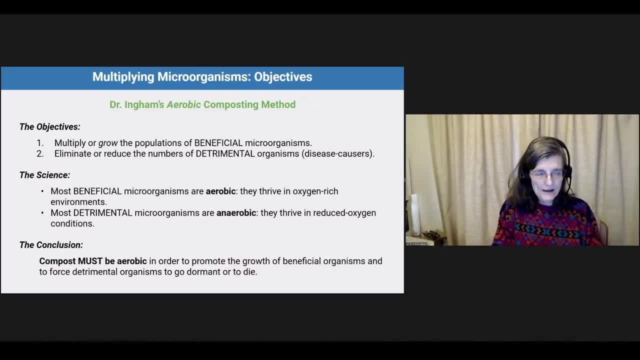 You have to have the enzymes, enzymes that require oxygen in order to perform functions, And that's what we need to have in our soil. So all these functions I just finished talking about are going to be performed. if we're dealing with aerobic organic material, The detrimental microorganisms require reduced 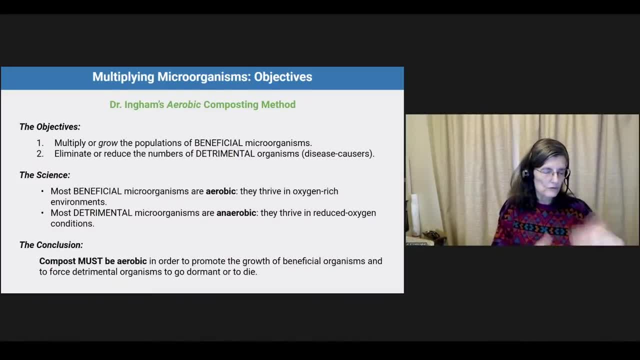 oxygen or reduced anaerobic conditions. They thrive in those reduced oxygen conditions. So compost has to be aerobic. Now, does it have to be aerobic absolutely every second of its life? Well, you know, you can have pockets of anaerobic conditions in the middle of the microaggregates. 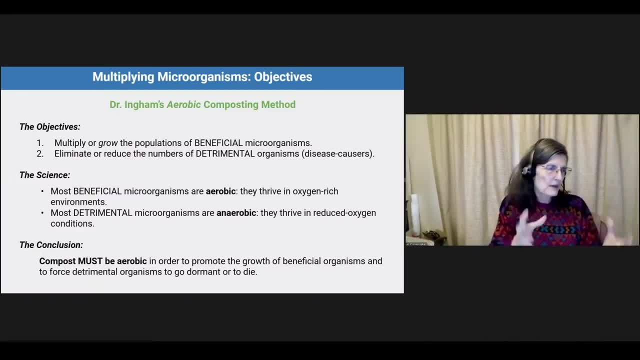 in the middle of the macroaggregates. You can have some anaerobic organisms in there, but the instant they step out of that protected area, you want them to be eaten. You want them to be attacked by the beneficial organisms. So the majority of the living conditions in soil or compost. 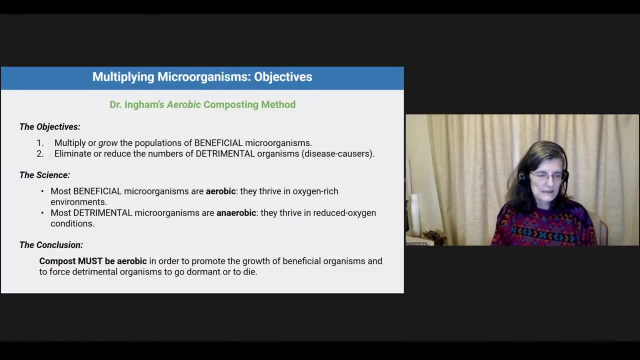 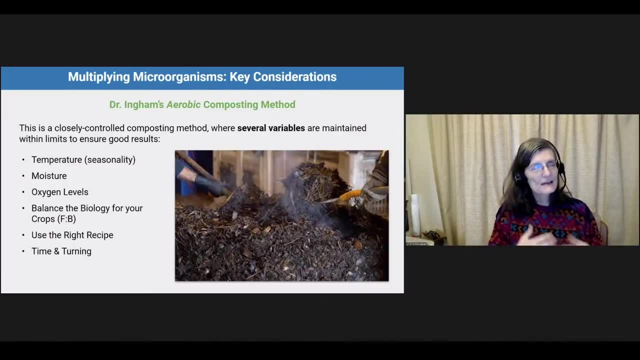 need to be aerobic. Next slide: We take a lot of care to understand what all of the important variables are in the soil. We've got to get the temperature such that we are going to get high enough temperature for a long enough period of time that the disease 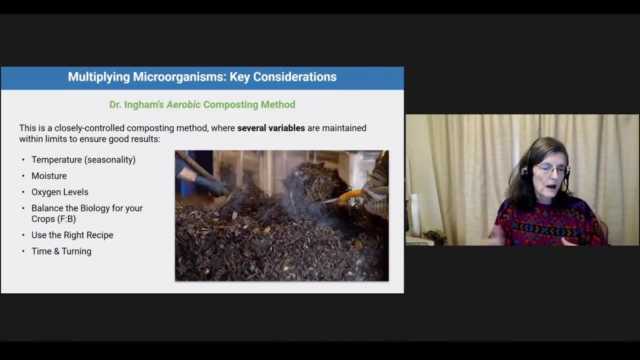 causing organisms. the things we don't want in that soil are taken care of. So we'll talk about those temperature. What are the temperature levels that you want To be attaining as you're going through this composting process? Seasonality is important. 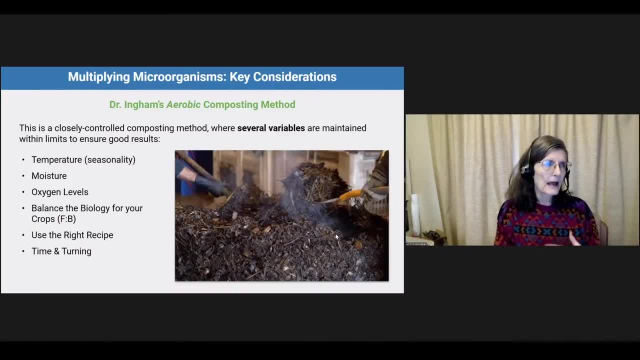 This affects the kinds of foods that you're going to be putting into your compost pile. to get the balance of the microorganisms that you want, The first step is getting temperature to occur in that pile, and that occurs because the microorganisms start growing very rapidly, as I talked about before. 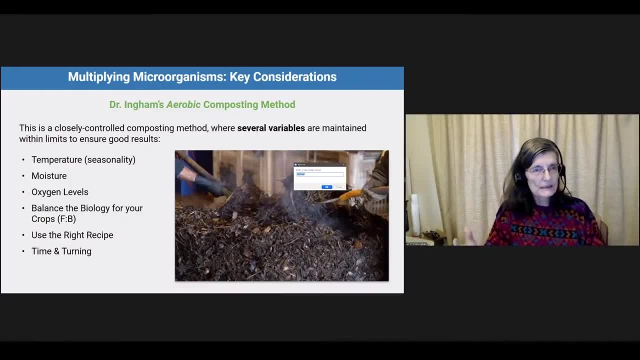 The faster they grow, the more heat is released. They're well, just like human beings. Think about you doing reproductive activities and how much temperature is raised by performing those activities. Same thing for the microorganisms. It's that heat of reproduction that we need to have happening in our compost piles. 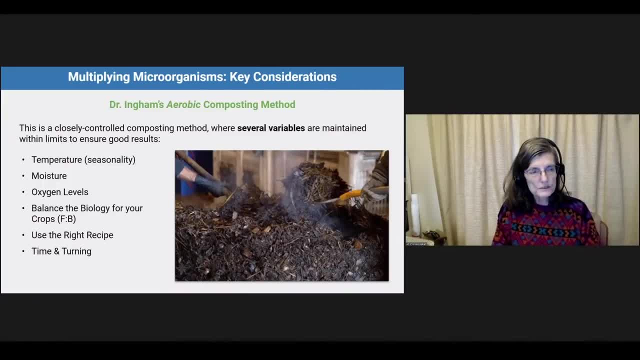 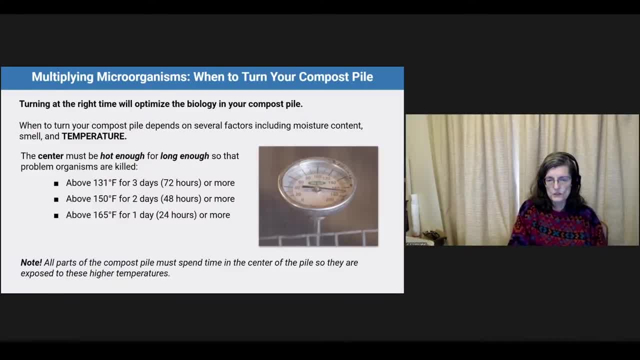 So the foods we put in there have to promote enough rapid growth for them to survive. So the foods we put in there have to promote enough rapid growth for them to survive right around. in that range you can buy a little like one and a half foot, one like 16 inch ones. for like 35 bucks if you're doing small composting in your backyard. yeah, so it also depends on the size of the pile that you're using. um small piles, you know you cannot retain heat in a pile that's smaller than, uh, one meter by one meter or three feet by three feet. that's the minimum size on any. 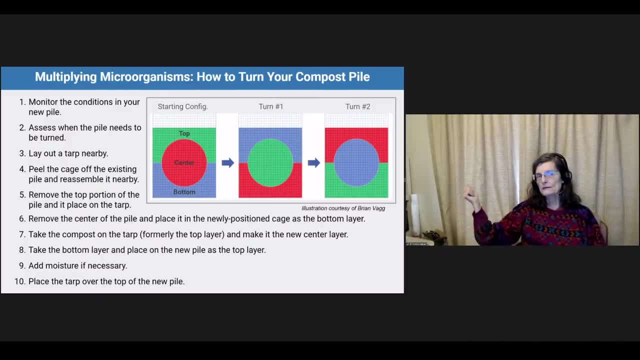 of these piles and i like to be able to get my thermometer all the way through the compost pile so i can look at where it's still cold, because this is expressing this slide, is expressing the turning process that we want to have people be cognizant of. so, if you think, brian, brian put: 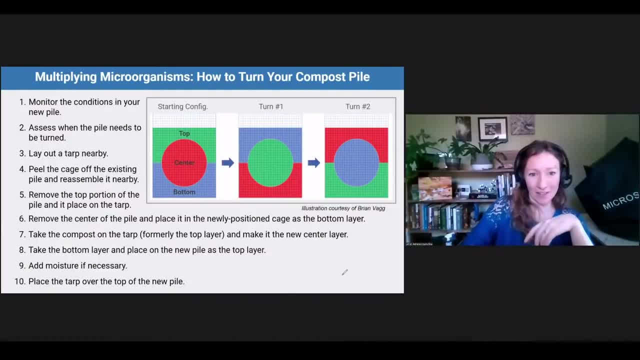 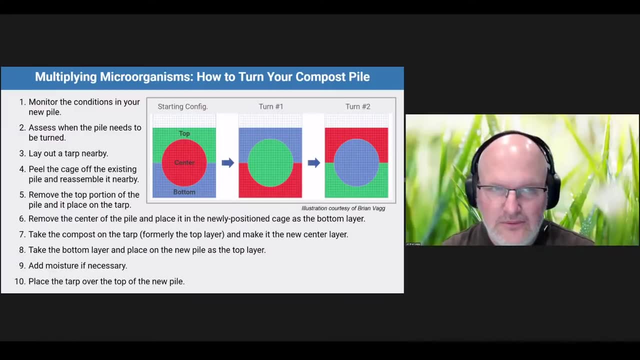 together this really beautiful diagram based on elaine's method. um, brian, you want to tell us about it. um, i mean, the colors are kind of self-explanatory: the green was the top, the red's the center, the blue is the bottom, to start with, and, as elaine mentioned, you want to get everything through hot. 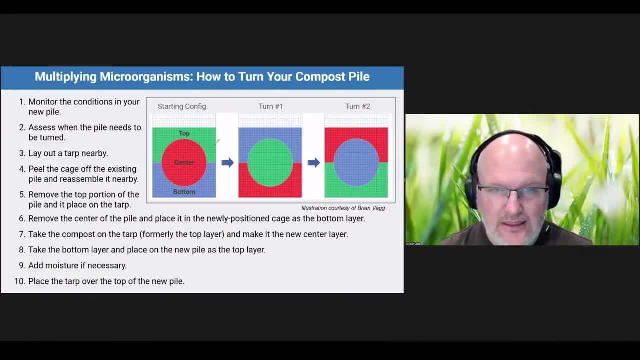 center. so your turning technique is important to make sure that you're able to get things through that hot center. so when you do your first turn, we typically make sure that the top, which was the top, now becomes the hot center. what was the hot center becomes the bottom and what was the bottom of the 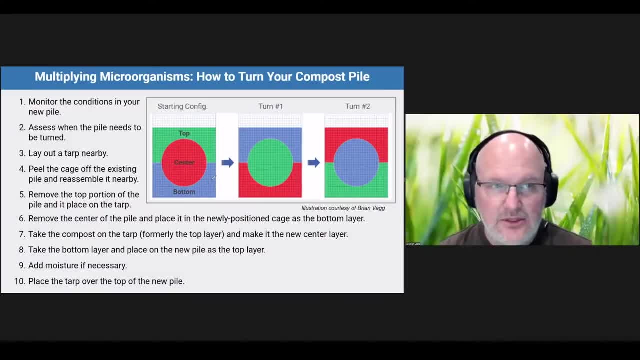 pile to start with now becomes the top. and then what is happening? do you get out of the purple around it because of the one dot and fill that hole up, get that under the bottom line there. at this point it's a little bit like jenga, right, you like jenga, you pull the blocks out. exactly. it's not that simple, but yes, it's. 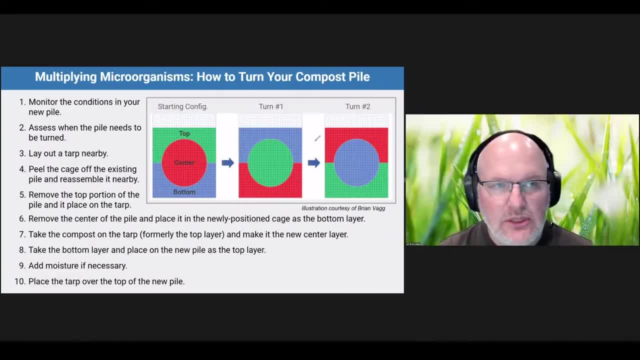 not that simple but close enough. and you know, um, everything elaine mentioned before about the temperature and the moisture, and and then having that as your guide to do the turning, you just want to make sure that you, you turn to get everything through a hot center, and we stopped the diagram at. And you don't have to turn five times what we've seen. as long as everything gets into that hot center and has the chance to deal with the disease or the problem organisms, That's all that you have to turn. So with the caveat that as long as your compost is still generating heat, you do need to keep. 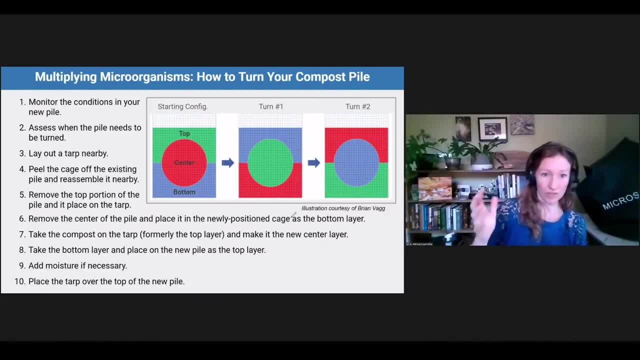 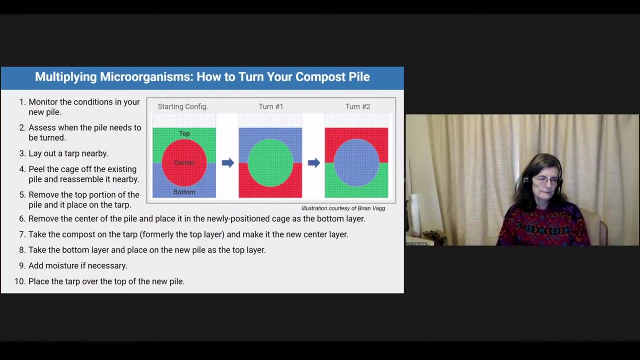 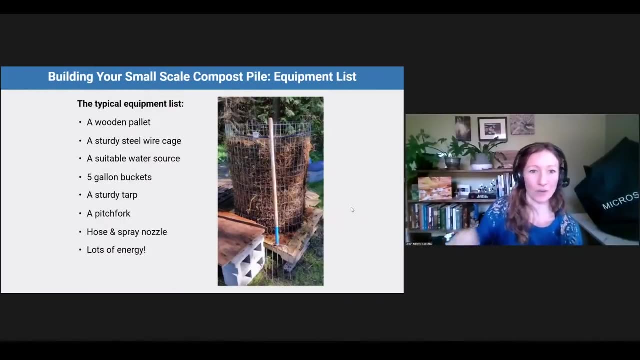 turning it right. If you have the heat that, you need to keep following those temperature, and any time you get to 170 again you got to turn the pile. Awesome, All right, Let's talk about the equipment. What do folks need to make a good compost pile? 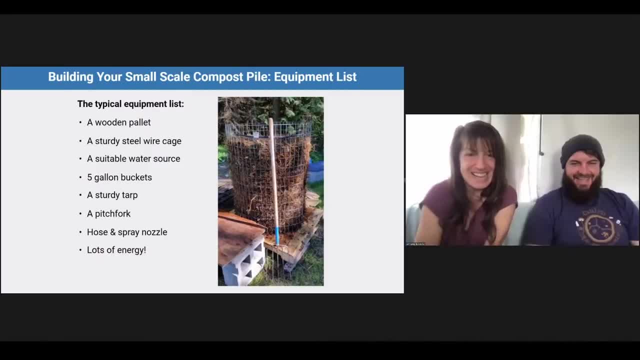 Casey and Keisha take it away. Thank you, Sure thing I mean. just I'm not really. I find that it's hard for me to use these cages because I'm so short, But They do work for holding the. the actual structure of the pile. 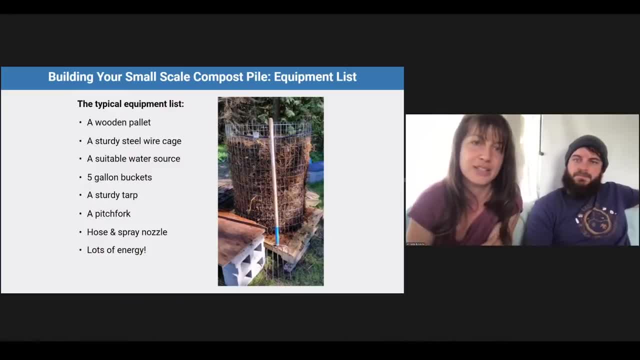 The wooden pallet is really useful if you're going to have a lot of rain so you don't get excess moisture moving to the bottom of your compost pile. That organic material is really good at sucking up the water and pulling it into the actual pile and creating an anaerobic condition. 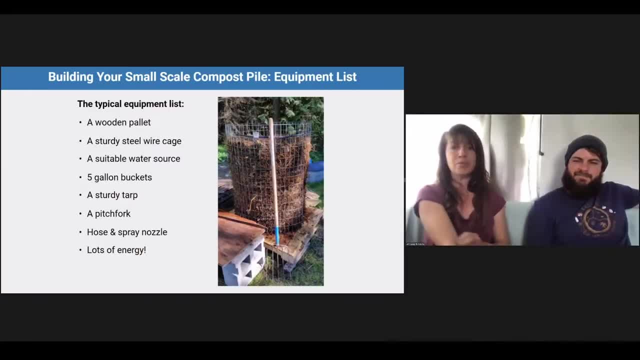 You're going to want some clean water, something some people have mentioned: the Boogie Blue filter that takes up chloramine and chlorine. You want something like that on your hose if you're using City water- five gallon buckets, or we use those 14 gallon totes if you've got a helper. 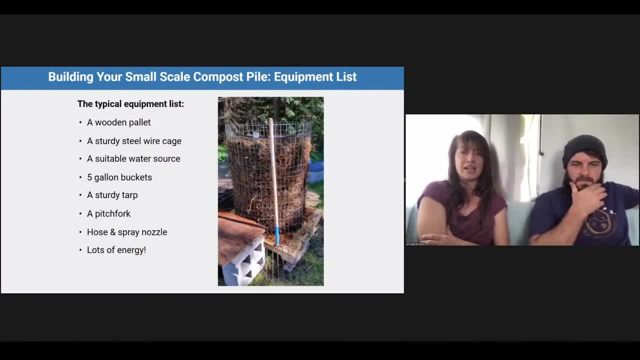 Five gallon buckets are very manageable and don't get too heavy. A nice sturdy tarp, a pitchfork- I mean, I could go all day talking about the tines in a pitchfork, but I won't bother you with that right now. 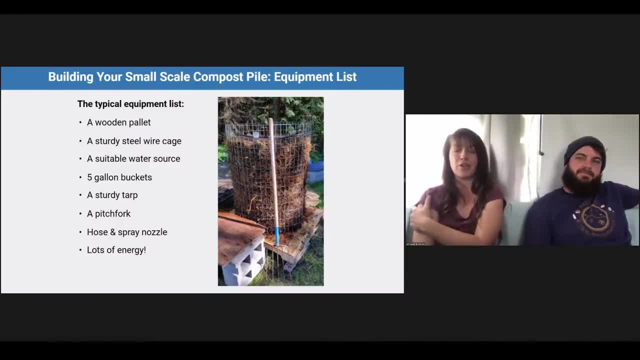 And then a hose and spray nozzle It's. it's nice to be able to stop that flow of water so you don't get a bunch of pooling in your work area and make it muddy. And then, of course, lots of energy. You're going to have to turn that pile and make sure it's all nice and mixed as you're building it. 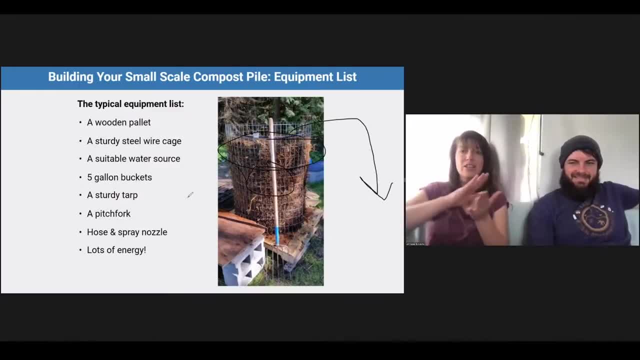 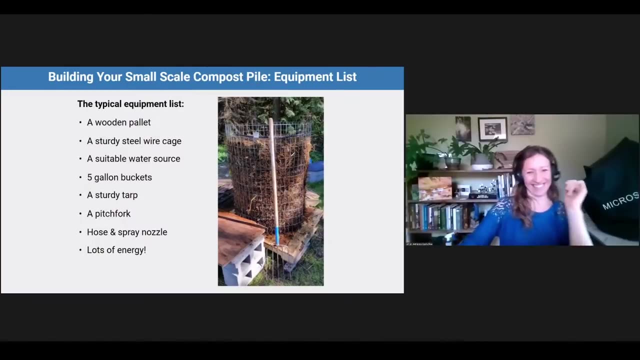 It's very important to mix that pile up and get nice contact with all the organic material to kick everything into gear. with the moisture: Wow, I like I'm building a pile for you. I like the energy, OK, Oh man, I do have to sit down every time I turn the pile, though, and be like: OK, what part's going where? 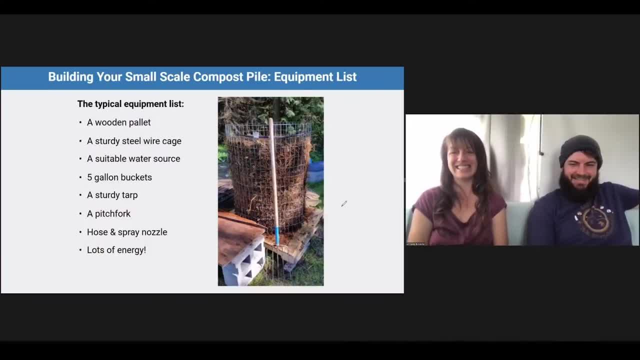 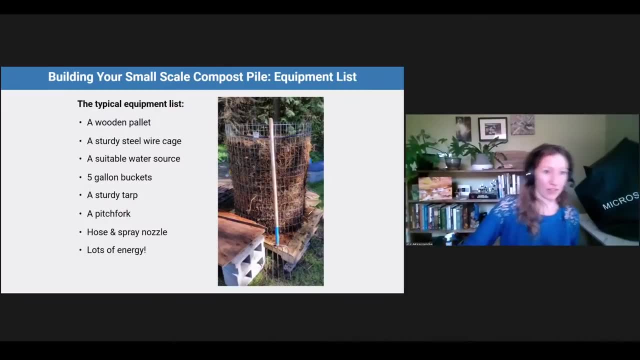 Because you know, just think it through- It does help to have multiple pallets so that you can start out your fresh turn on another pallet, so you don't have to move everything off and then rebuild it on the pallet. But yeah, And why? Why the wire mesh? 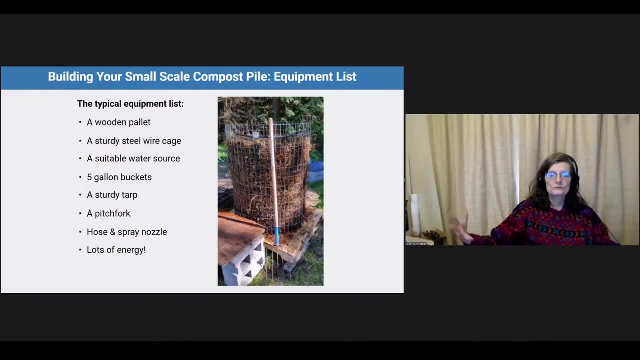 Why do we have that? So oxygen can move through very easily? Yep, Not, you know. notice that they're not real small openings, They're relatively large. But you just have to. You have to keep the compost in place, and usually it's pretty good. 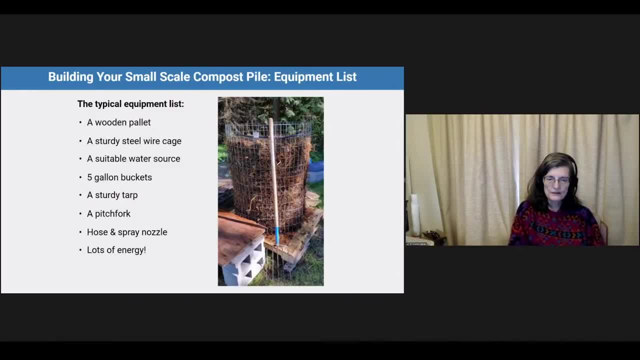 It's moist enough. We're keeping it at 50 percent moisture so you don't have, you know, the dry hourglass sand effect where everything falls through the openings, So you don't really need it. any smaller opening sizes than what we've got here. 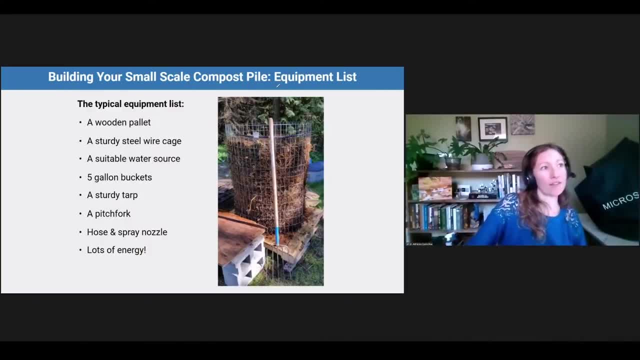 You probably don't want it. Depending on what kind of outside temperatures you're dealing with, I often will stick a broomstick into the middle- And I learned this from Elaine, of course- And drape a tarp over the edge. 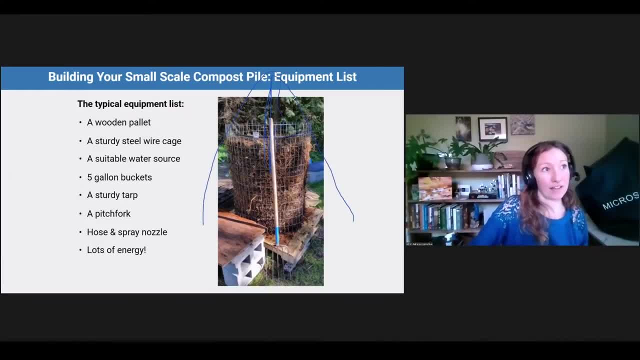 So that the tarp, the steam can rise and then dribble down the sides and away from the pile so that top of the pile doesn't get waterlogged. And that works really well for me. And then when it gets really cold you can kind of tuck the skirt in around the pile or bungee it if it's really intense, or let it flow freely on the hot days. 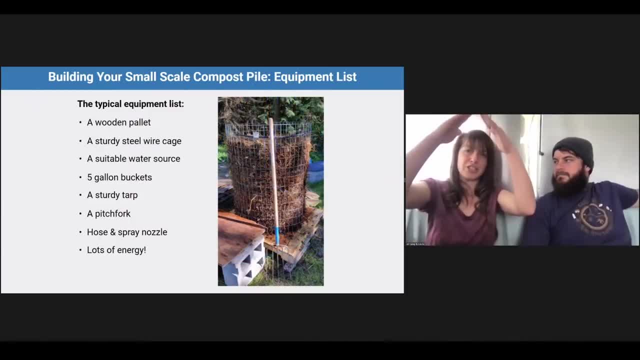 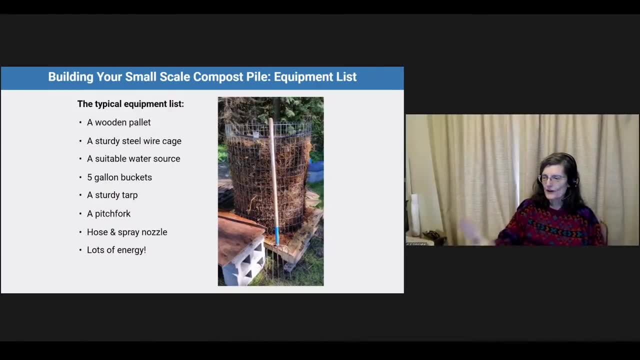 Awesome, Anything to add? Yeah, it makes. if you get the sheet propped up just perfect over that cage, it actually looks like a spooky goat. It's a spooky ghost. You're all set for Halloween. The composting, my friends. 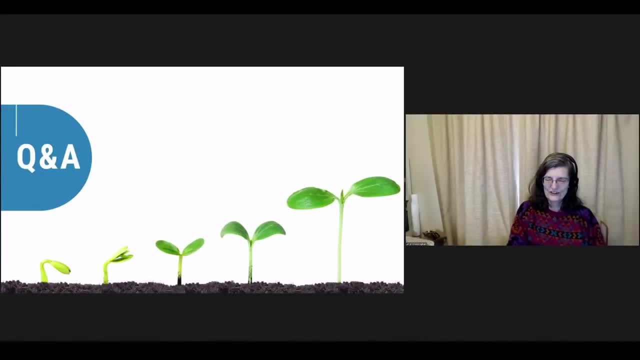 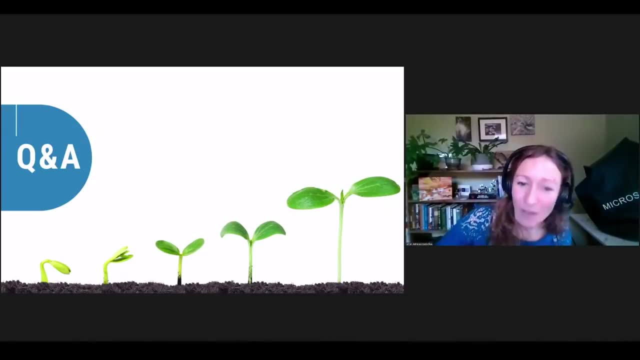 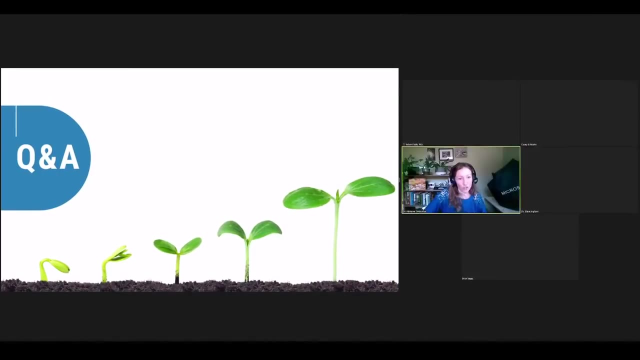 It's a compost compost. You're all ready for Halloween, The fun you have all been waiting for, and then submitting your wonderful questions. Let's start off by: how do I compost for sugarcane, which I think could either mean: how do I create a compost that can then be applied to a sugarcane field and grow? 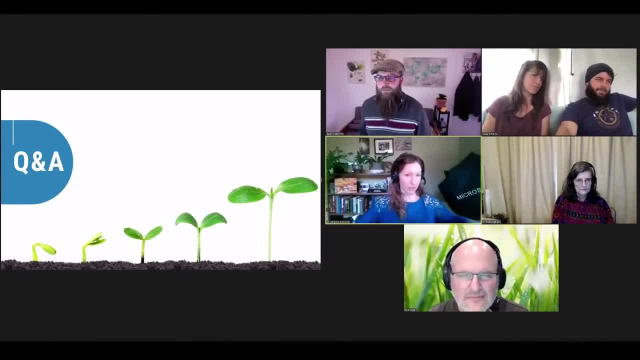 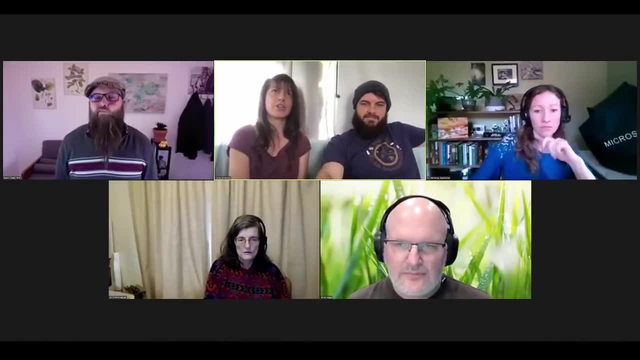 Healthy sugarcane or using sugarcane as a starting material. I'm going to let you all actually see each other and talk to each other. What do you think Sugarcane? That's a good question. You're going to want to think about whether it's already been juiced or not. 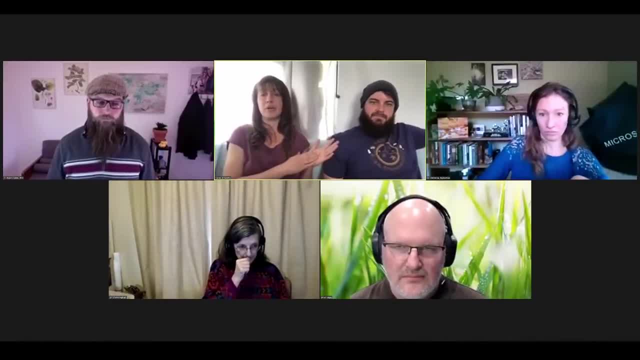 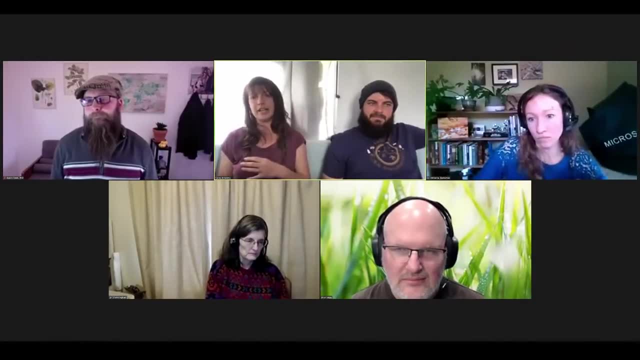 So typically when you get sugar pulp waste, it's going to be a brown material, because they have these machines that they squish the sugarcane and pull the juice out And that's the product that they're creating, And then the waste is actually that, that squished stem. So yeah, it's going to. It's going to depend if the sugar content is still in the stem for some reason, I believe it's going to react a lot differently than it will once it's been juiced. So if for some reason, I can't imagine why you wouldn't get all the crazy yummy sugars out of it before you're composting it. But if you are going to compost it whole, it's probably going to High nitrogen. Well, it's probably not going to be high nitrogen, It's going to be high sugar, Yeah, And that's carbon, Yeah. So your bacteria are just going to go. we have a grand old time and it's going to generate a lot of heat. 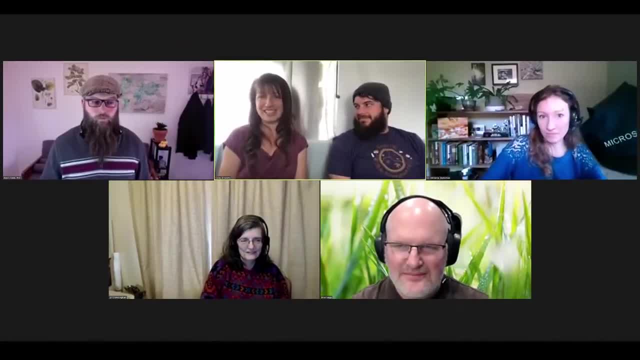 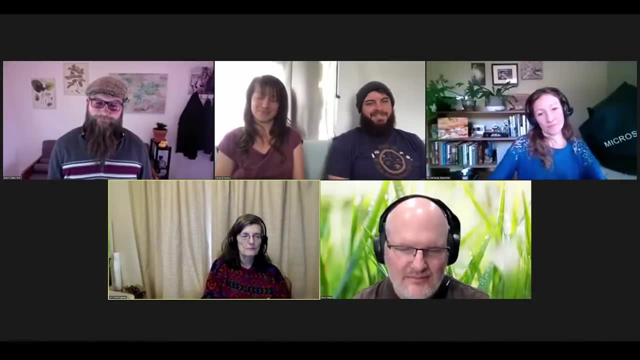 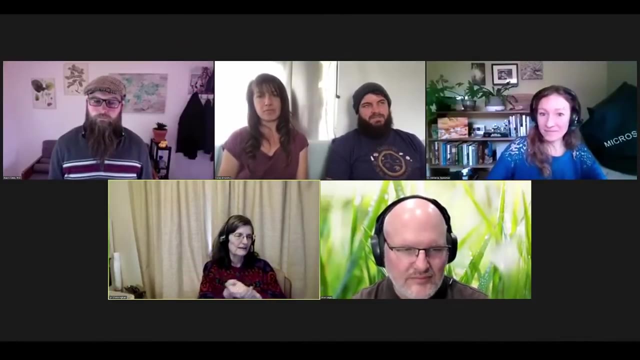 You're right, It's a super green You could call it, But given that most people don't grow sugarcane just to put it in a compost pile, I think we don't probably have to worry about that. It's all been squished and all as much of the juice as possible has been taken out of it. 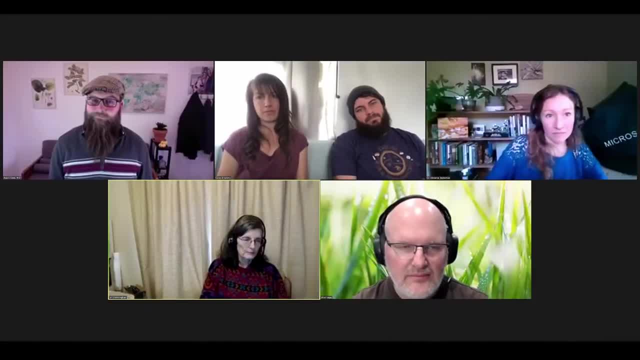 And it you know. so it gets dry pretty rapidly, And now you're dealing with something that's very wide C to N ratio, probably up towards the hundred to one ratio of carbon to nitrogen, So it's going to definitely be a brown material. So it does great, It makes great compost. I would probably break up the big long strands, You know anytime, if anybody's ever composted. but just by cutting you know grass, you know you're going to get a lot of compost. 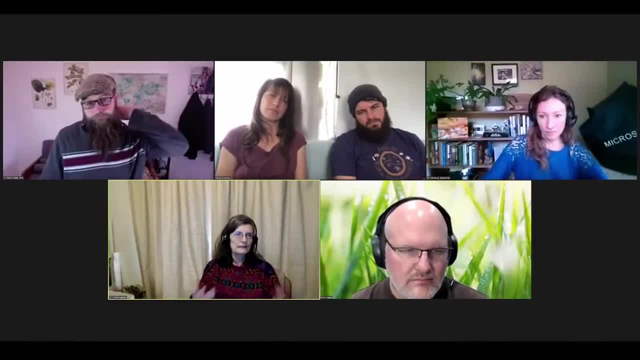 If you're going to put grass in a in a field and putting it in unchopped up, you'll realize how crazy difficult it is to turn a pile where you've got big long strands of grass. So don't do that. 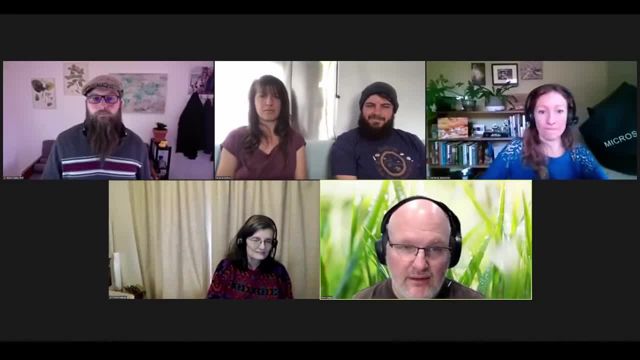 I can say from experience. I grew this rye that was about eight foot tall and I was like fantastic, Oh, that's great material. Well, I didn't break it down at all And then trying to turn that pile until about the fourth or fifth turn, it was just impossible. 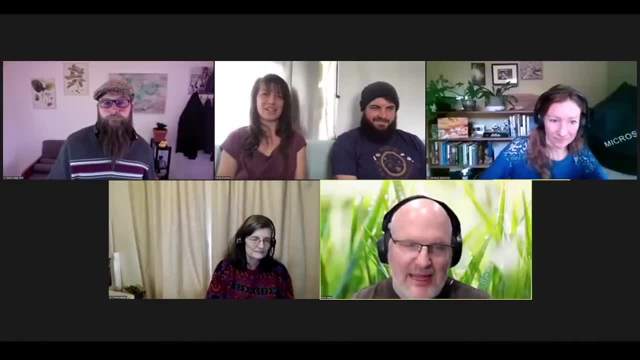 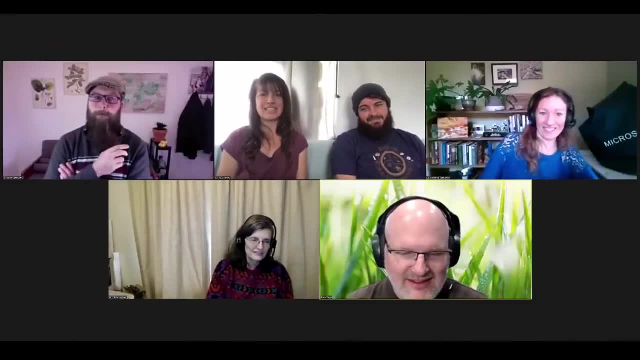 It was just all locked in solid mass. I had to take my hands and pull it all apart. Yeah, If you've got long strands of things that may take a while to break down, chop them up. Sounds like a job recipe for building houses. 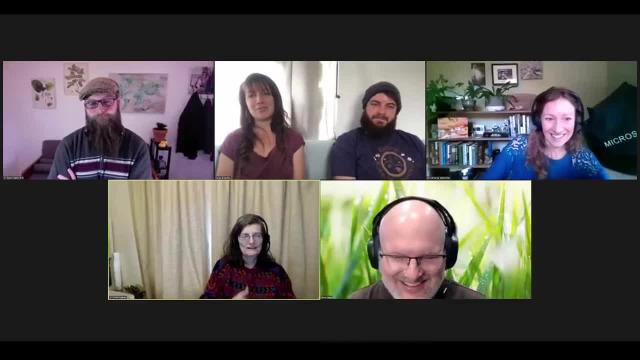 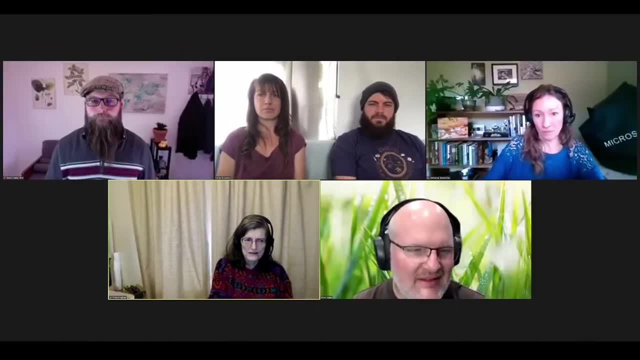 Would have been good for that. Yeah, So break them up. Yeah. And I just noticed a comment on the question. Somebody said that the sugar cane is high nitrogen. It fixes nitrogen. No, sorry, That's not the case. So 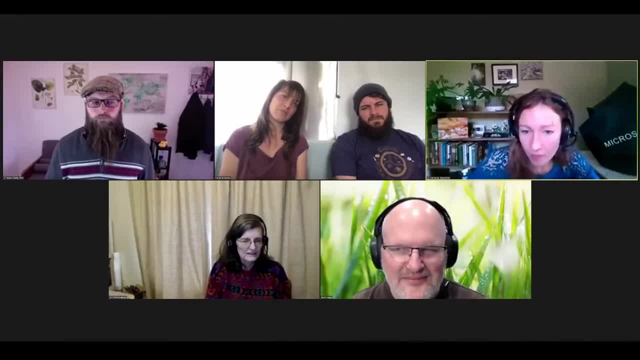 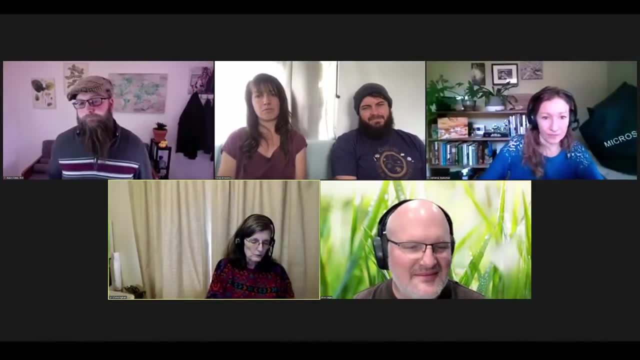 Well, I do want to clarify. We had a question about what is party food. Can you explain a little bit more about that? Party foods are the things I talked about, where you know manure of different kinds, given that you understand the caveats that you have to look into. Legumes of any kind. But you do have to make certain that there are nodules on the root system of the plant when you're talking about legumes and rhizobium. that system I know. when I was at Rodale I went out and looked in their soybean fields, assuming that that would be a really great nitrogen fixer, and pulled up the first plant and looked at the root system- not a single nodule. 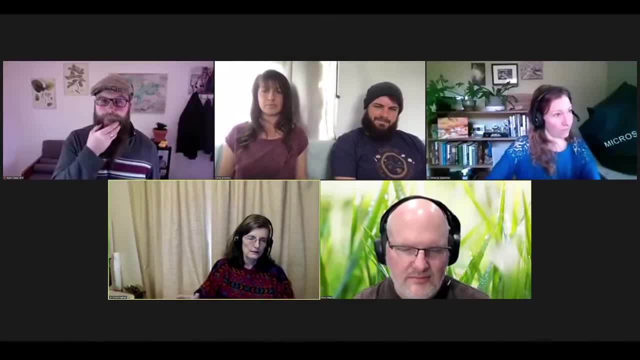 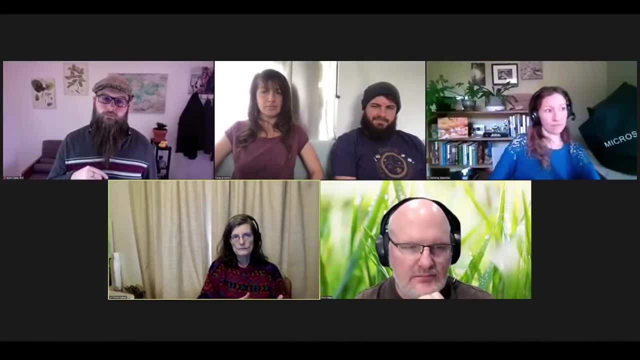 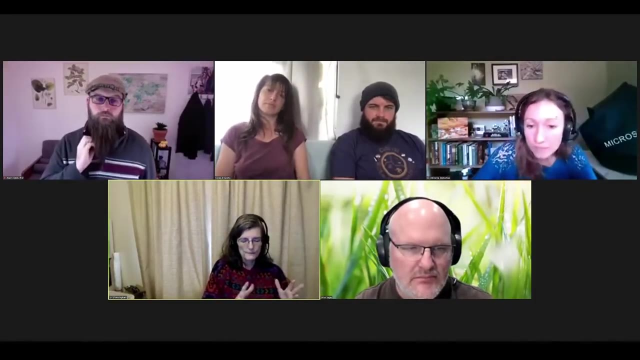 So the whole entire field, not a single nodule. So you got to be careful on that one. So high nitrogen is, got you know, typically Typically 10%, 5%, something in that range of nitrogen present. So, and I think we had those slides previously- 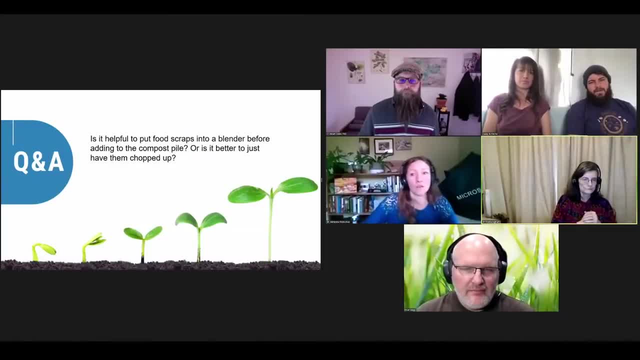 So I don't, I don't need to go any deeper than that right. Party food just really means that those are things that are going to help that pile get up to temperature fast. Those are what we call our party foods. Yeah, it allows those microbes to have a party right. 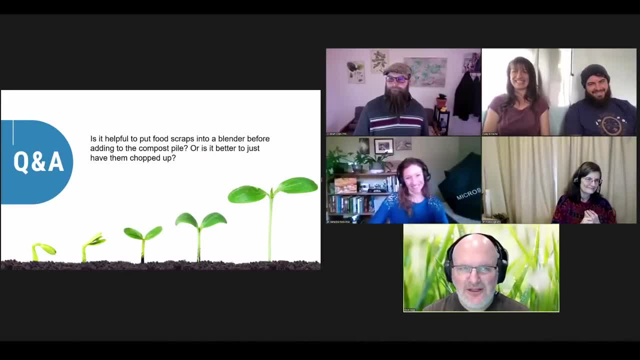 It's that heat generating from that reproduction. So, speaking of breaking up materials before composting them, we had one question: Is it helpful to put food scraps into a blender before adding it to the compost pile, Or is it better to just have them chopped up? 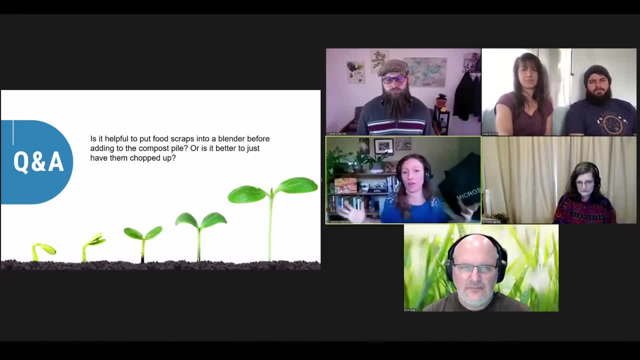 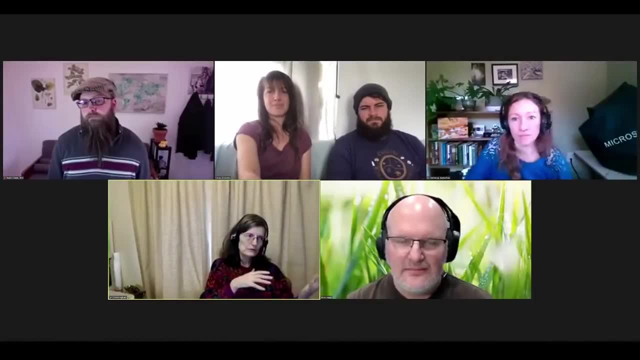 And if this makes you think of other starting materials in the size and how to prepare them, feel free to share that also. Well, microorganisms grow on surfaces, And so you grind something up, you break it up, So it's Kind of runny. That it's going to be used so rapidly by the microorganisms that you're going to get too much of a temperature burst And you could get real high real fast If you're, if you're doing that especially with veggies or fruits or something like that. So I don't like that Other. Yeah, You need structure to start with. If you have a lot of really fine Like using sawdust, it's not necessarily a great woody source, at least as it being predominantly your woody source, because you don't have enough structure yet built in that pile, but you can easily go anaerobic. You don't have enough pore spaces. Yeah, I don't. I don't like necessarily blending things up. Manures can be a little bit different in that sense, because sometimes it's hard to apply manure, Sometimes you make a little bit of a slurry with them, but but if you have the ability to keep them chopped versus blended, that's my, my opinion. 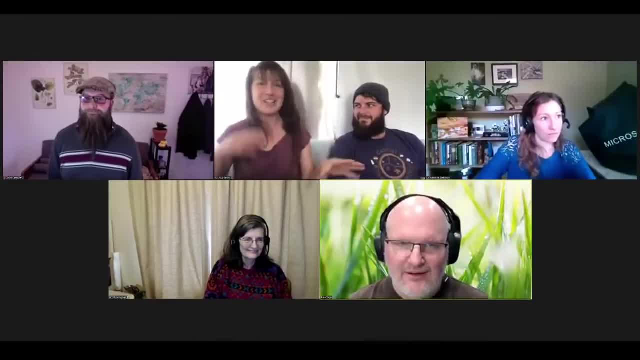 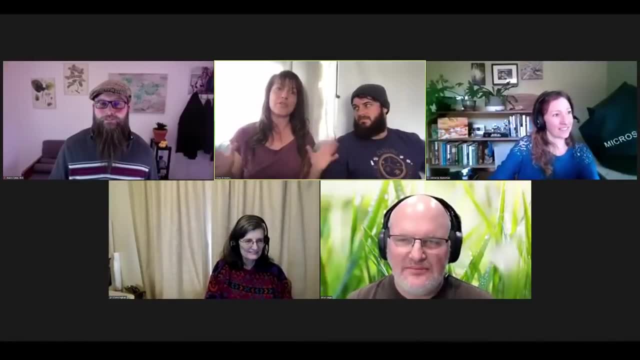 I want to be a little contrary here. Just with an All right, All right, I love it. Well with the with the food waste. actually it's. it's it's really a problem for some people to store their food waste. 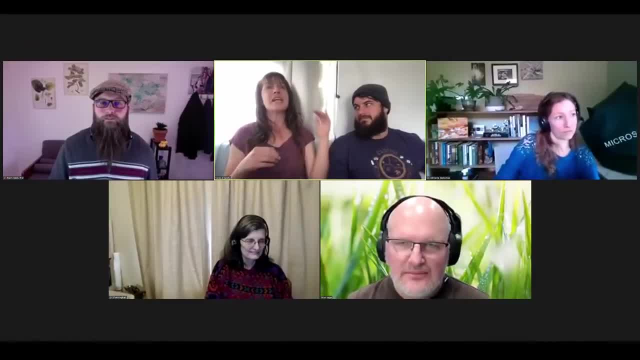 And so there's a little bit of an added procedure here. but if you do blend your food waste down and then you dehydrate it, it makes it more compact and it puts it in a state where it's not decomposing anymore And you can actually just save it in a five gallon bucket. 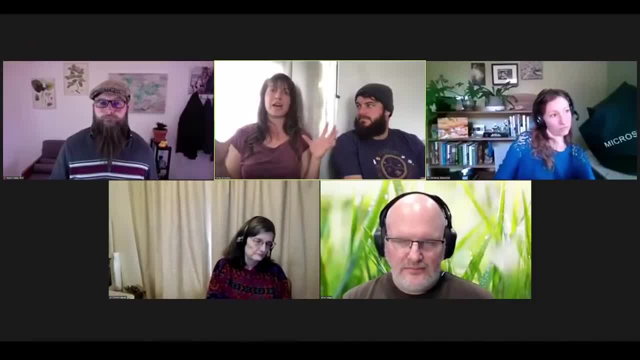 And then when you go to make your your hand turn pile, you have all this dried food waste that's been chopped down into small pieces And, like Brian says, you don't want too much of it, of course, because it's so much particulate, but you can distribute that through your hand turn pile. 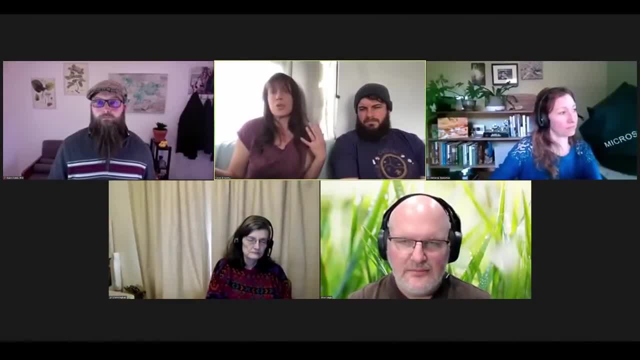 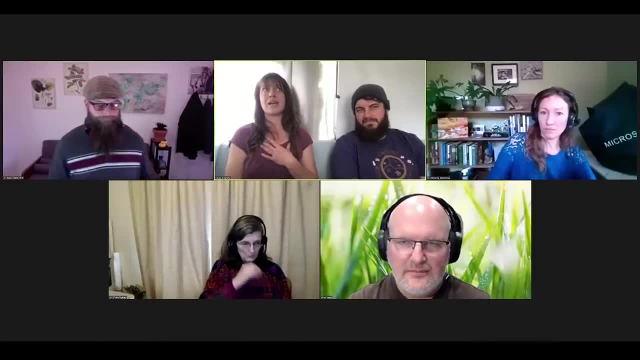 And it's just a way that you can hang on to, you know, maybe a year's worth of food waste without having to make that pile right at the moment, Because if you're like me and you cook a lot like I, just I produce a lot of waste and I rarely have time to compost it because I'm working. 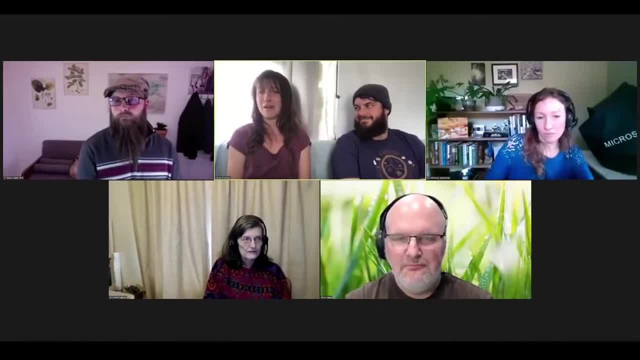 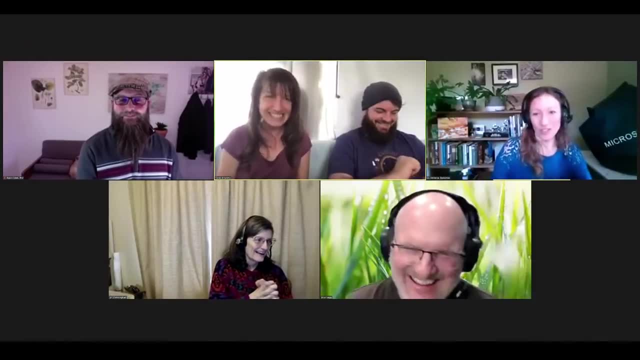 So I do like the blend and dry method. You don't have time to compost it because you're working on the compost. Yeah, Just checking. We're not technically allowed to use food waste in our product, Adrienne. Oh, interesting Really. 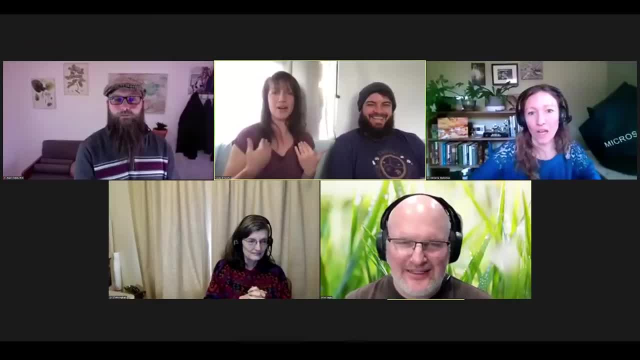 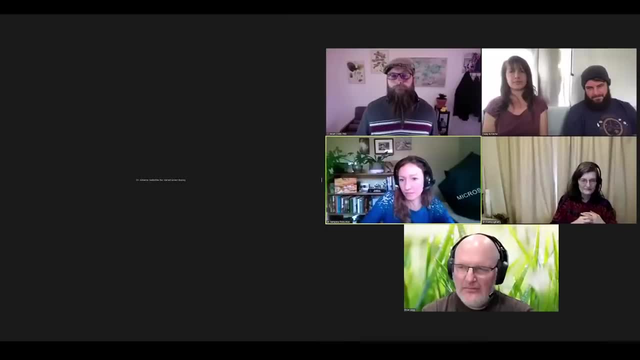 In case anybody from the CDFA is watching: I hear you, I hear you. Well, that's, that's interesting. That actually brings me to my next question, which is right. here Is a big static pile still best recommended for the everyday household? 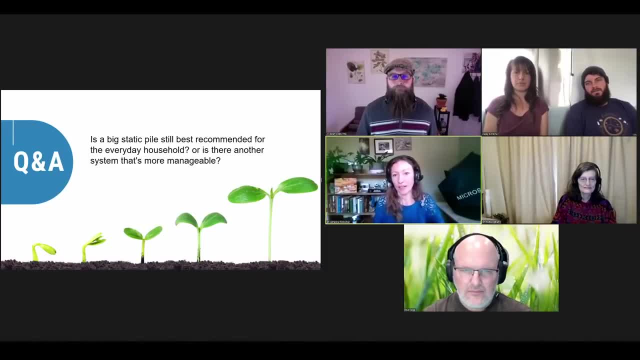 Or is there another system that's more manageable? So basically, how can you know your average homeowner deal with their food waste most effectively? We've been working with this a lot lately with the static piles And we've found that if you have a really nice biocomplete compost and you mix it in with that, it's not necessarily static. 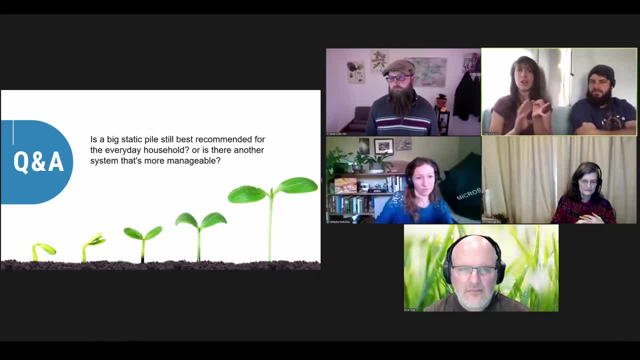 You still need to pay attention to all the things Elaine's talking about. Moisture really smells- Smells is a big one. And temperature, But our static piles, we still. we watch the temperature to make sure nothing is, you know, booming out of control and going higher than 131.. Or you know, we're not going to be able to do that, And so we're going to have to make sure that we're not going to be able to do that, And so we're going to have to make sure that we're not going to be able to do that. 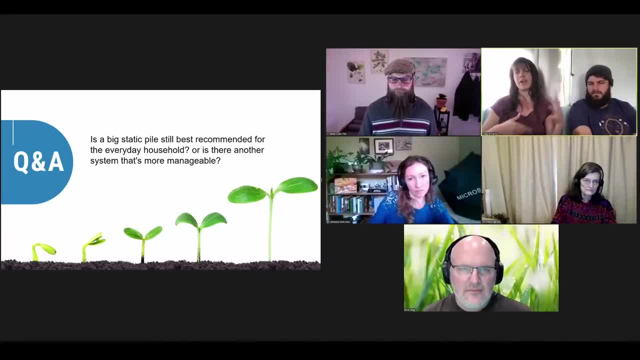 You know, up at 170.. But if you get a good inoculum in there and you mix it in with your yard waste and your food and your food waste, I've been seeing gorgeous microbes growing in static piles And you know the intention of those static piles is to use them to compost later in our thermophilic process. 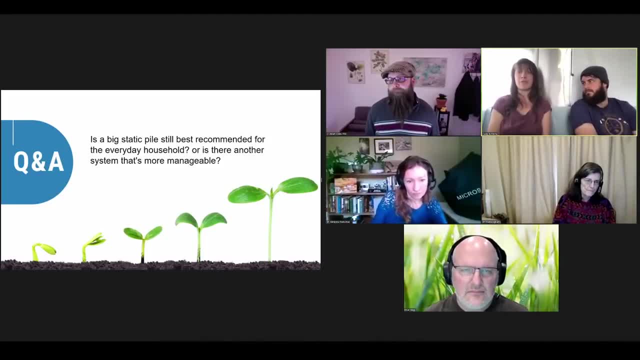 So I think that static piles could have a really nice place in our thermophilic system, as a, you know, as a holding space for microorganisms to grow while we wait for extra time for composting, And so, like in the Johnson-Hsu bioreactor, they basically make a compost pile a static compost pile. 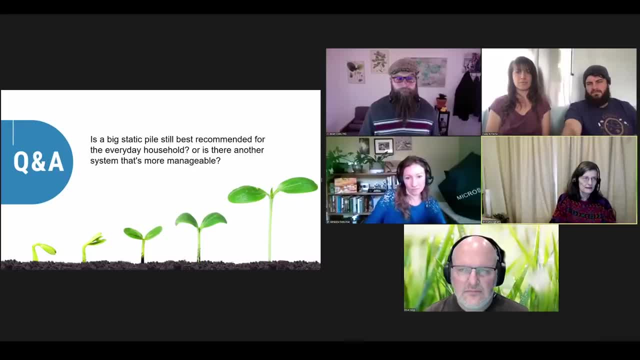 They don't add foods into it the way you would in a household situation with a kitchen waste. But at the end of composting for a month or so- a month to three months, I think it is- they now take their thermal compost. 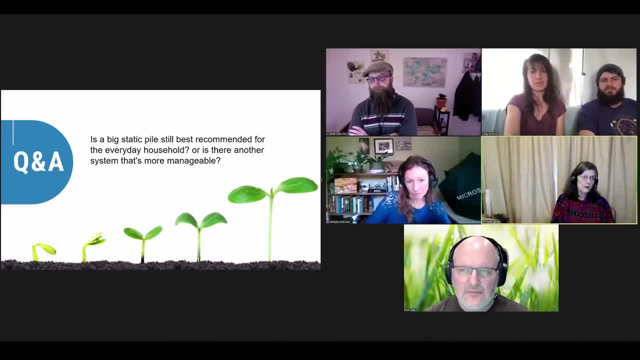 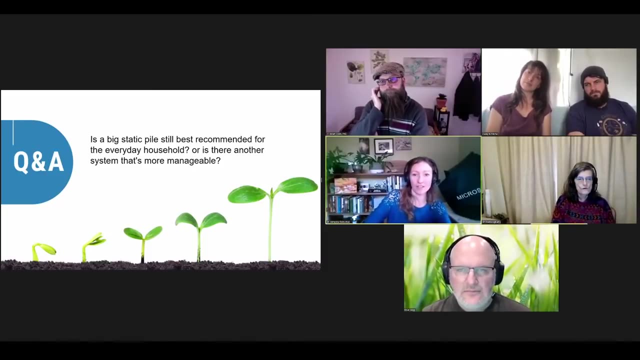 And run it through a worm bin, And so it's kind of two ways to make absolutely sure there is no disease-causing organism making it through in the finished product. Some of the most beautiful biology I've seen started as a thermophilic or a static pile that was then used as starting material for a thermophilic pile that then was fed into a vermicompost pile. 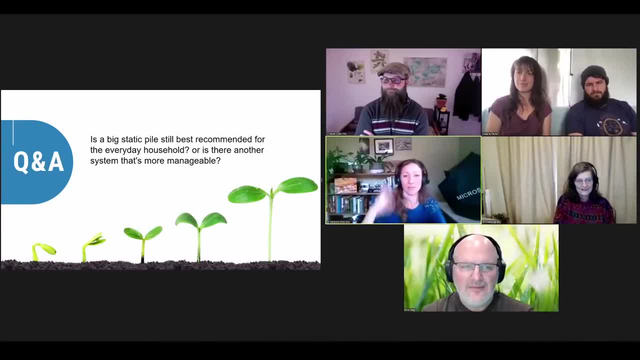 So it had like multiple layers of composting and it just got to mature. Wow, It's a little overkill. You know, one thing I like about household waste is vermicompost. You know, it's a system that's easy to put the food waste in a regular basis and the worms are happy to deal with it. 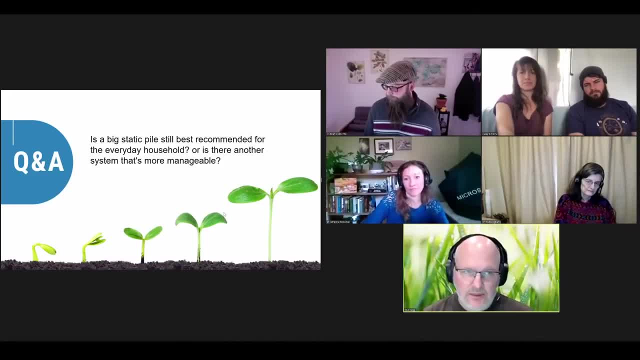 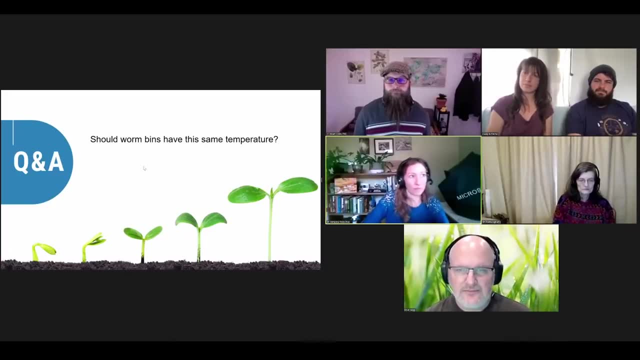 I mean you need to make sure you put a good vermicomposting system in place, but you can do small-scale vermicomposting very successfully. Speaking of Brian, should worm bins have the same temperature? I assume this is referring to the thermophilic temperature guidelines. 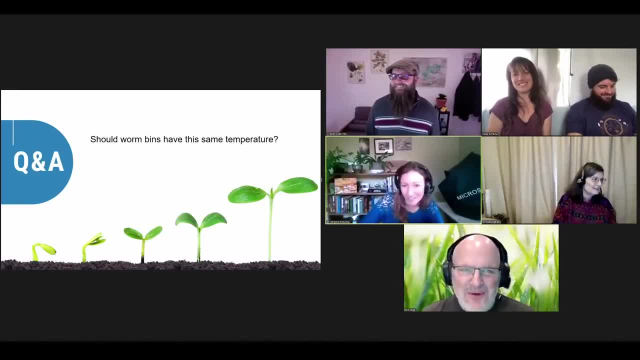 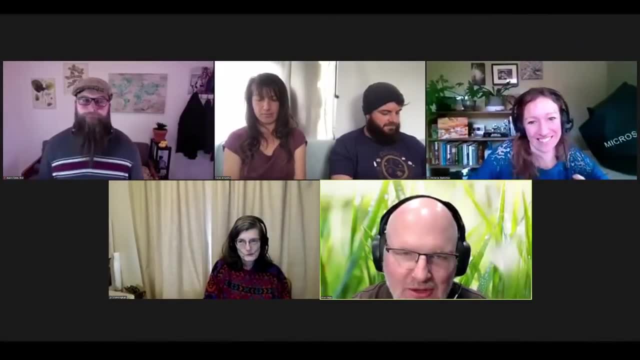 No, No, you won't. Why not Tell me about worms? They will split. It gets too warm for them. So yeah, you know worms are going to be, you know, composting a little bit differently: They're going to be shredding, consuming it. 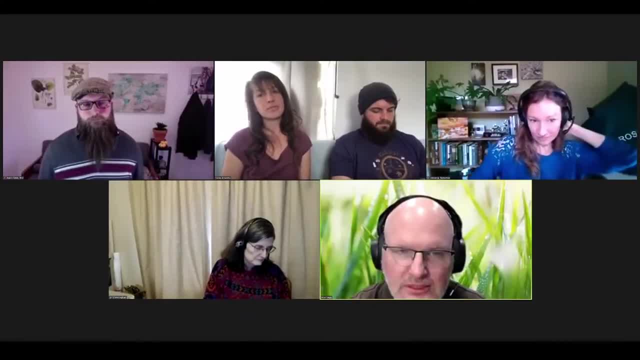 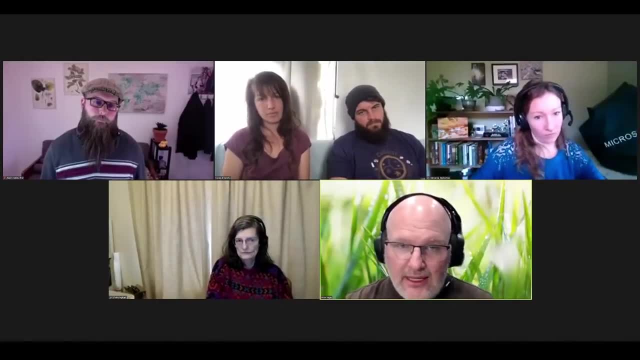 In their gut it's going to be a lot of microbiology that's going to help them also continue to break down those organisms. So vermicomposting is definitely different from thermophilic composting. Now, as we just talked, you can do thermophilic composting and then do vermicomposting on top of it. And I have to say that almost every one of my thermophilic piles have basically turned into vermicompost. You know, after about four or six months of me just storing that finished thermophilic compost, there are tons of worms inside of that compost. Yep, you're getting the benefit of both. Good job, Right, and Johnson's two piles become a vermicompost after the worms get added in that final stage, right, Yeah, Yeah, just try to keep the worms out. I've never been able to. 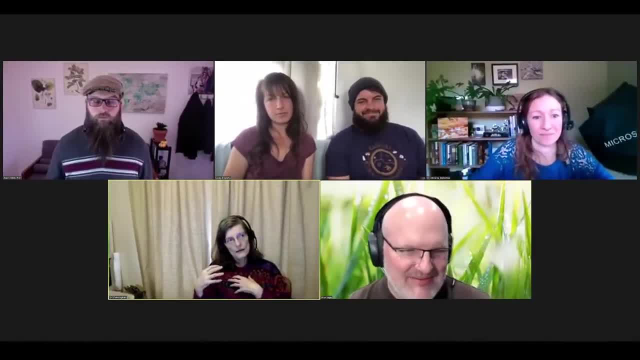 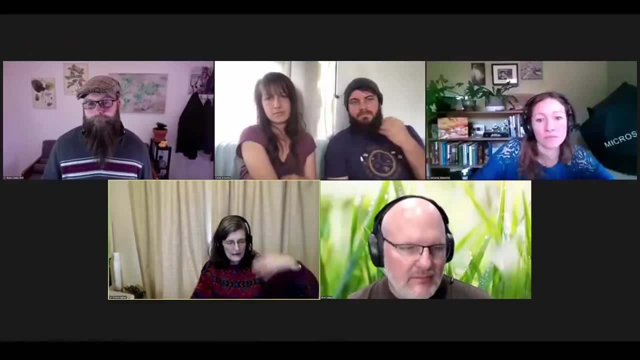 When you think about humans, Human beings and worms have a lot in common actually, because if you can't put your hand into that pile without going, yeah, oh God, that's hot, neither can the worms, You know, they just don't. we can't hear them say, God damn, that's hot. 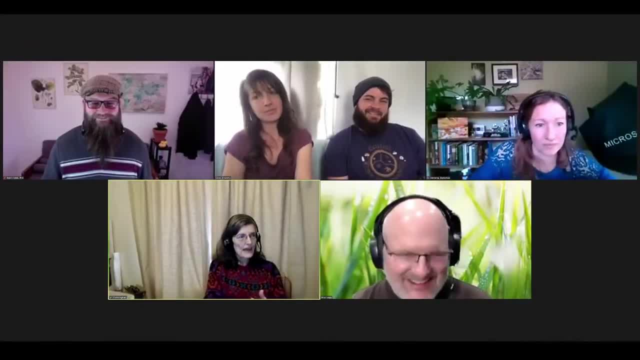 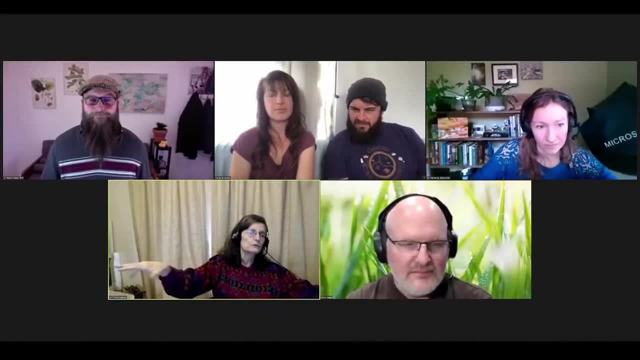 Ouch, I'm out. Yeah, and they usually, if that heat doesn't out and out, kill them right away. then they're going to go for the edges of the pile and try to escape out of the pile and go elsewhere Where things aren't quite so tough on them. 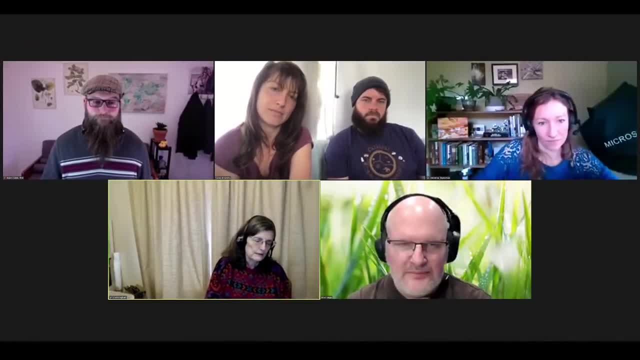 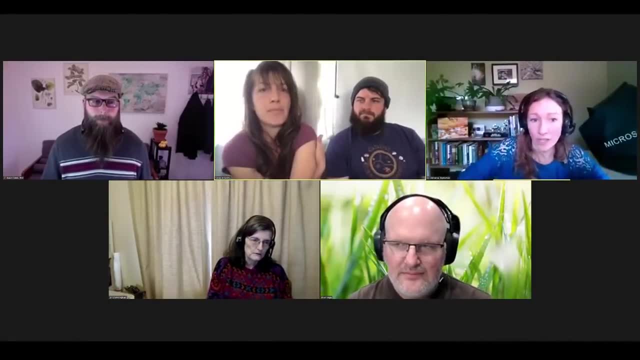 So yeah, you're not ever. you shouldn't ever put worms into some compost. that's that hot that it'll kill them. People are vice versa. What kind of material should you not put into a worm bin? People are bringing it up right now. 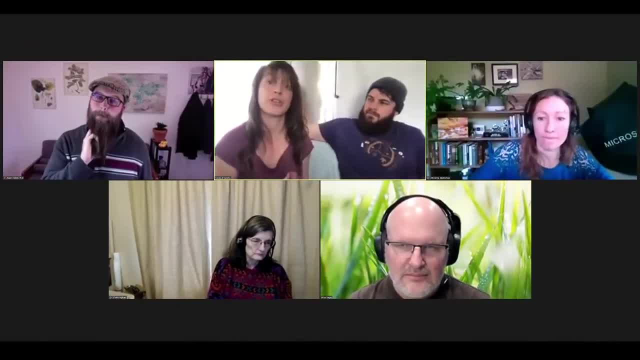 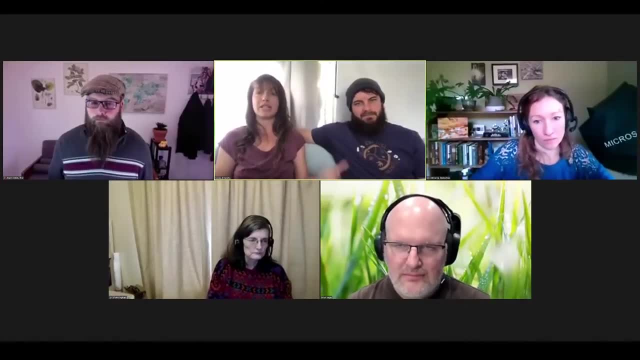 If you do have this excess amount of food waste, which will generate a lot of heat, you can freeze it or you can dry it And, you remember, you can always use solar dehydration. That's a much less wasteful way to dry products. Then to use the power in your house right. These things are easy to build outside and a great way to dry any materials at scale that you need to put in a worm bin so it doesn't get too hot. Just doesn't work in high humidity areas. If the humidity is 90%, yeah well, it's not going to dry down. So you have to have backups for those periods of time in your annual calendar where you can't dry it down. Oregon: in the time Period from October 15 to July, it rains all the time and Oregon's a special case from California. 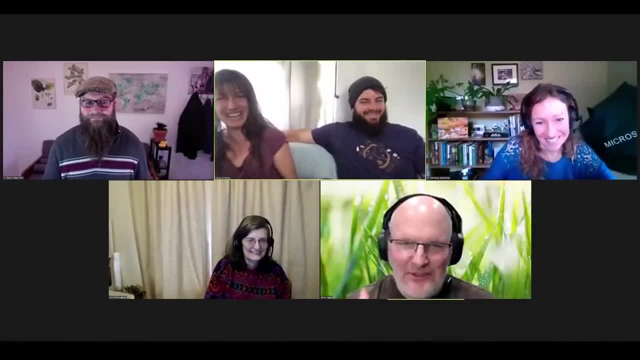 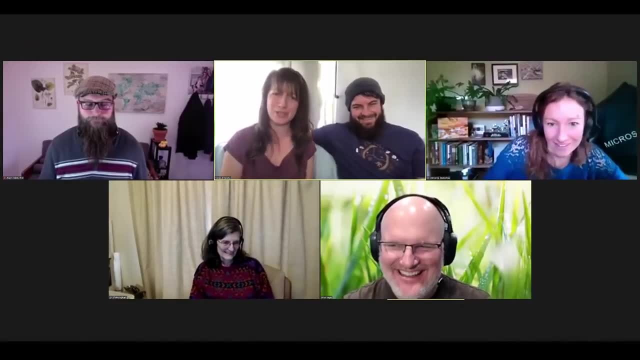 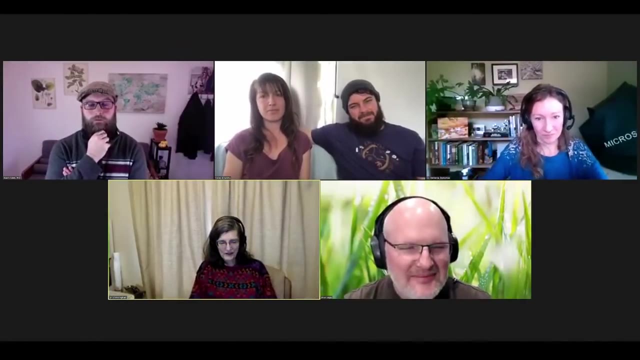 We can drag things out all the time, Even when I'm learning that from California to Oregon, you can dry your rivers down to very effectively. Oh man, there is an aspect of climate in all of this. Mm, hmm Well. 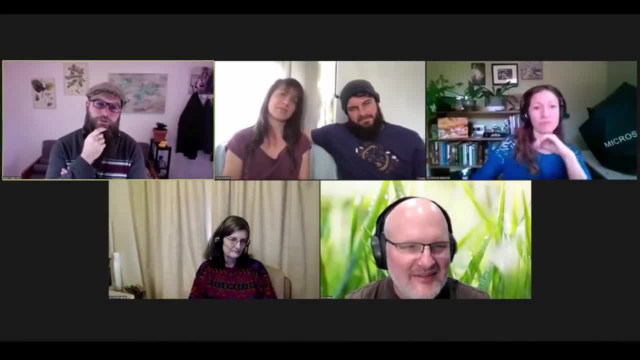 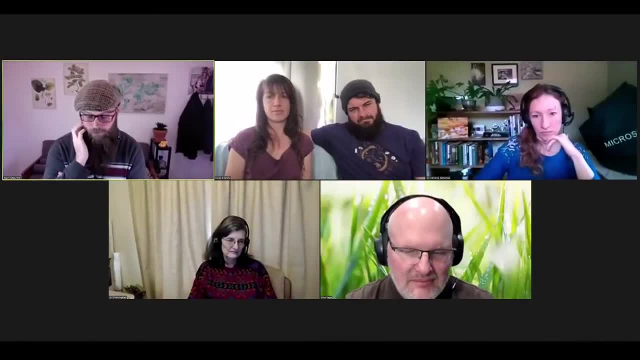 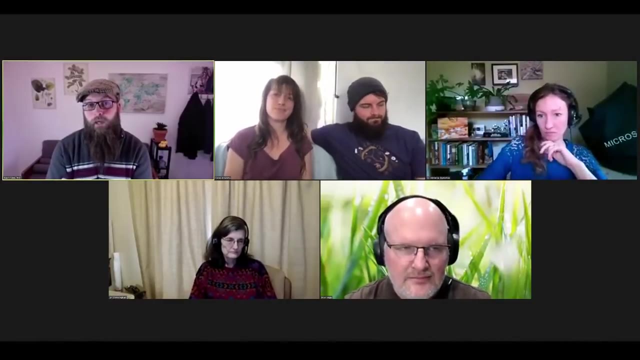 we're talking. oh yeah, Adam. yeah, that you posed about some things to be aware of with vermicomposting, which I had some experience with before I came to Seoul Food Web School. So sometimes people make the mistake of loading the worms up with too much material at a time and you can deal with compaction issues. 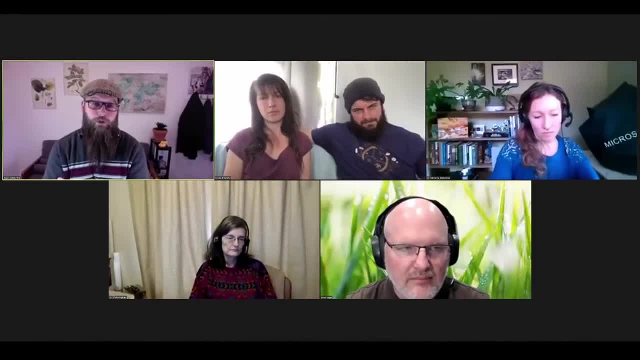 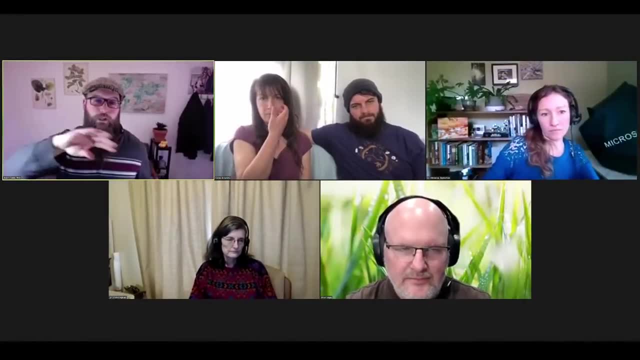 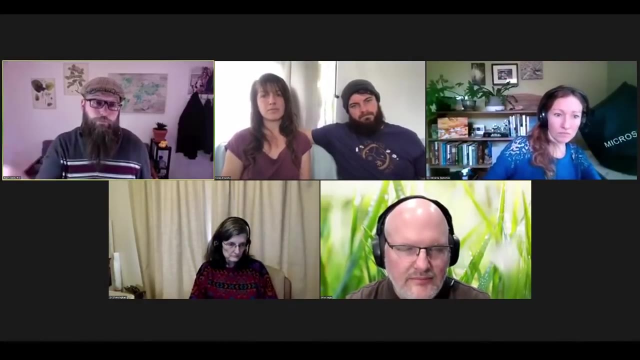 You can even basically smother your worms, depending on those kinds of things. So having more of a thought process that it's a flow through system from top to bottom And that the worms are eating the material- especially if you can have a system and they're out there even at small scale where the material falls through as it finishes- can be great. 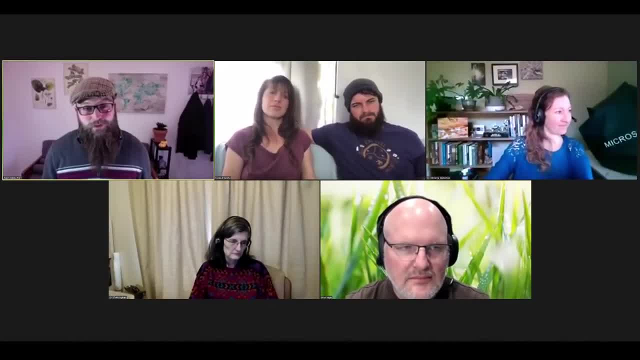 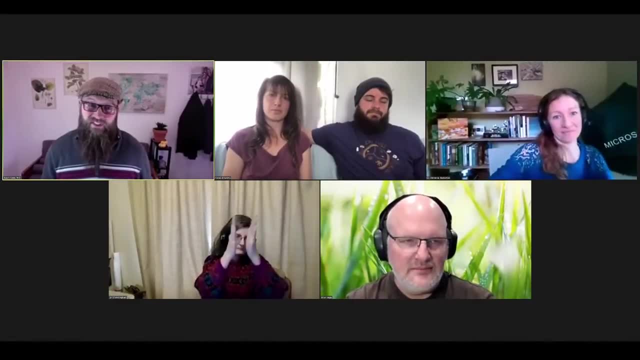 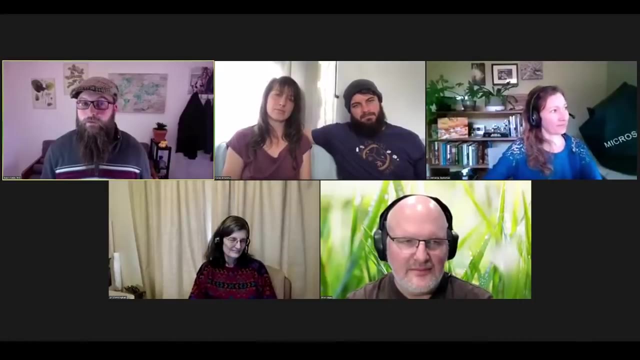 And I was just talking to one of our Seoul Food Web Associates today who said he's getting like a five to one fungal to bacterial compost consistently out of a very small kitchen based worm bin process And even if that's not enough material, That's not enough material to cover all of the needs of your farm and garden. 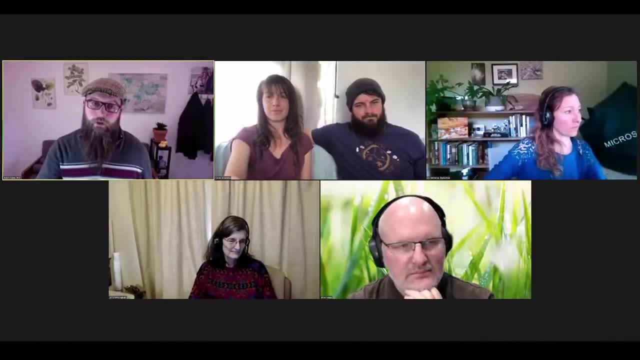 You can use it to inoculate other piles as they're maturing. You can use it just when you're transplanting little seedlings. Maybe if you have a high value crop, you can put a little bit in with each seedling, because it's like black gold, right. 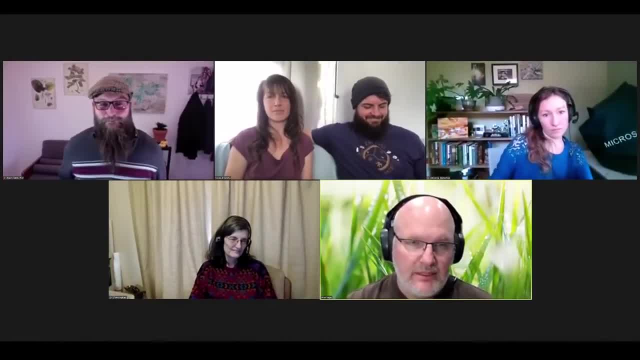 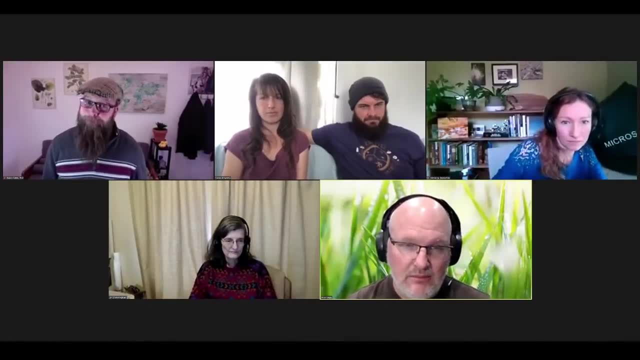 Well, you know, Elaine was talking about thermophilic piles as a recipe, right? How much high nitrogen green in, in similar sense, vermicomposting? there's a recipe there as well. Like you mentioned, Adam, You have to have. You have to have bedding material which is, you know, going to be a woody material that you can't load up with too much high nitrogen and too much green material. You're going to have anaerobic conditions occurring. You need to have grit or sand or something, some other components, to help the worm shred and break down that material. So yeah, once you get the recipe set right and you're adding the appropriate amount of foods, then you can really get your vermicompost to sing Okay, Related question. I'm going to pop it up here because we have a bit. 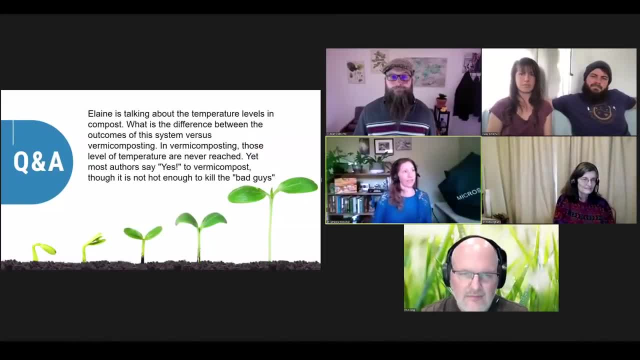 A few words to read. So Elaine is talking about the temperature levels in compost in our presentation today. So what is the difference between the outcomes of this system versus vermicompost, which is warm composting? in vermicomposting, those levels of temperature never reached yet. 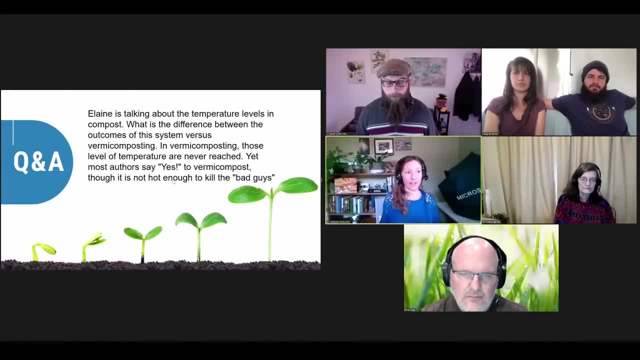 Most authors will say yes to vermicompost, even though it's not hot enough to kill the bad guys. So how can we trust them? Yeah, What happens to the material that the worms are ingesting? Yeah, What happens to the material that the worms are ingesting? 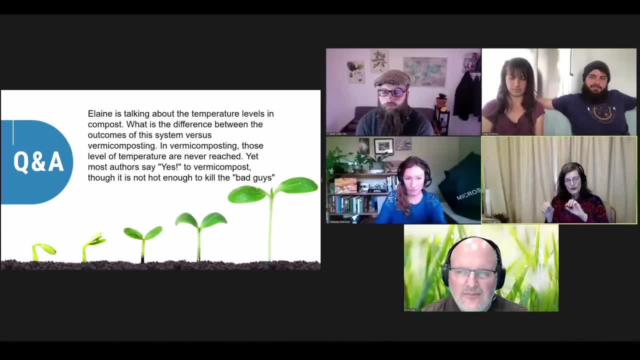 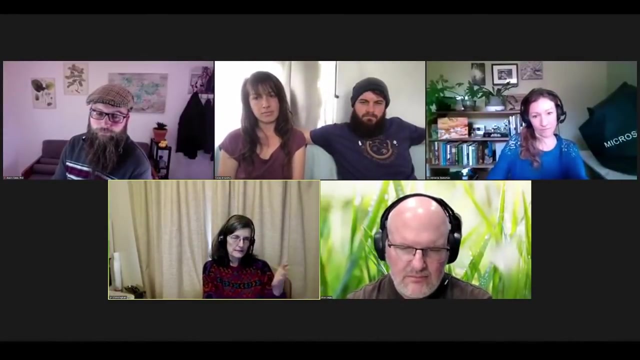 What happens is it's going through the digestive tract of that worm And there's several studies that show that. you know, if you've got 10 to the 6th E coli or salmonella in the materials that the worm is eating by the time it makes it past the crop, the beginning part of the earthworm, that the salmonella level has dropped by four orders of magnitude. 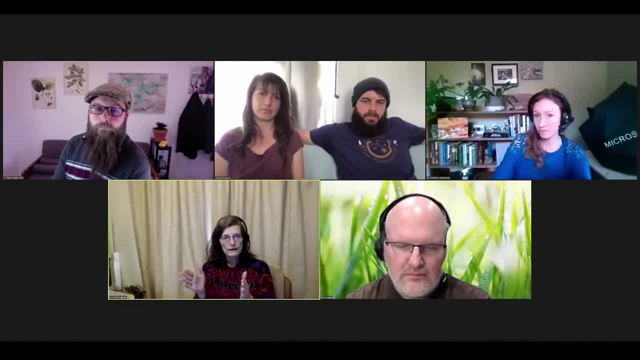 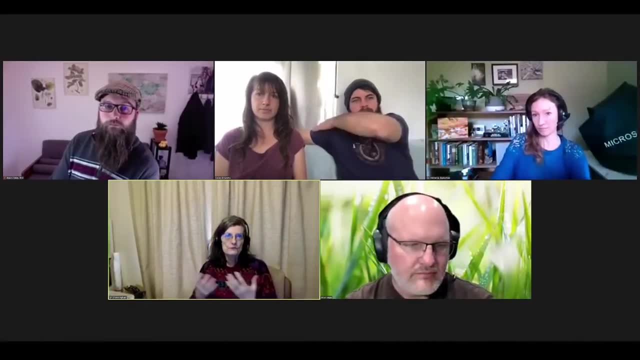 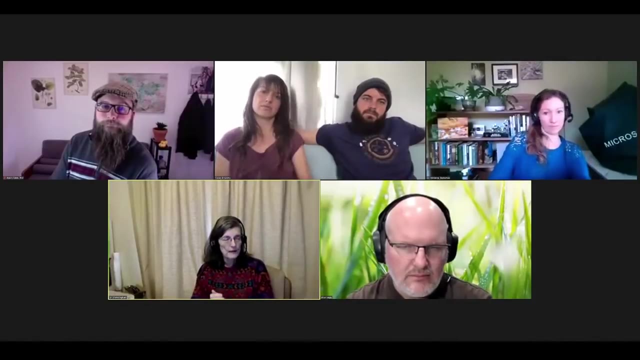 As it moves into the back part of the worm and moves into that large cavity where you have just massive numbers of really beneficial organisms: fungi, protozoa, bacteria, of course even some nematodes, permanent residency basically in that area and a high growth rate. And that basically wipes out all the rest of that salmonella population. So all the time it's what's going on in that earthworm's digestive system is extremely detrimental to the disease-causing organisms, which is why you want to keep your worms happy. 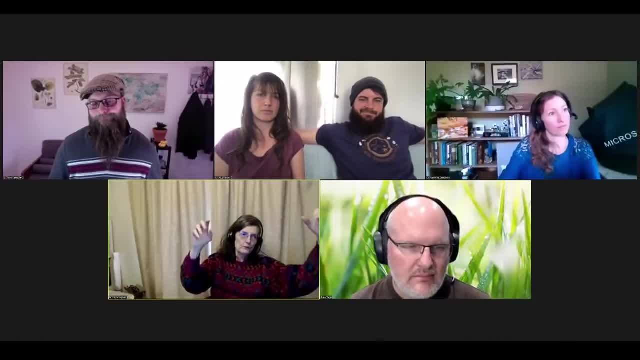 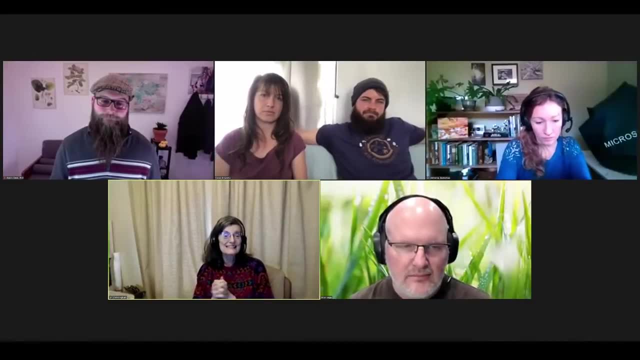 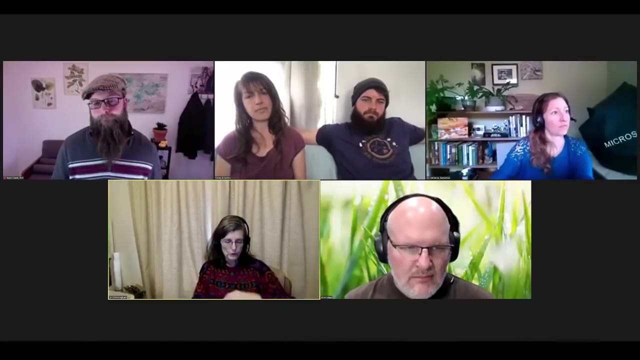 When you see your worms trying to crawl up the side of your worm composter and escape out the door, that's telling you that disease suppression is not happening here. So even on the outside of the earthworm where we've driven, We've dropped worms onto petri dishes where we have a lawn of salmonella or shigella or one of the pathogens- human pathogens. 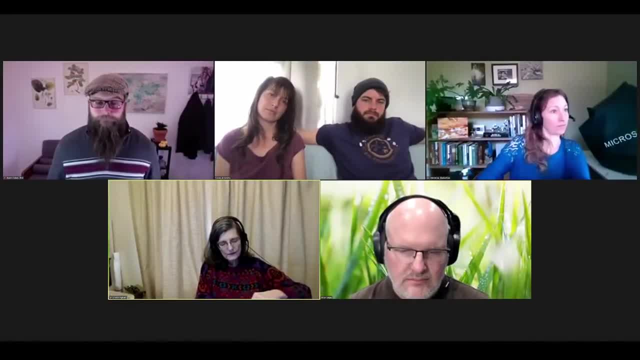 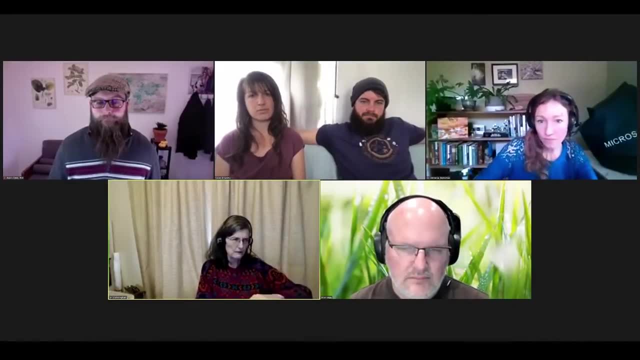 We drop a worm onto that surface and let them go for the time before they poop. So you're pulling that worm off after about a minute. The next morning you can see. well, you put the petri dish back into an incubator. pull it back out in the morning. 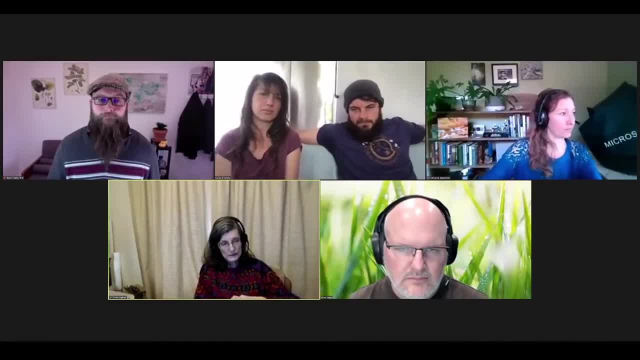 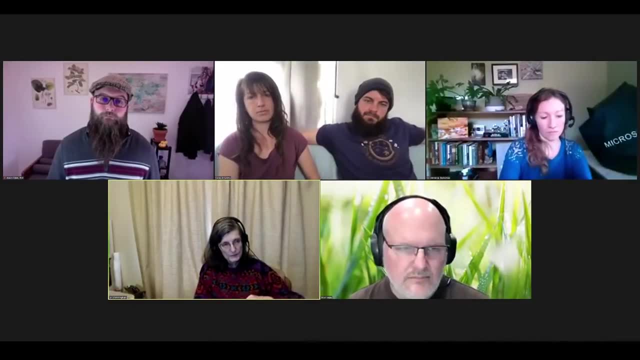 And you can see that the area that was cleared by the earthworm eating the bacteria has now expanded to twice, to maybe three times, what it was from the direct effect of that worm, And that continued death of the pathogen is due to the organisms that are on the outside of the earthworm growing, consuming and thus replicating. 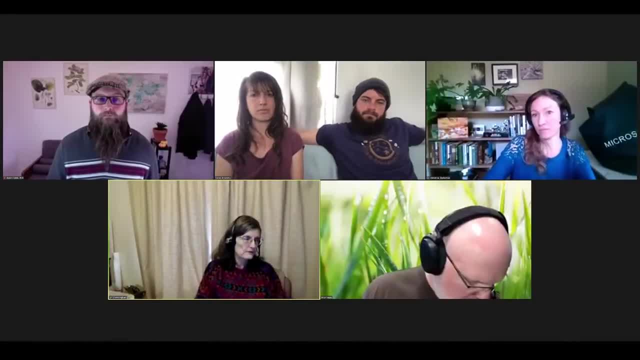 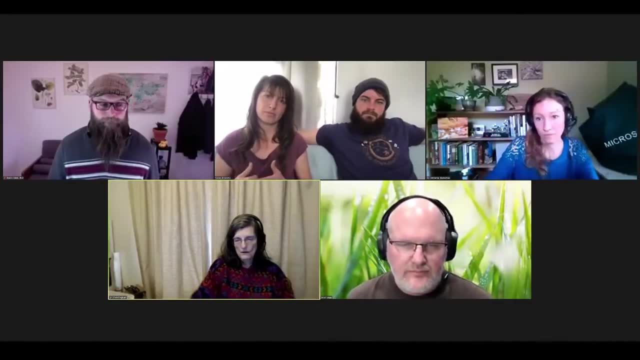 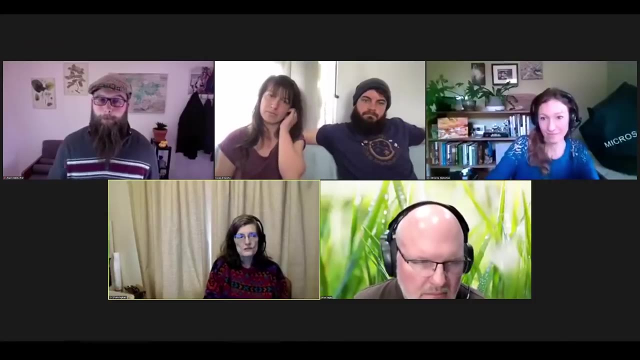 And killing off the rest of the salmonella or shigella in that petri dish. Within four to five days all of those bad guys are gone. You would not know that that had been covered by horrible disease-causing organisms when you first put that worm in there. So different mechanism. The worms do it by competition inhibition and consumption. And the worms do it by competition inhibition and consumption, Whereas in the thermal piles it's getting hot enough, long enough, temperature, I'd say. one other big benefit of thermophilic is it kills the seeds. It kills weed seeds. It kills any of the plants that you're putting in there. That's one thing that worms aren't going to eat. They're not going to eat the seeds. So thermophilic is great for making sure that you're killing off any invasive species that you may be using in your compost as you're creating it. 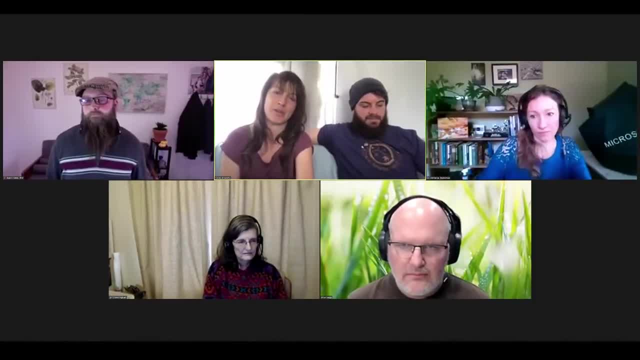 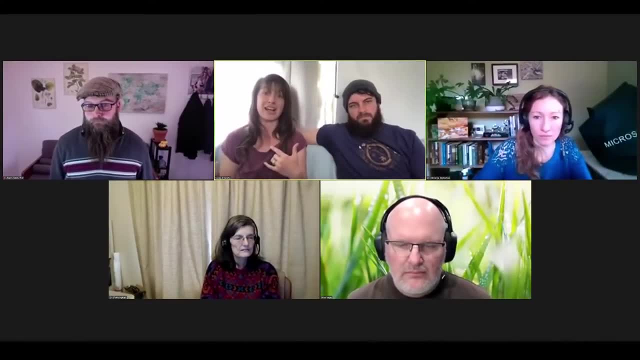 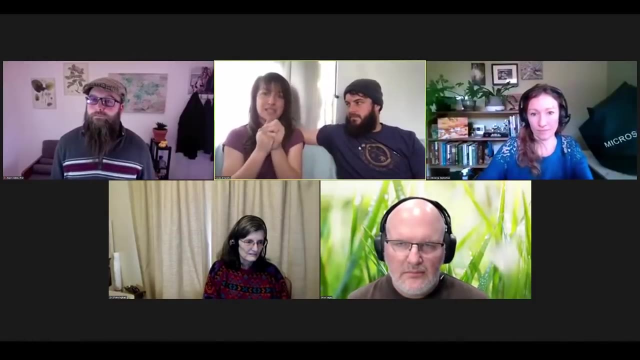 It's also a good idea to mention predation. It's a good idea to mention predation. You're talking about thermophilic compost or worm compost or static compost. when you have a diversity of microorganisms there, they eat each other And I've seen it live on the microscope before a spirula coming through the medium and a flagellate just grabs it and wraps around it and eats it right there. 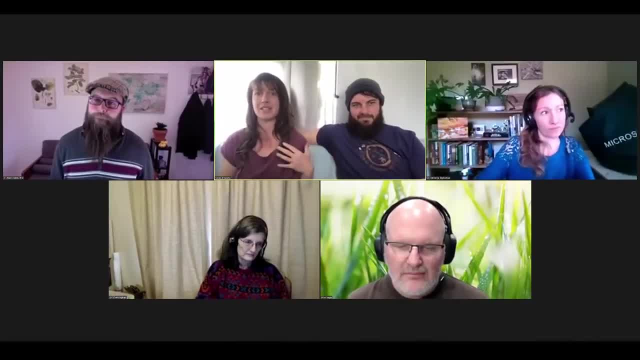 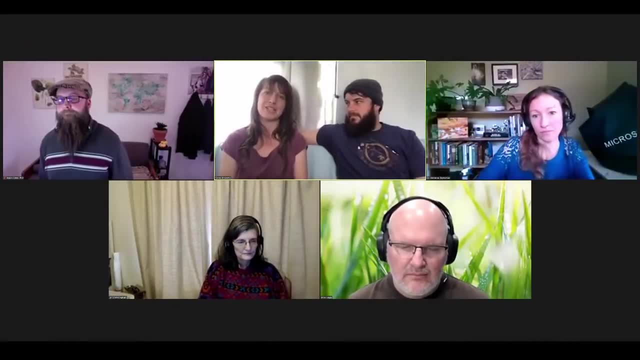 So these natural systems are set up for this. It's not natural to have one organism take over absolutely every inch of space. So nature has set in checks and balances for this, And as long as we're pushing For diversity, then we're going to see that predation happen and we're not going to find this extreme unbalance. 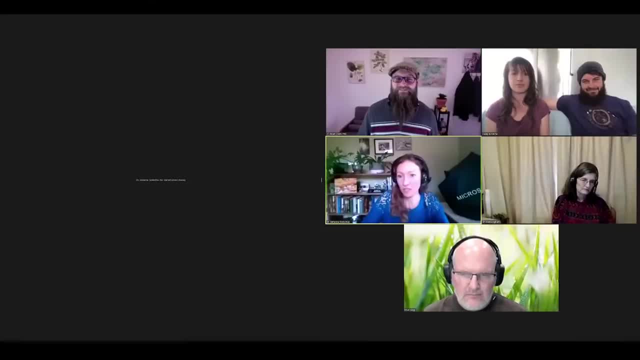 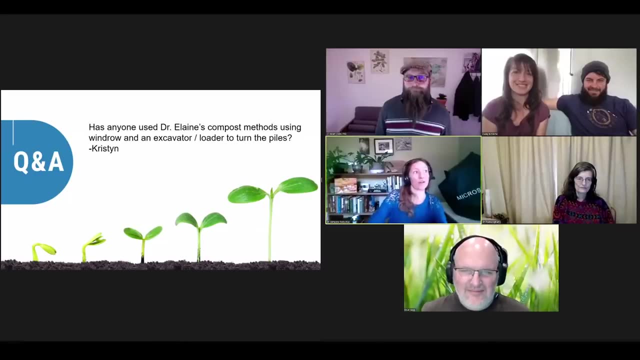 Brilliant. Well, keep yourself off mute, Keisha, because the next question is: has anyone used Dr Elaine's compost methods, using windrow and or or and an excavator or loader to turn the piles? So, if you're going to, we've used the window turners. we've used a few window turners. they work great. 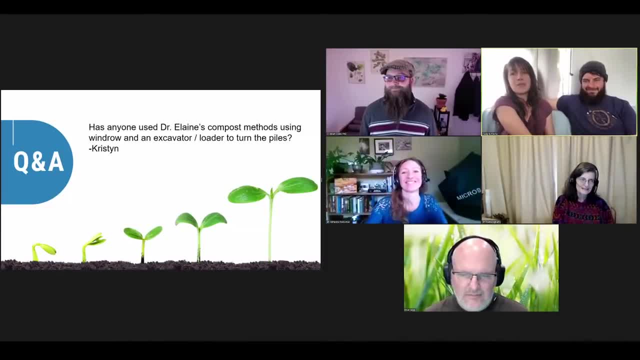 As long as you can Keep them clean. But I will speak to the loader. It takes a great amount of skill. You saw the picture that Brian put together earlier and how you go about the finesse of turning these piles And you'll see, even when you're using a pitchfork and your hands. 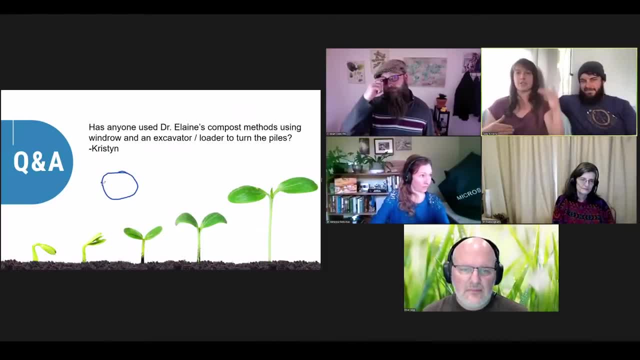 It takes some time and skill to get used to finding where the hot center is, where the top is, where the bottom is. now imagine that you're sitting inside of. you know it's one of those machines that you reach in and grab the toy, The claw. 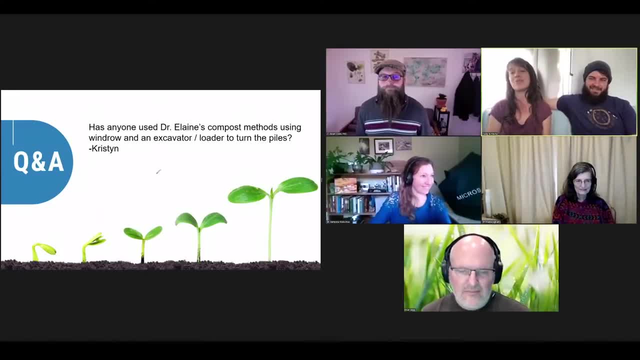 The claw- That's basically what you're offering. The claw- That's basically what you're offering. So you want to have a really, really skilled person on the machine. if they're going to try to do it with a loader, It's really easy to make to make mistakes with the tractor. 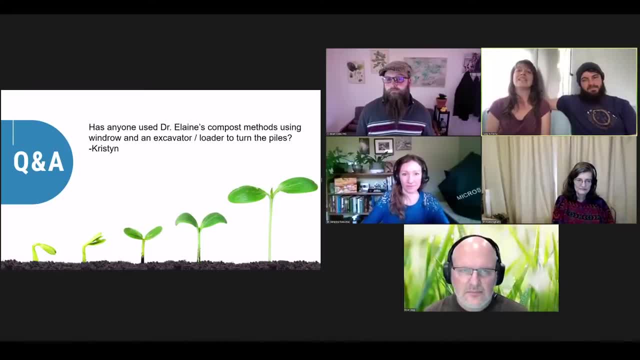 Even the compost piles I've seen, with nice diversity, tend to not get hot all the way through and you're still going to see quite a few. you know: ciliates, sporilla, spirochetes, places where issues come up because the loader excavator is just kind of hard to maneuver. 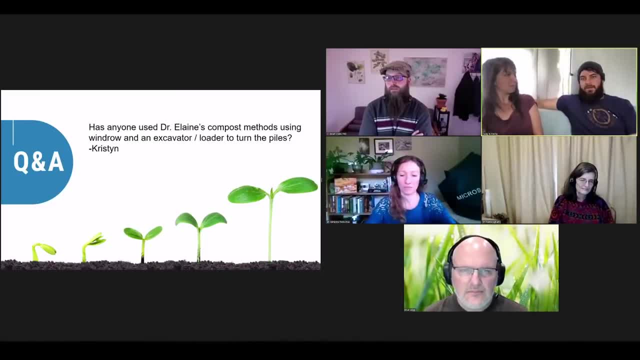 It's also the amount of space required to produce compost with a loader is is five to 10 times More than what you would need with a compost turner, because it leaves the compost in the place that it's in and you just pass right through it. and so, yeah, I would definitely, if you can, if you're thinking about going into larger scale- definitely get some kind of a windrow Turner. it's definitely the way to go. 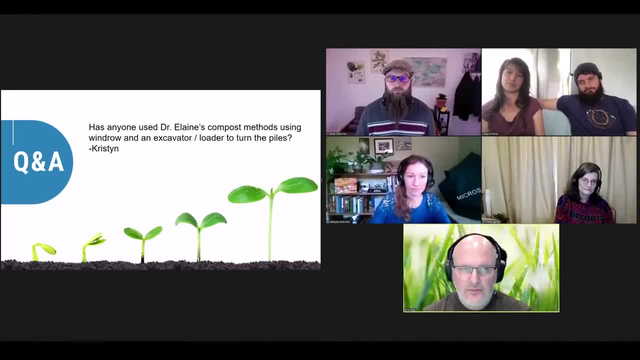 I think, in my personal opinion, it makes superior compost versus using a front loader to do your turning. It just mixes so well and- and that's the thing with like can turn piles Well- a lot of people fail is they don't mix. 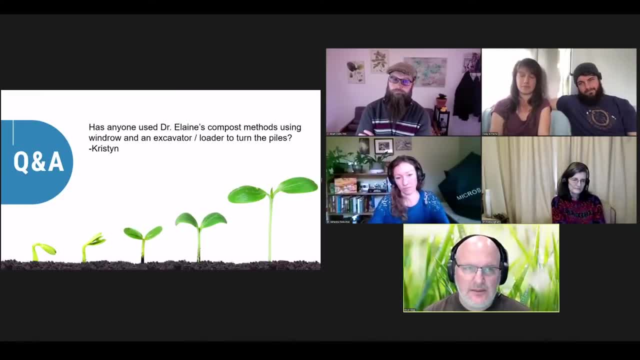 Their materials homogeneously well enough. so you get hot spots and cold spots, you get anaerobic areas. you know that you have to try to deal with. I think the Turner does such a good job of organizing all that material that you get a really consistent temperature throughout in composting. 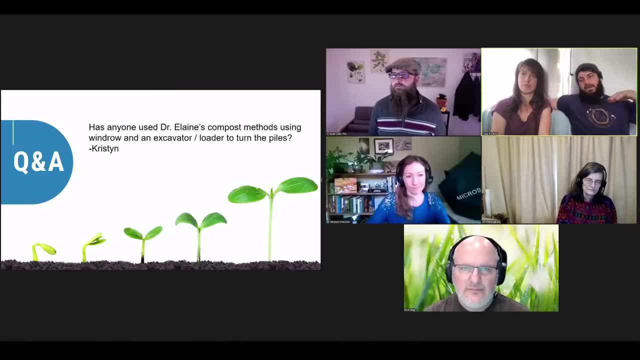 You also don't get all those giant tread pucks either. like when you're driving through compost with those giant tires, you know you're starting to create all these little cakes And those all get mixed back in and tossed into the pile and they're just like these little compressed. 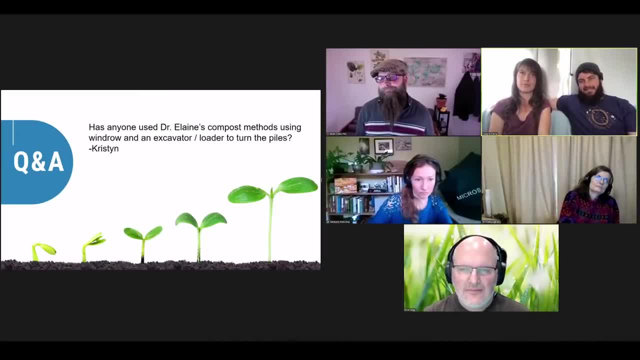 sacks of anaerobic just nasty. Sometimes you would break those open and they'll be full of like maggots and things like that. when we have seen compost coming in from like larger scale facilities that use loaders and excavators for turning, so yeah, it's just something to look out for. 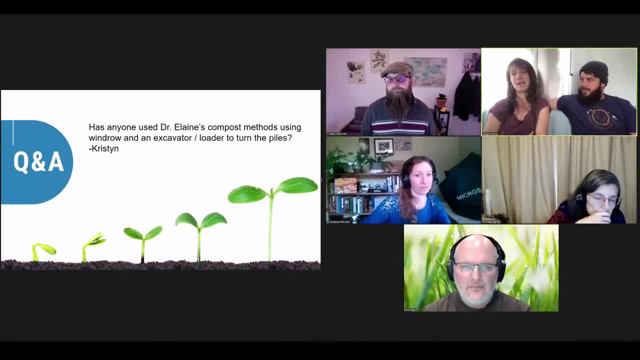 And if you already use a loader, do a smaller pile. don't ever make the mega pile and drive the loader on top of it to scoop it. yeah, So many times I walk it, So Compost is still in. there's 30 tall windrows. you're like, oh, that is not going to be good. 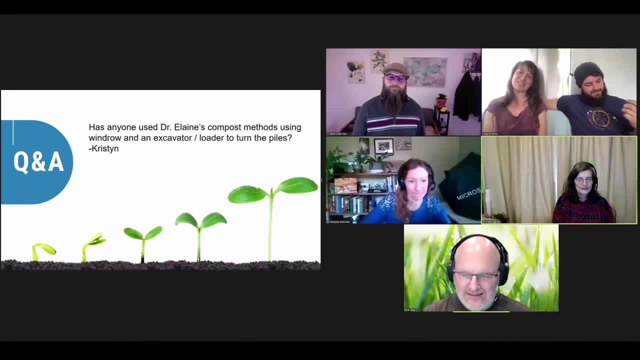 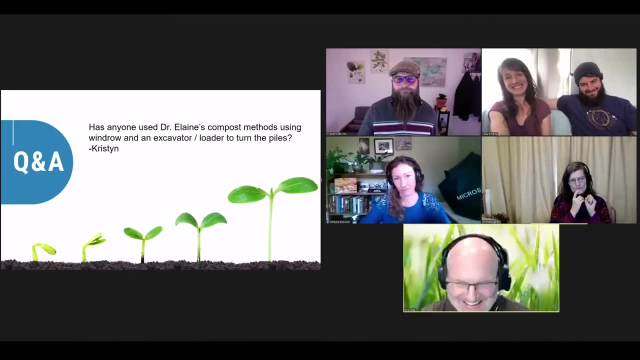 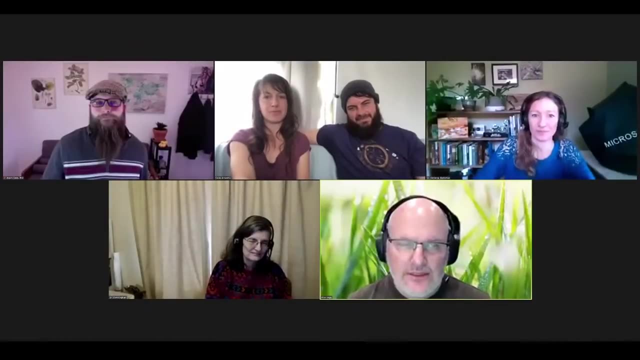 I often One thing: I, Oh, go ahead, Elaine. I often have images of: could I put you in the middle of that pile and ask you if you have enough oxygen, Right? One thing I was gonna mention is that the nice thing about turners is that that you can start with a small scale Turner. That's It's attached to the PTO or hydraulics of your tractor and you know there's the relatively expensive, you know. but for 15,000, $17,000 you can get a decent Turner Where you don't have to spend the quarter million on the really high in turners for large volume input. you know those types of things. so for on farm especially, you know that's some of my farmers or clients look at and say I don't want to do on farm compost because in their mind they're thinking about those big, you know quarter million dollar investments like no, no, we could probably build you some windrows. 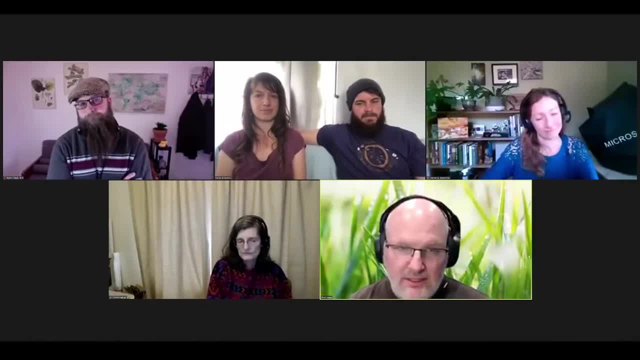 You've already got the tractor, let's get a small scale Turner and start doing that, that method, because you know at some point so your farmers gonna say: I can't make 100 yards or 500 yards of compost by hand turning it, that's just labor, just makes no sense, you know so it's. yeah, the farmer is not the only one who says: when you are working with those larger piles, how do you have to adjust your recipe to match the thermal mass that you're generating? 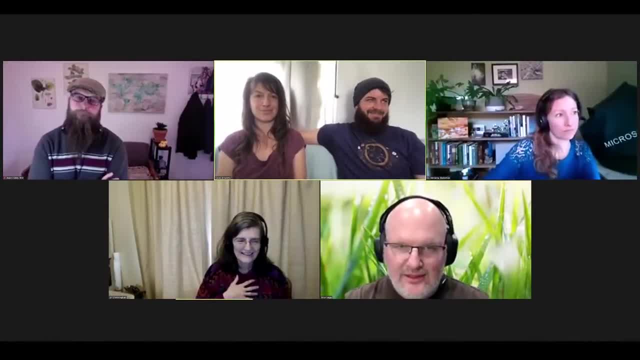 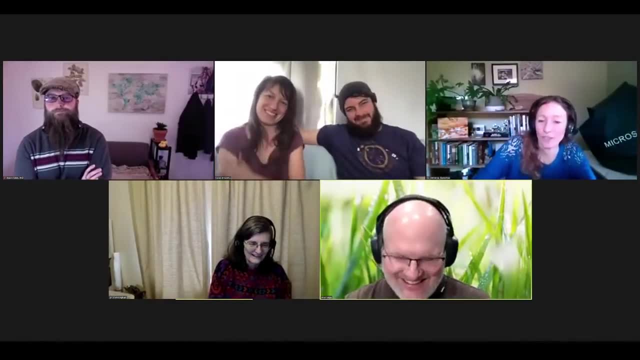 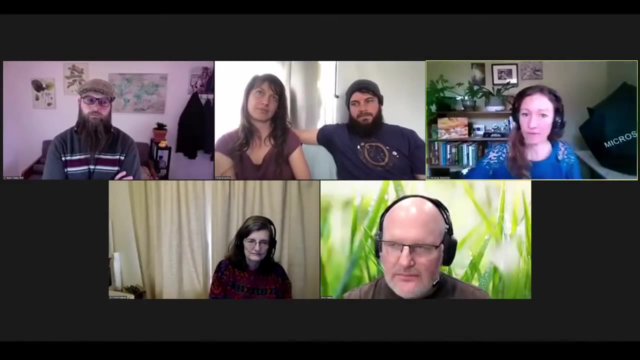 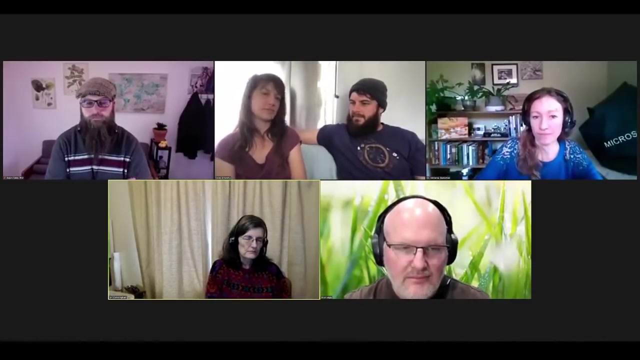 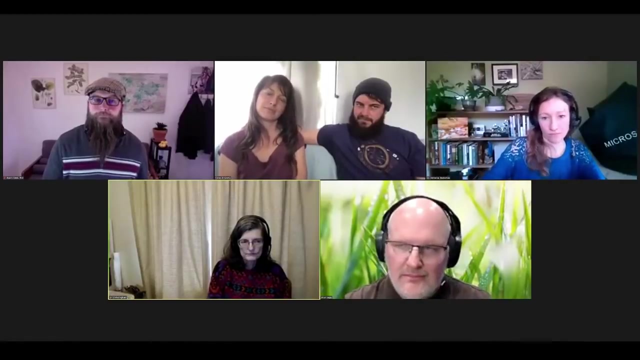 When you are working with those larger piles, how do you have to adjust your recipe to match the thermal mass that you're generating? Not at all. Not at all. It's the same recipe, It's a, you know, just to get the hot high, high enough, temperature long enough, and then turning when it gets to the right temp. you know, hot enough, long enough. It's not no different recipe works just fine for both stat, for both the small piles and the windows. I would say: get, get your small pile game together first before going With the big guys, because if you, if you build, let's say, 500 yards of compost that you're expecting to be biocomplete and you mess up, that recipe has a lot of waste on your hands. 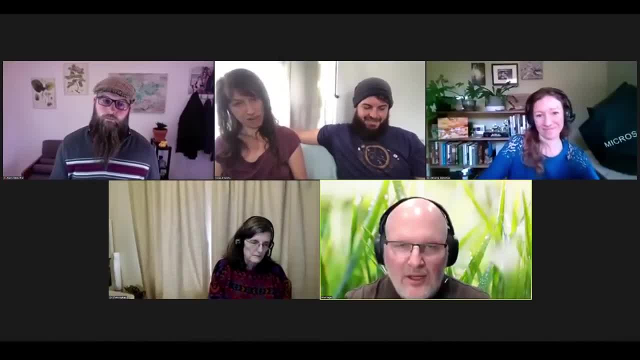 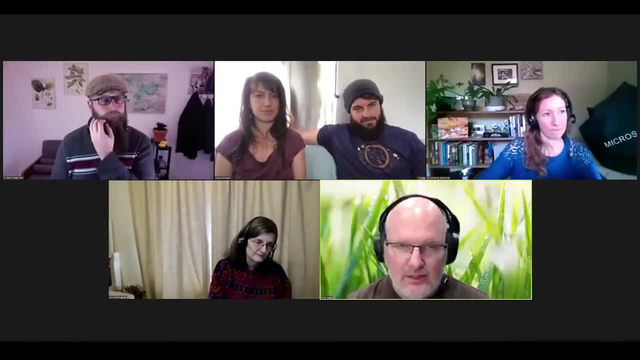 So- and I'd like your point about getting experience- you know I'm working with a really large scale green waste facility that makes you know compost and they now switch to the techniques that links talked about. you know much more on managing your thermophilic piles. 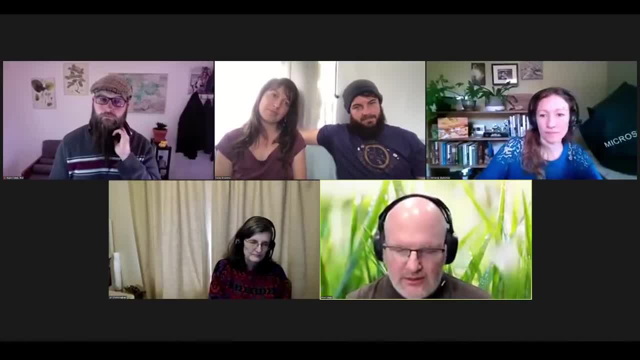 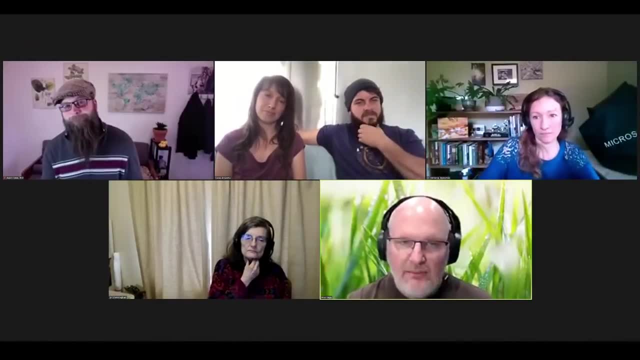 And one of the things that we'll be doing this prototypes. the comment that came back from the composer was like we cannot believe the difference in the material that's coming out of the biologically complete compost versus the compost that they make more of what they call conventionally. 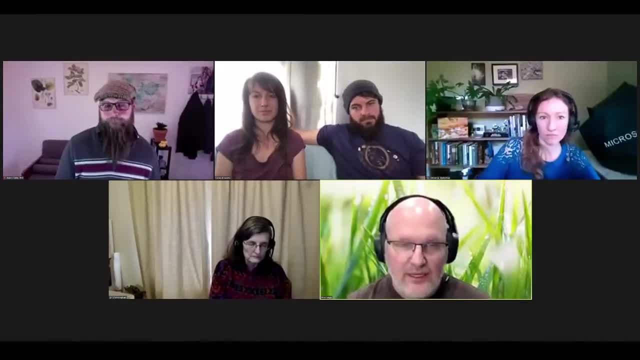 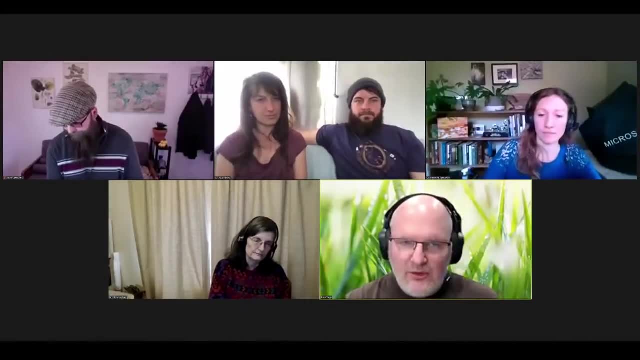 And he says: it smells different, it feels different, it looks different. And now they're getting the intuition by doing those prototypes of: okay, this is what a good compost should really look, smell and feel like. And you know, like he said, start. Small, get an intuition about what good compost really looks like And then when you make the large scale and you have a much better idea if you've been successful or not. We do, I guess we would say we do adjust our recipe for winter and summer, when the outside temperatures- like where we a compost, can get up to like 110 degrees. You don't need as much high nitrogen and those files, because you know you're only. you only need to raise the pile like 60 degrees sometimes. So you know from outside ambient temperature so and And. then in the winter time We'll, you know, just the high nitrogen up just a little bit, or maybe just a little more green and kind of play with those, just to kind of help hold the heat a little bit longer. like, just like a month ago we just got about a foot and a half of snow on our compost. 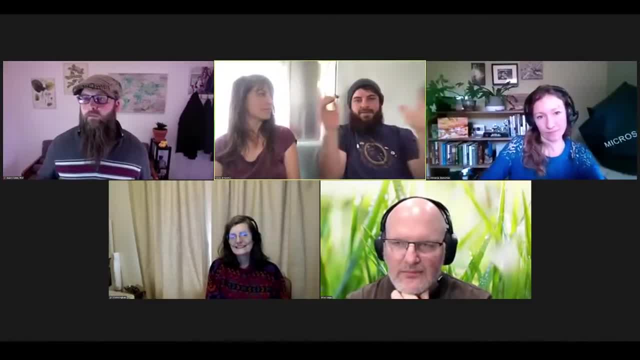 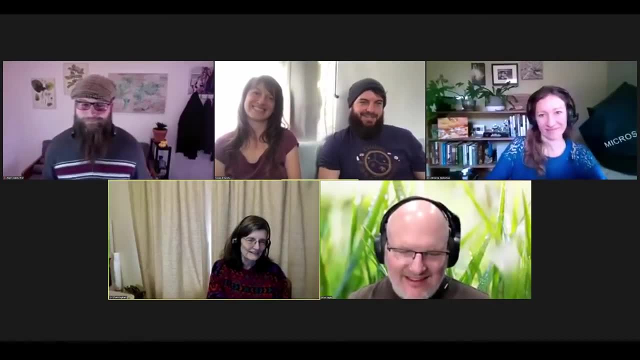 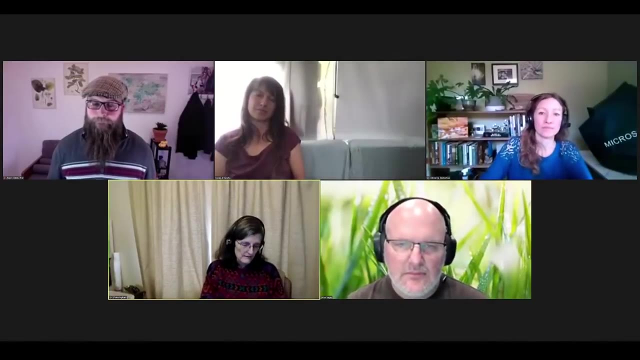 lot And you can see, like the piles, it's like everywhere else there's snow, except for anywhere near and around the pile, But it did cool your piles down significantly. Sure, And the caveats we've talked about with respect to the recipe apply for the big windows as well as for the smaller piles. 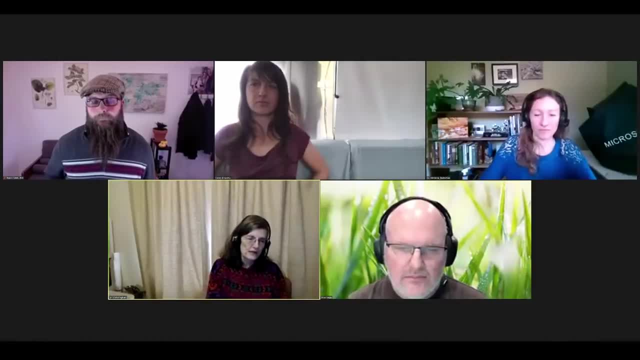 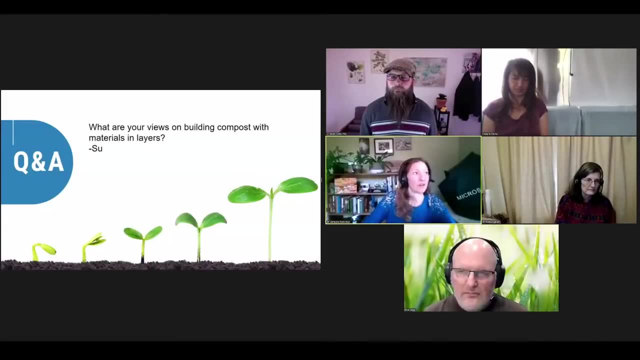 So, yeah, it's the same recipe with all the same caveats- Brilliant. So when you're building that compost pile, What are your views on building compost with materials in layers? It's going to get turned soon enough and then all those layers go away. 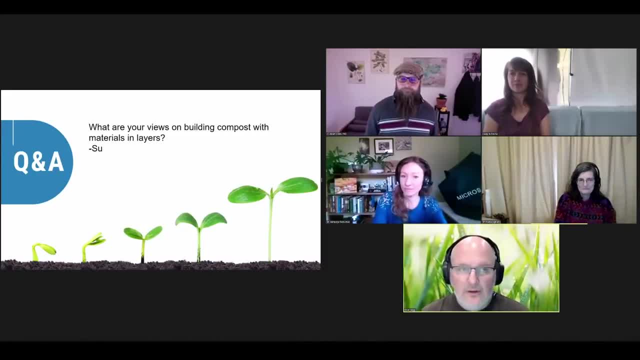 So yeah, I Go ahead. My personal opinion with layers is that the challenge you run into is that sometimes those layers you'll get, like the high nitrogens are, really clump together and then you you'll get a hotspot. you could smell it when you open that pile. 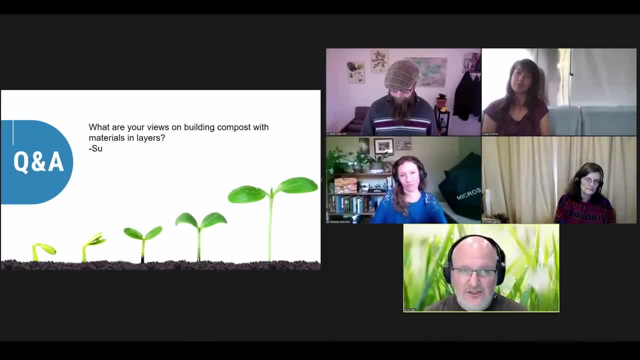 If you're using a compost Turner, Yeah, you start with a layer, but by the time you, like Elaine said, you do that turn. It's too much layer. Yeah, it's too much work to try to keep the layer the same. 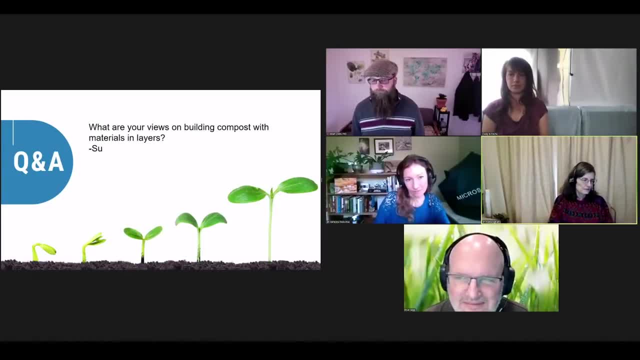 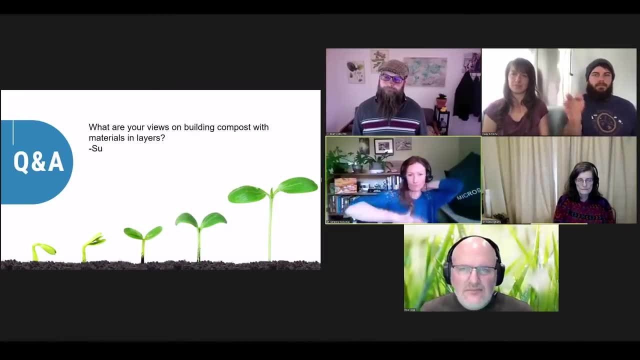 The same width all the way down the pile, or you know the same and different piles. I just say all the way down. Do you mean in a window or in the small window? in the window, Yeah, Yeah, so in a small pile. and I've seen pictures where you do some layers method posting. I think that's what they call. 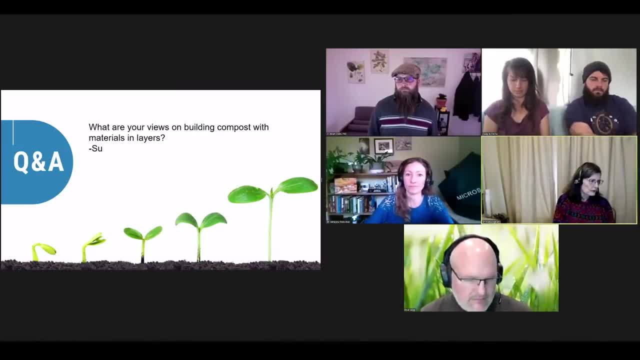 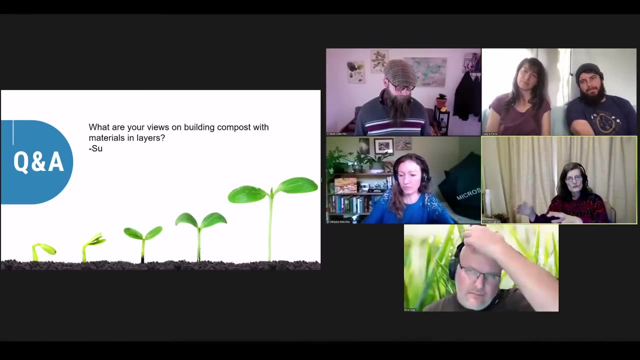 We did. we did a fair amount of work at the Sonoma Place near Sonoma in California, where we very carefully layered everything very carefully, did not smash any of the vegetables or the apples going into the pile, versus we did. We smashed them, cut them up pretty well, then that we turned it into applesauce pretty much and basically didn't make any difference at all. 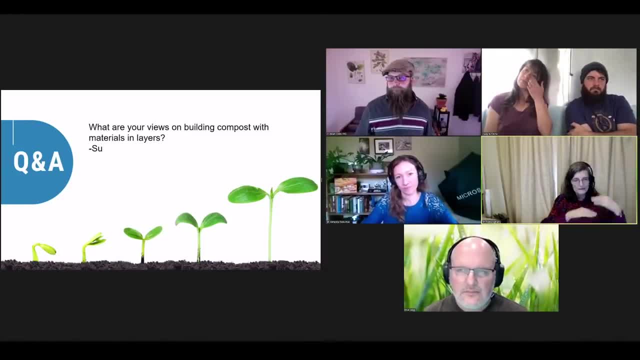 And it's. it's just a lot of work to try to layer something evenly. It's just too much work. you know you're going to be turning it for the first time after you hit 135 for three days or 145 for two or 70. Yeah, so you're going to turn it. it's all going to get mixed together. 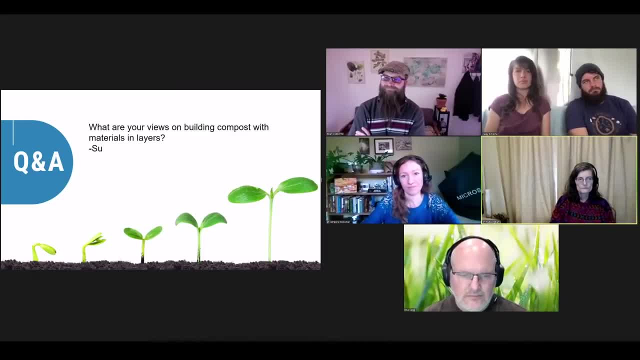 There's no reason to be that anal about it. Now I have seen some situations around layering materials, where somebody is maybe trying to establish a new garden area and they do like a layer- Yeah, Yeah, Yeah, They call it a lasagna bed in there. or sometimes we know who culture and some of the other ideas that are out there, and I've been seeing questions about people saying: can you put trenches in your garden and put materials in there to compost? 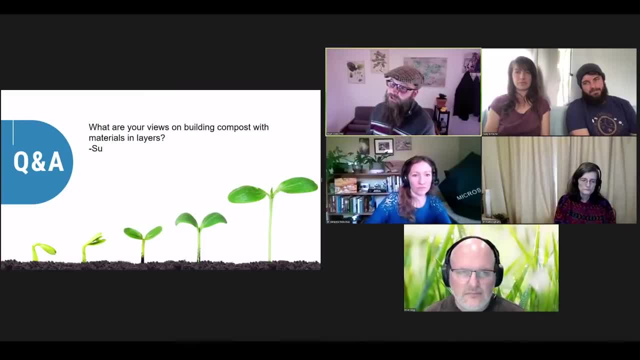 But you have to be really careful about the materials and that you're not leaving, you know, introducing pathogens, weed seeds, all those kinds of things, because you're not going to be getting hot enough in those kinds of systems that can work especially for just a home garden. 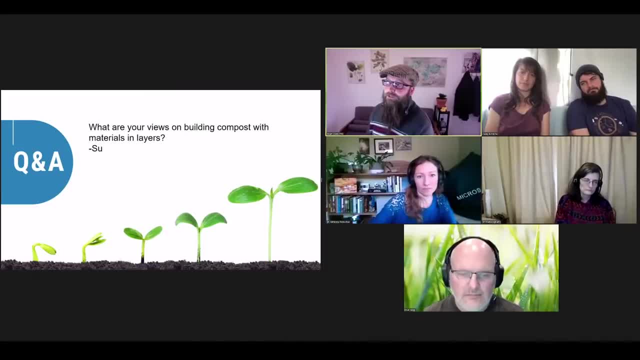 Yeah, Yeah, I don't know. I'm not sure if it's a tree or a garden or whatever, but they're not subject to the same, you know, process of removing seeds and and pathogens and other things. Yeah, what if it starts getting too hot? 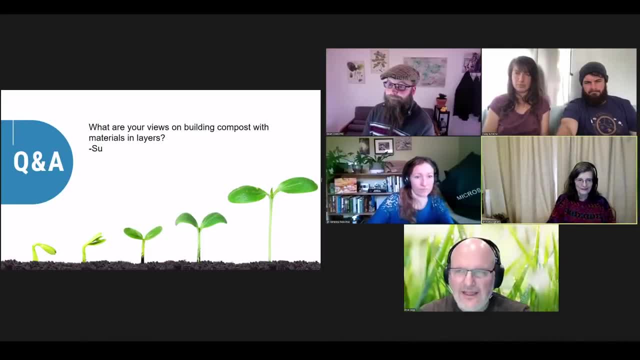 And now you've got like an underground fireplace going for a while. Yeah, kill all the plants you planted. Yeah, at least when, when you're keeping the pile of weeds in place, Yeah, Yeah, Yeah, Yeah, the piles of compost material, uh, where you can see them, you can measure them, you can stick your 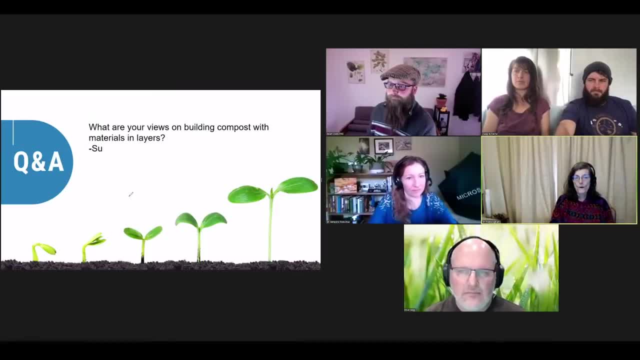 hand into them. there's no question about what's going wrong and it's easily fixed. yeah, i think the the misconception about a lasagna mulching is essentially composting in place, whereas it's better for the plants, you can get it and it goes faster if you pre-compost the materials and then. 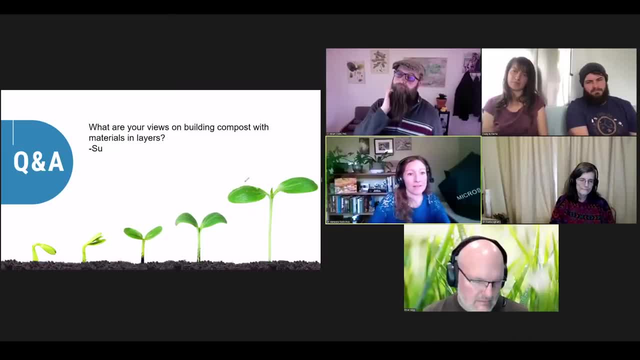 get that out there in the garden beds for plants. but um, i have also found, working with different materials, depending on which kind of high nitrogen, which kind of green, which like, how fresh the greens are, i've had a lot of trouble mixing together a lot of like fresh, like greens. they 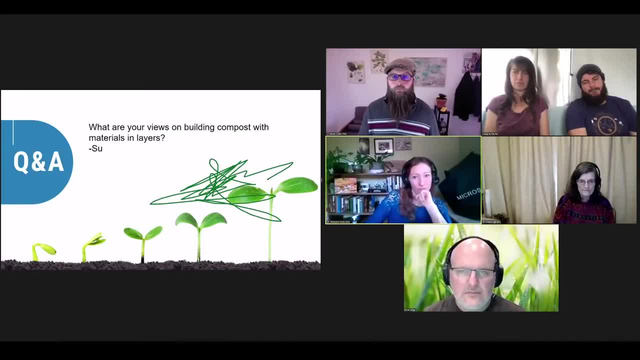 just like you know, mat together. so what i've- i've tried out a couple times- is i'll mix my, my woody materials, my bark chips. i'll like mix them on a tarp in the right ratio with high nitrogen. i'll like sprinkle in my little high nitrogen and i'll make a lasagna of sorts. 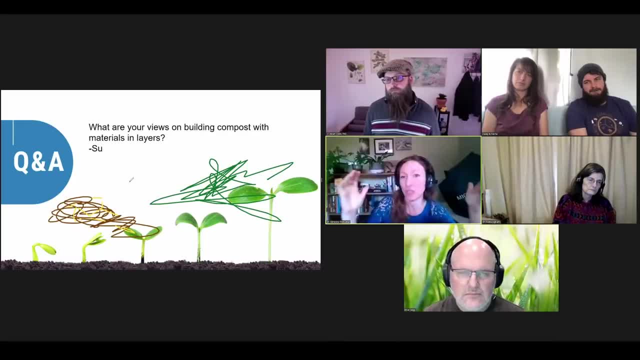 where i'll make a like one, one to maybe two inch layer of this, you know, basically six to one woody to high nitrogen material as my like meat sauce and then just lay across like a mat of my fresh green as my noodles, um, and as long as everything touches everything else i've had. 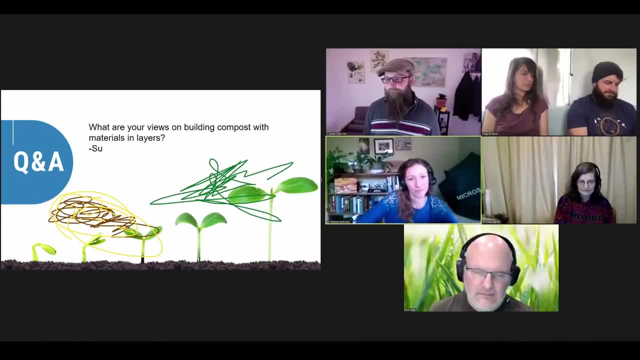 success because in the second turn it all gets mixed together. so, depending on the starting materials you're working with, do what's easiest right. if you get coffee grounds wet before you mix them into a pile, you're gonna have a film like a whole clump of coffee grounds, whereas if you sprinkle them in dry, they'll pick up the moisture, it'll be okay. 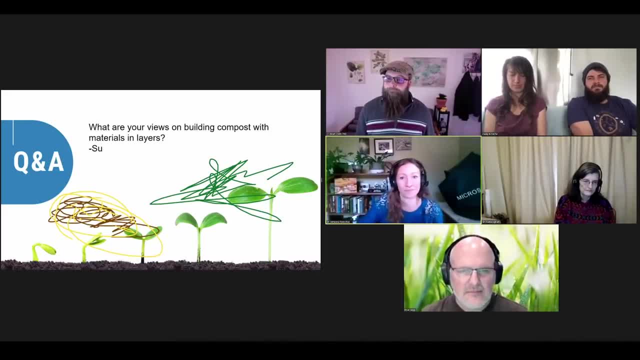 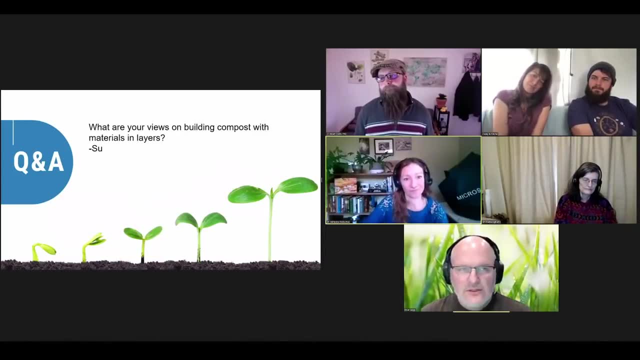 you don't have to soak, pre-soak your coffee grounds, any other starting material tricks that you all work with. well, i just wanted to circle back on something adam talked about in hula culture. i've used hula culture quite successfully- my guards and so forth- but you're being very 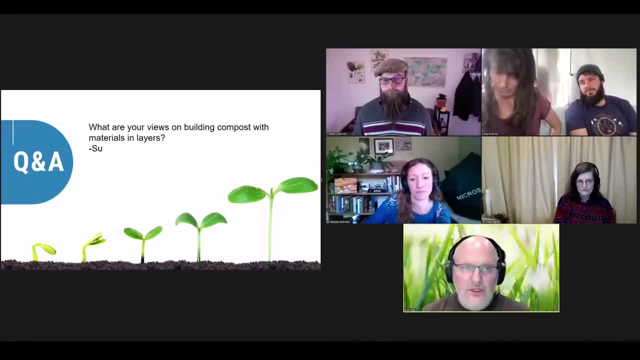 thoughtful about the wood that you're using. you want to use very well rotted wood to start with, when you're doing like a hugel trench and putting that into your gardens, um you know. so, yeah, you can be very successful, but you just have to be very thoughtful about the materials. i i never in my 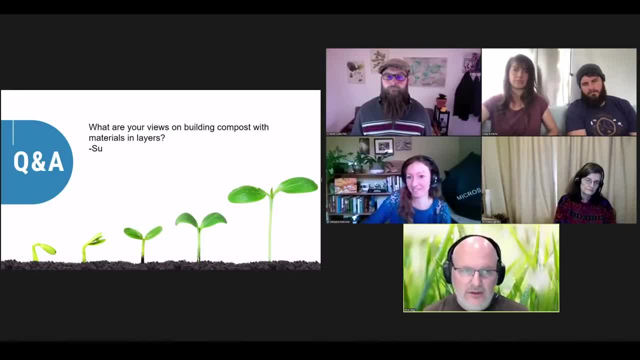 hugel trenches used fresh cut wood. you know i wouldn't go out there and get fresh cut cedar, redwood or eucalyptus and say, hey, put that my hugel trench, i'm gonna have success, you won't. um, you need to be. you know sure the kind of materials that you're using. 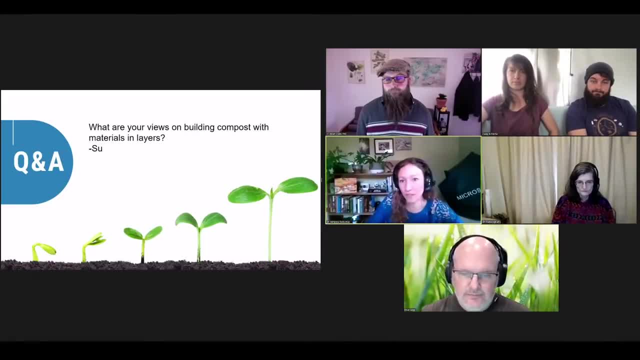 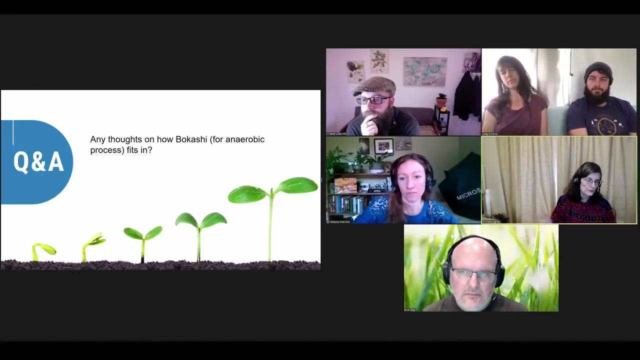 brilliant. um. speaking of composting methods, any thoughts on how bokashi or other anaerobic based composting methods? how do those methods fit into this whole process? silage, bokashi, etc. well, you make silage in order to preserve um food uh through into the winter time for your 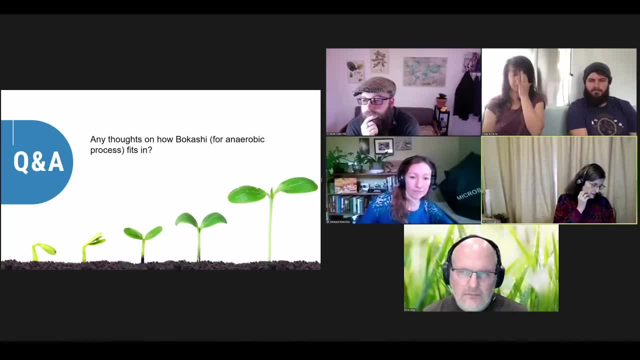 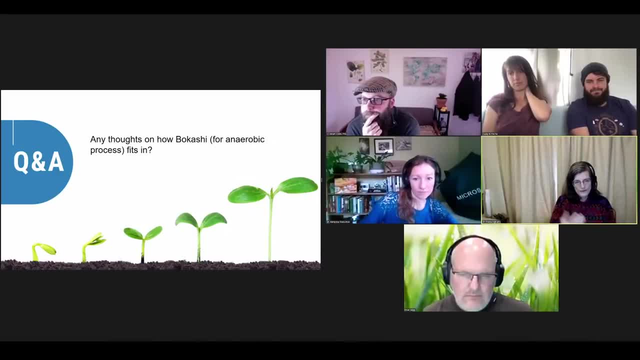 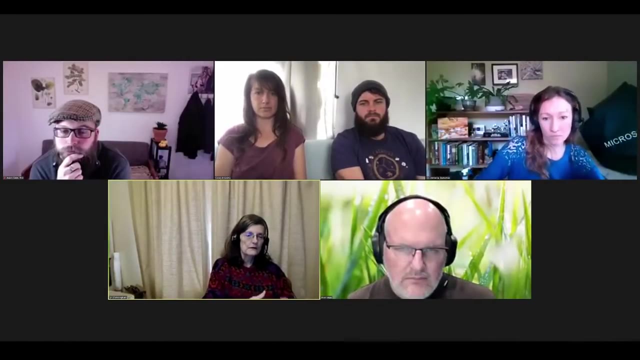 so it's a preservative process. um bokashi, you know it's uh taking materials that perhaps you you have a over on a large amount of cabbage and you're trying to figure out what to do with the excess. okay, preserve it, stick it in in a jug into the ground with water salt typically in it to. 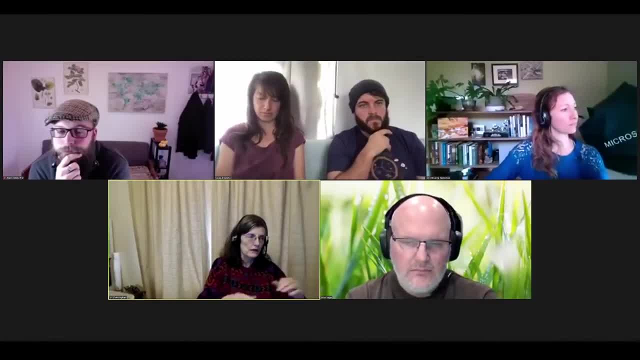 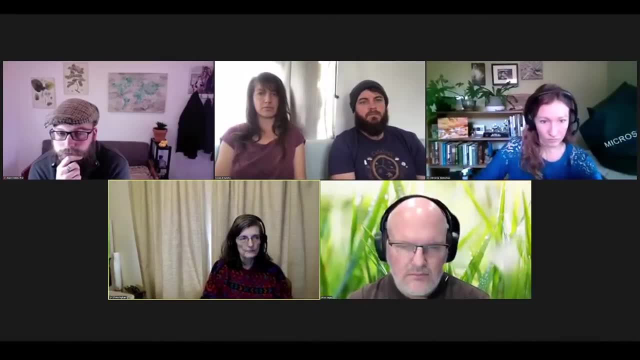 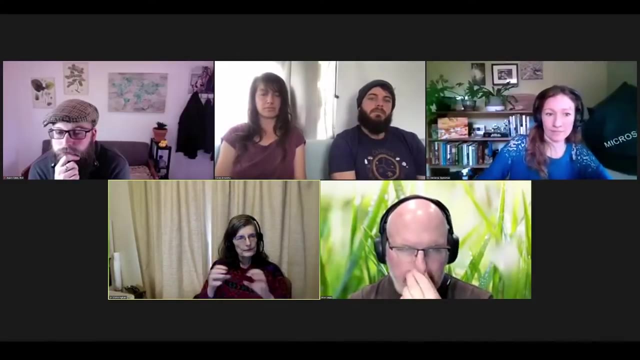 discourage diabetic pathogens and you seal the- the juicer that's researching that the jug- and you bury it for you know, a couple months. it's well preserved, works, works fine. now is it a good idea to put it on your plants? quite often, if you put it on the leaves, you're just going to. 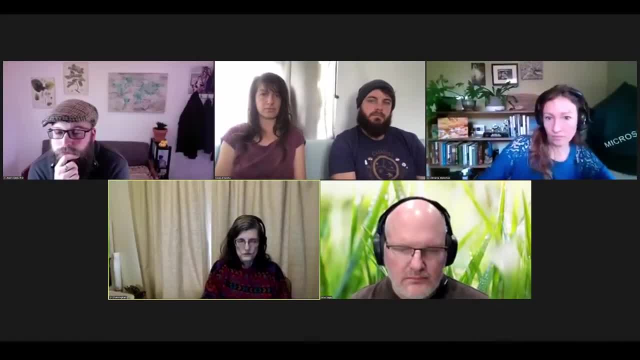 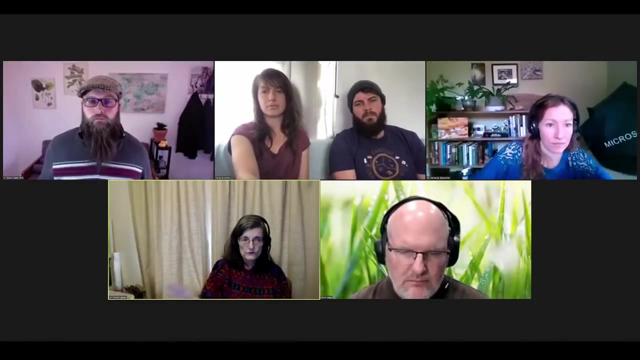 cause all of those leaves to curl up, and usually you lose your plant. if you apply the bakashi around the root system, however, you might be able- or even above ground, if you spritzed it on places where you have disease causing organisms, you can knock those disease causing organisms way back. because all of those materials that are made under the anaerobic conditions are fairly well, they're preservatives and all of a sudden all your disease causing organisms are preserved. well, they're not coming back. so you can have some good effects, but long term you're going to want to get the really beneficial organisms back into that system immediately after the bakashi does its job. so you've got to replenish the bakashi, the um, at the organic acids that are in that mix, the um. you know the loss of the nitrogen, the loss of the sulfur, because under anaerobic conditions you lose those things to. 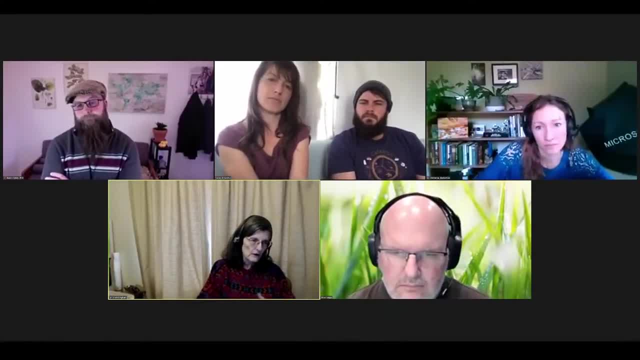 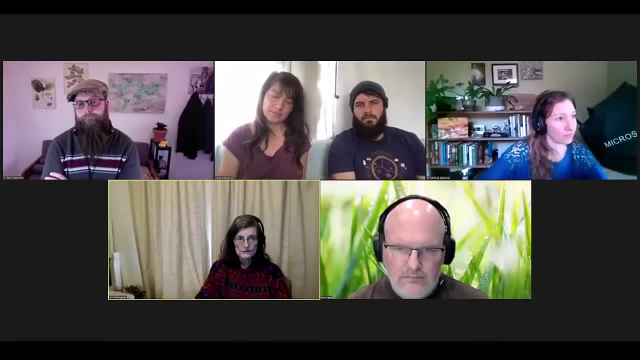 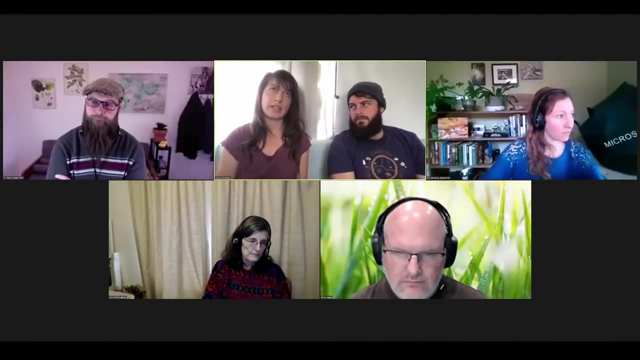 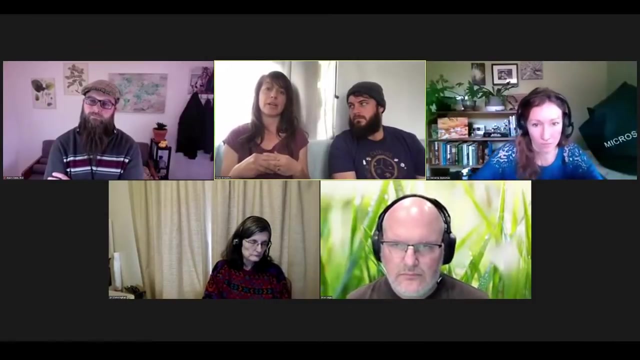 the atmosphere because they turn into gas, you're causing an imbalance in the soil, and so you're taking this into consideration. so that's why we're doing a lot of studies. we've seen it time and time again when we've tried to use brewer's waste as our main source. 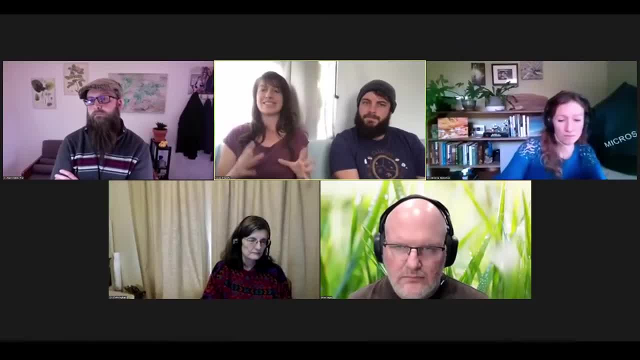 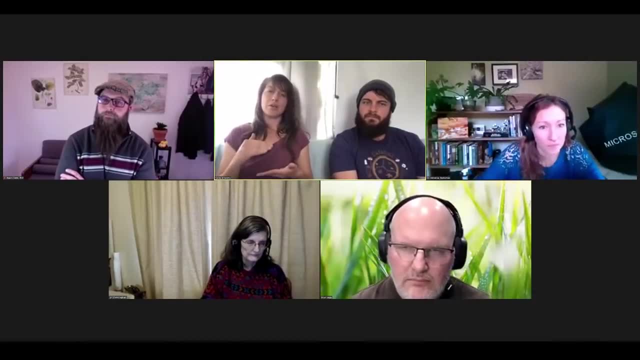 of high nitrogen, that the fungal content, just that the piles just don't look texturally or under the microscope exactly the way that we would like them to. but as long as we use it in small amounts- and I don't have an exact percentage for you- it's just not putting too much anaerobic waste. 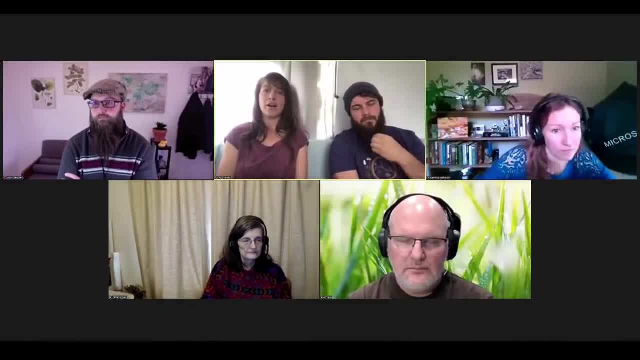 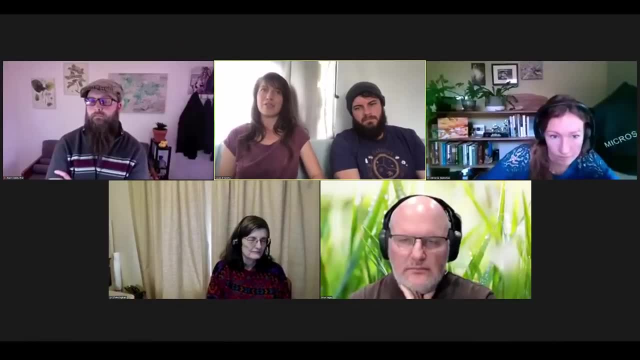 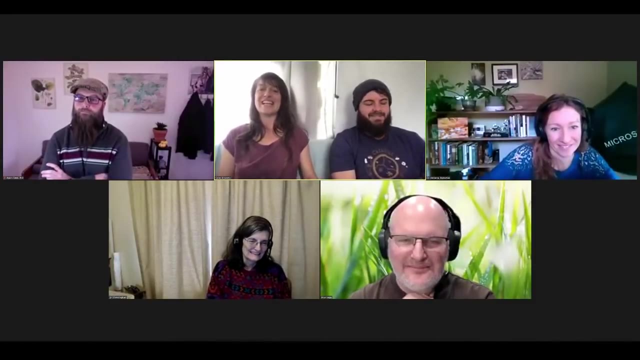 into you know a proposed aerobic pile. you kind of see as you as you, you learn as you go and you use these things. I've never had a chance to use silage before, but I've heard some horror stories from fellow composters in the food web school. yeah, that if you use it as your only green material. 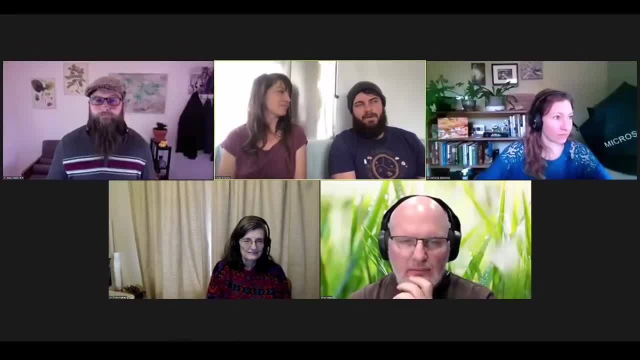 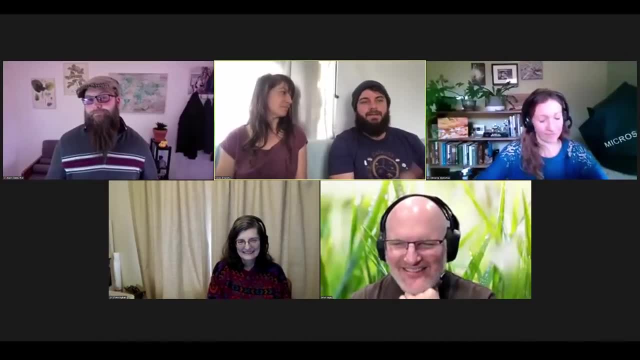 you're going to have some problems. yeah, I mean, I think, because she's throwing which is, oh, go ahead, Brian, no, go ahead, no, no you. I was going to say I think she's great for growing, like facultative anaerobes, these and these microbes that they do well they're. 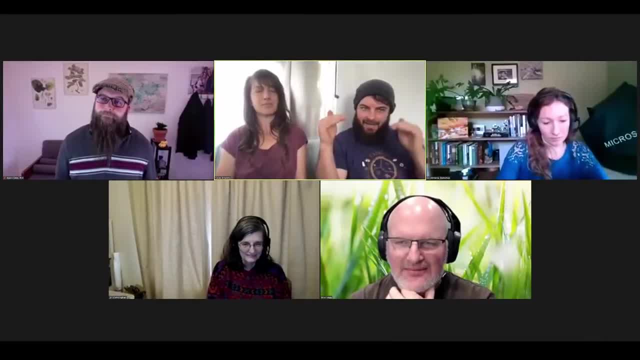 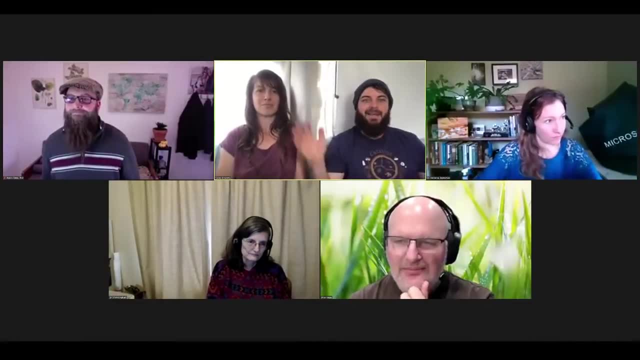 not technically anaerobic or not technically aerobic. they kind of hang out right on that threshold of where things are starting to go bad, and so I think they're great for like your paratroopers going in there and like putting them into an already anaerobic environment. they're. 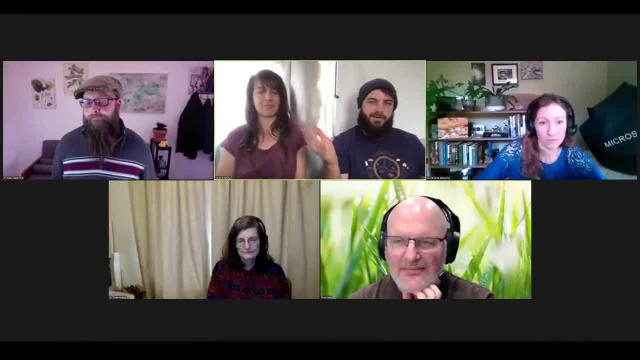 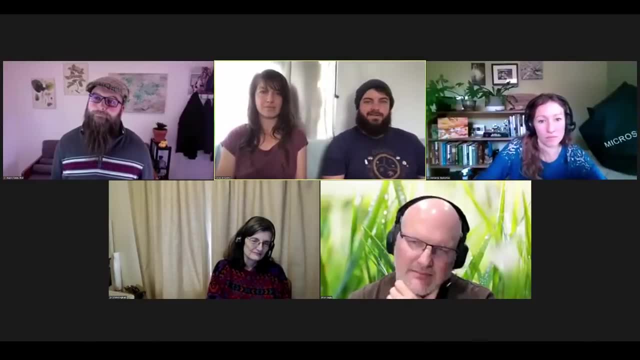 gonna start shifting the tide back to aerobic and then you come back behind that and start applying aerobic microbes over the top of it. so I think they're kind of like your, your first responders in a way. you know what I mean. I heard you bring in these bokashi, that's. it's always how I kind of 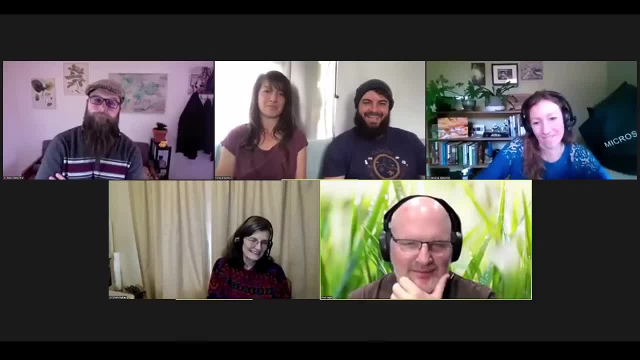 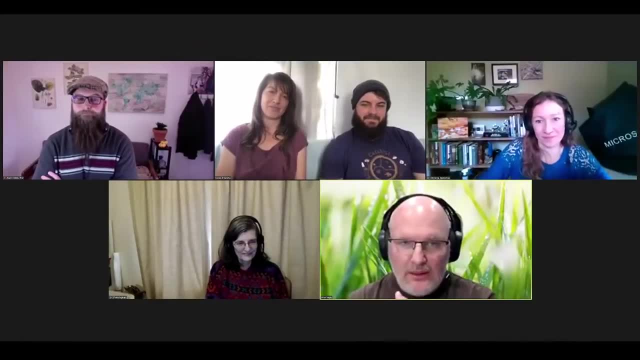 see it anyway. I see a cartoon. I was going to jump back to a point that Kishi was talking about. you know, using something in large quantity and I think that speaks to you know some of the best complex I've ever seen. it came from a very diverse set of starting materials that you use a lot of different. 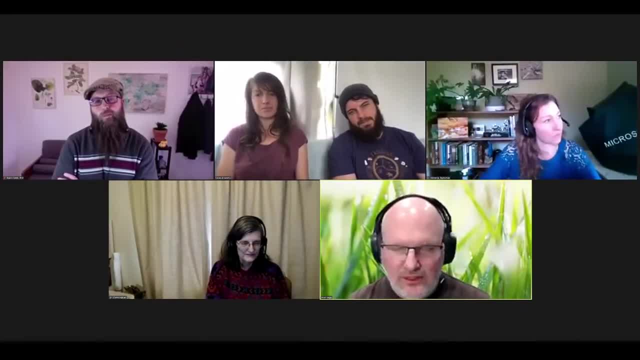 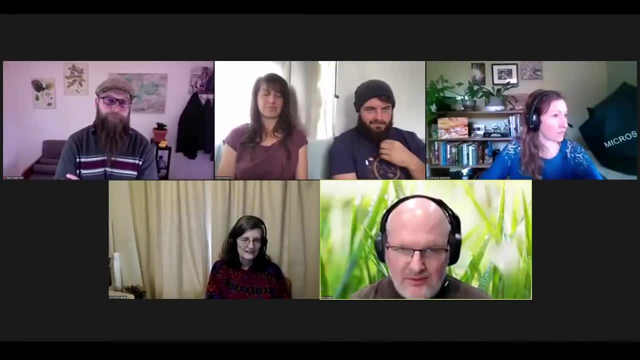 types of inputs. there's a lot of different food sources that are different types of microorganisms, you know, and some of the worst compost I've ever seen has been like a two input compost. it was cow manure and bedding, all right. well, there's a very small set of food sources that are going 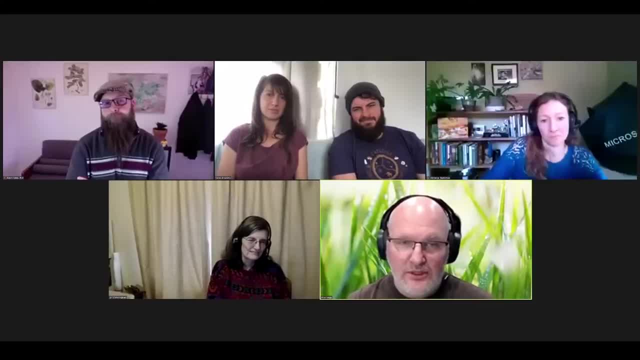 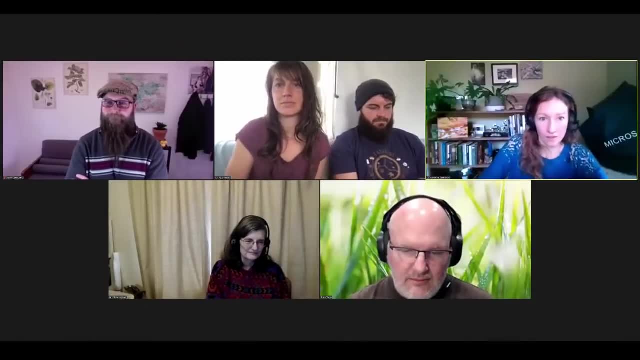 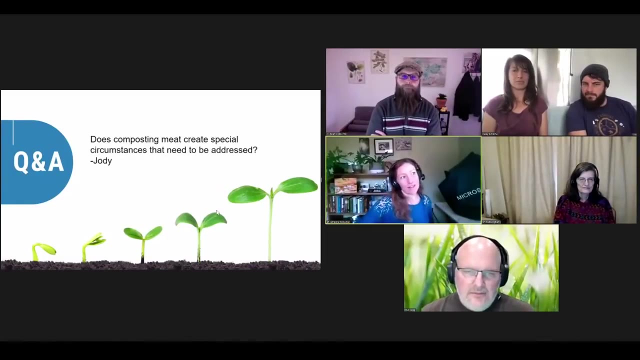 to be available for the microorganisms that are in there. so diversity of inputs typically equals diversity, microorganisms and good compost. speaking of diversity of inputs, does composting meat create special circumstances that need to be addressed? excellent question, Jodi. you've got to break up that meat into a real small. that might be one time. 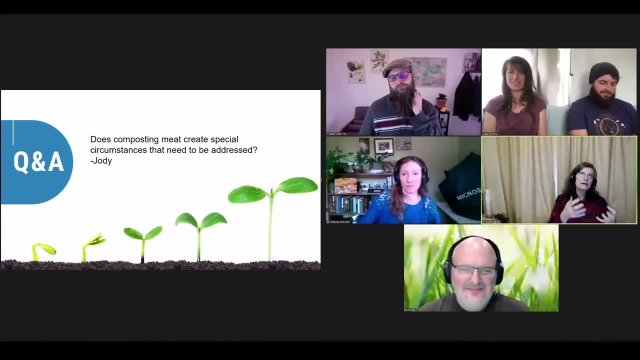 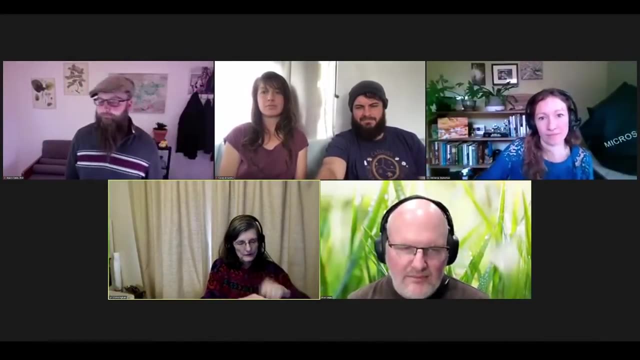 where I get the blender going, because the meat is such a high nitrogen source that it's almost impossible to prevent the microorganisms from growing so rapidly on that meat that it goes anaerobic. it's just really hard. so, you know, chop up those uh the meat into really, really small. 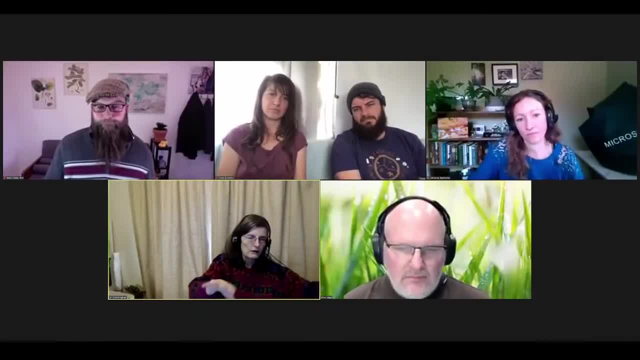 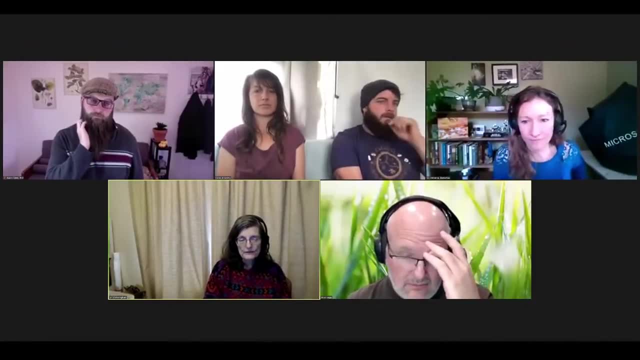 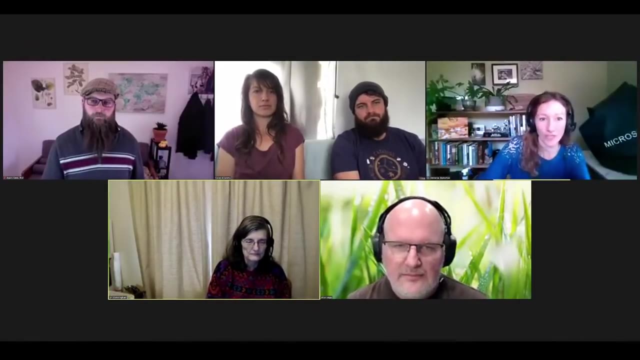 bits and pieces, mix them up and then you're good to go. so I think that's a really good question, Jodi, and I'm hoping that's something to keep in mind, because that's another question I'm looking to answer as well. but, like at any given point, I think, composting, I think, is just so. 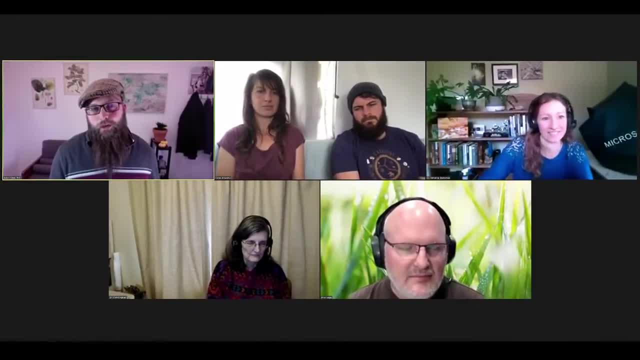 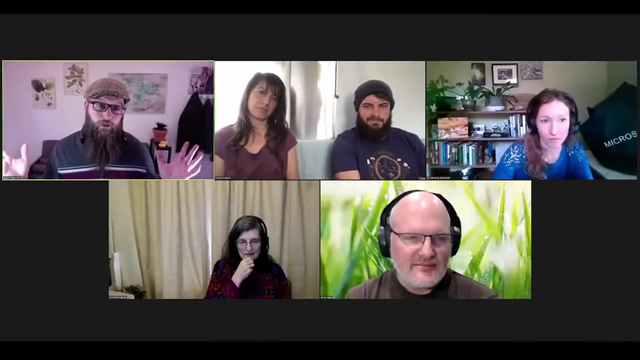 important because it makes it well with all of the at the beginning of the composting process, so it's more or less evenly distributed through the pile and don't use too much of a big compost pile. right, they could. they even the bones, even the teeth could eventually disappear. the hooves, the everything. yeah it. just because when you get in an anaerobic condition, the organic acids are so strong that you know they they've got a ph that's very, very low and they just disintegrate anything. so okay, you've got a. wherever you're, you put your goat in you're, you've got kind. 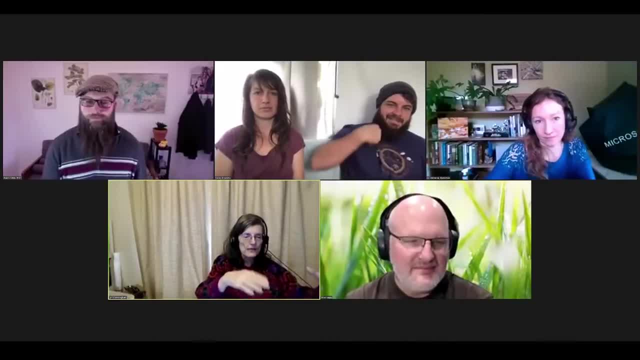 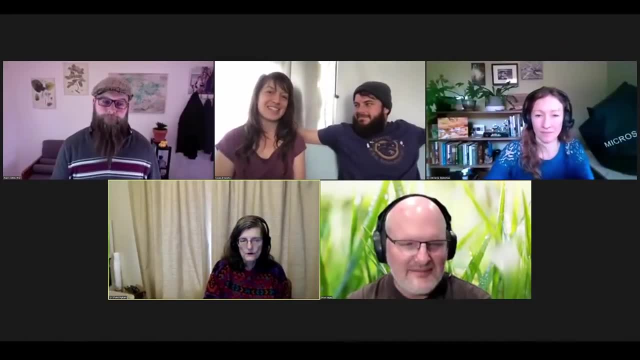 of an anaerobic spot. wait until the goat's actually completely decomposed and now run your windrow turner through the system. don't- if you, if you're doing this with a bunch of shovels- don't start until you absolutely know that that goat is completely gone. and how do you know? 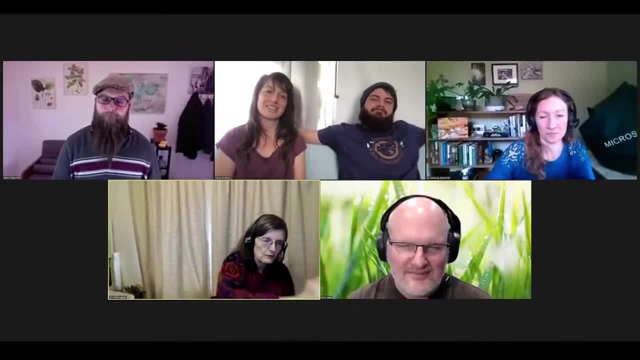 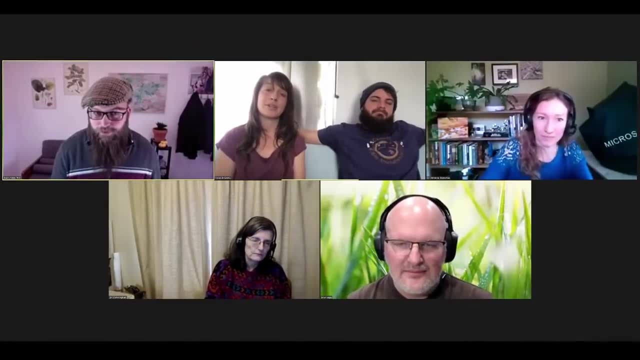 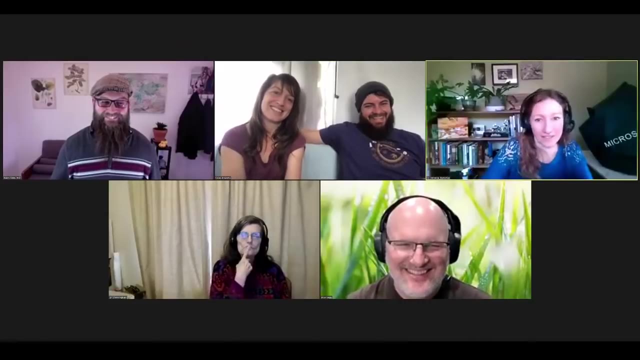 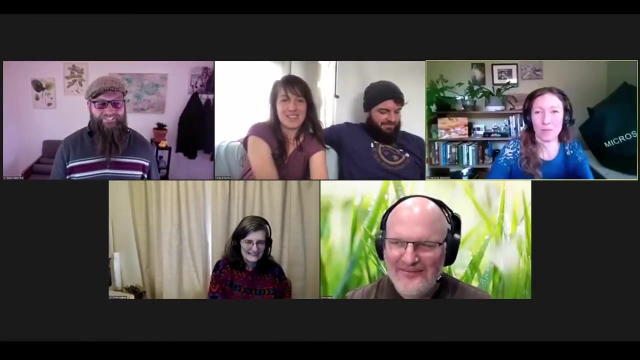 thermometer in the pile, check everywhere where that animal was and make sure that temperature is right down to normal levels. you, it was recommended to use goat compost on trees and not leafy green vegetables- excellent point. i wonder why i also have a side experiment in my yard where i'm doing a static pile of bark chips in the 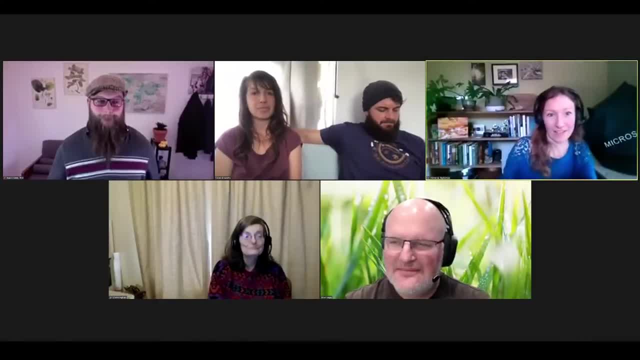 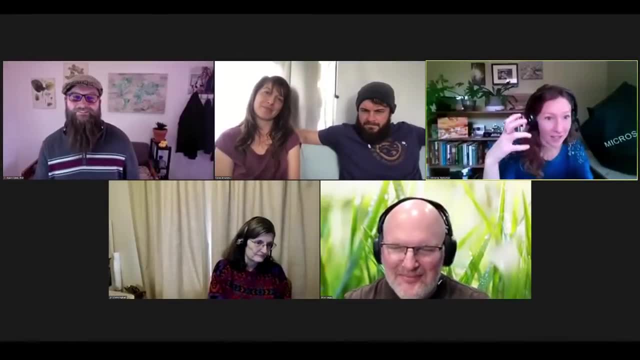 backyard for the dog. so i'm mixing a woody to dog poop, um, static pile. definitely not going to put that on the leafy greens, but curious to see how, after long enough in a static pile and then through my thermophilic, and then through my worms, we'll see what we can make. 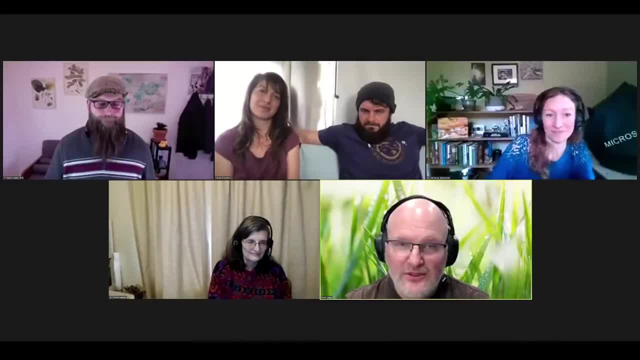 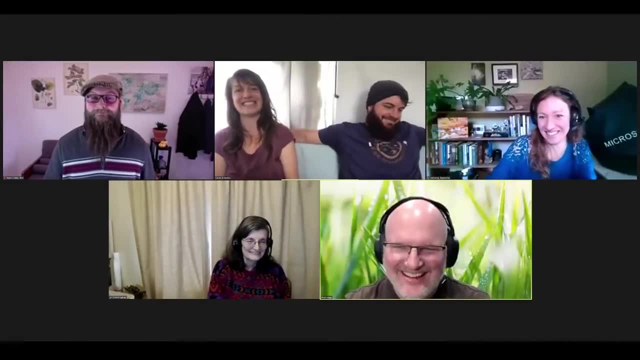 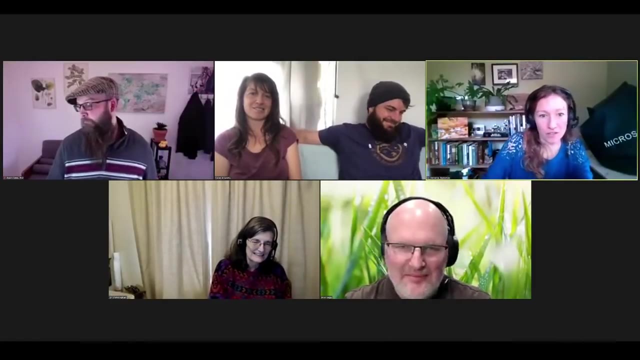 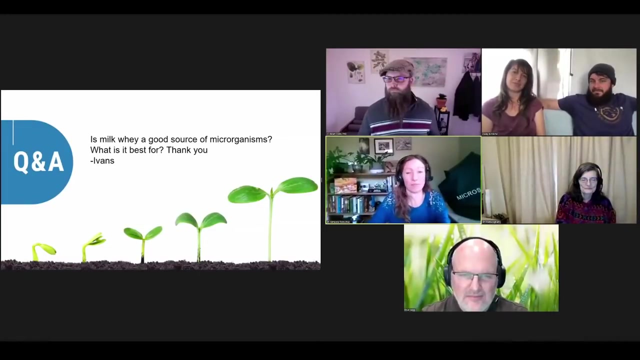 well, there's a whole new industry too, of human composting. human composting has to come. anybody out there? all right. anything else on meat, or shall we move on to milk milk? is milkway a good source of microorganisms? what is it best for faculty of anaerobes? yeah, lots of lactobacillus. and you know they, as um brian was talking about you know. they're. they're good as kind of a um, an in-between when something's gotten really anaerobic. now you're going to move into the- uh um, lactobacillus into the aero. so sorry, it was casey that said that. yeah, i'm sorry, brilliant. 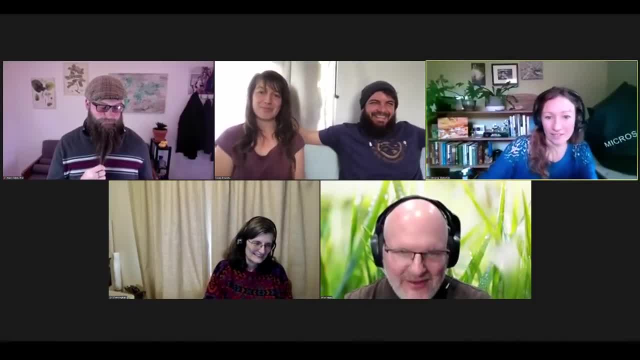 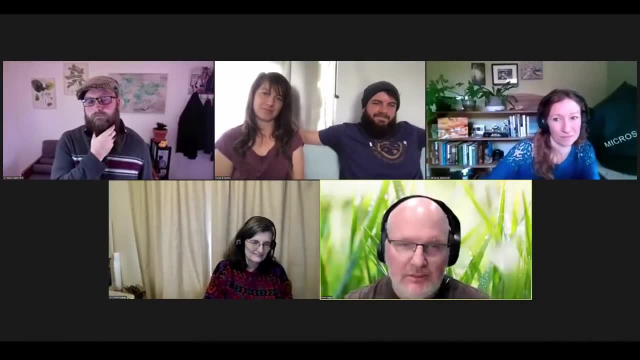 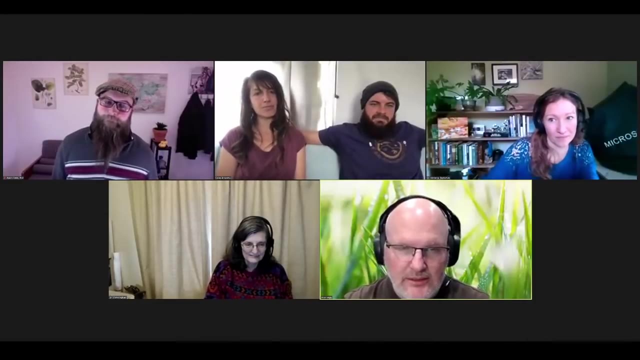 great, i've just decided on. on way, you know, before i actually, you know, knew about elaine's uh course and learned about the soil food web, i saw a video of a guy putting out way from raw milk on his squash plants and cucumber plants and melon plants to suppress powdery mildew and i was like i have. powdery mildew on my grapes and my squash and and i had access to raw milk and and we made some some yogurt and i had the way and i sprayed it on my grapes and my squashes and my cucumbers and i suppressed powdery mildew pretty good- not as good as i can do when i make my compost teas now in the 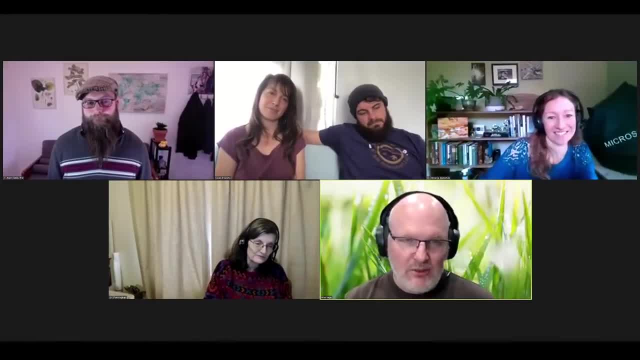 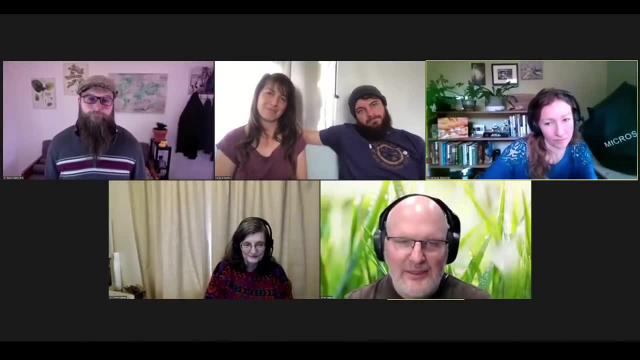 soil food web. i could, you know, completely suppress it, but i was just blown away. it was one of those steps that led me into. i need to know more about this. i need to understand more about this whole, you know, biological aspect of it and it was just kind of a cool thing. i was like, wow. 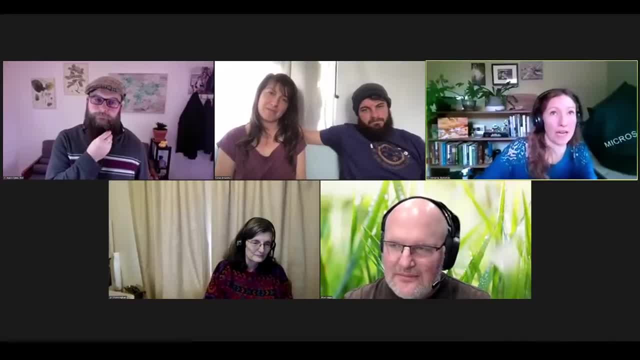 and that is a beautiful role of that anaerobic metabolism, right? so both the lactobacillus as well as some of that focaccia can be used for, um, just immediate controlling an outbreak in the moment. so it might not be the best long-term solution, like you're saying, brian, but 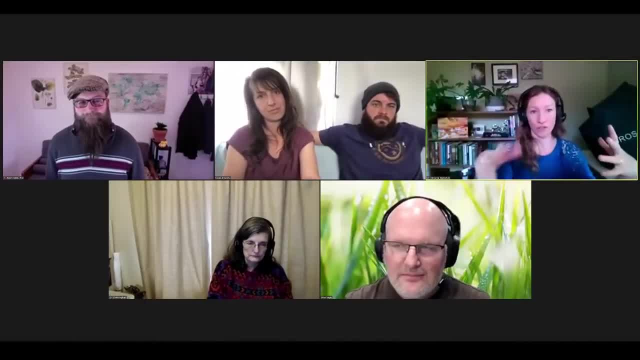 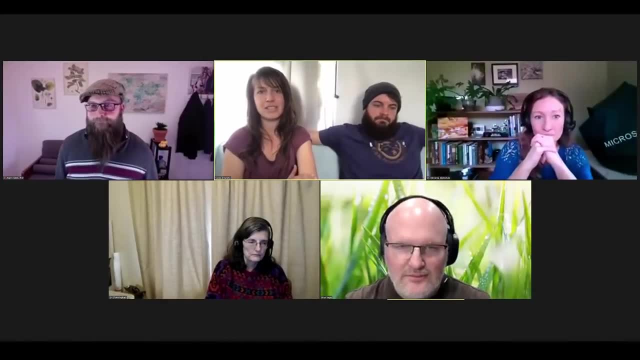 the or the acids that are being produced are great for, just like you know, arresting the chaos and stopping it from continuing. you can imagine those facultative anaerobes probably have a hard time to continue their life on leaf surface. there's just too much too much oxygen there for. 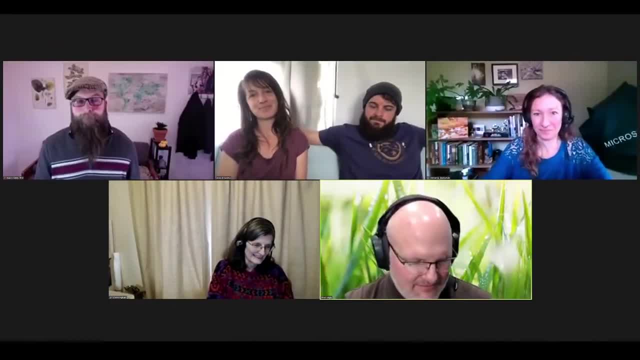 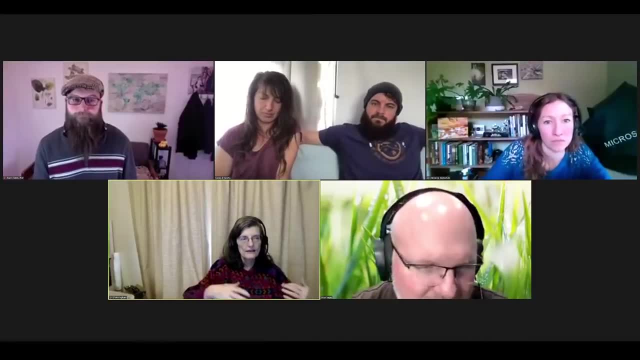 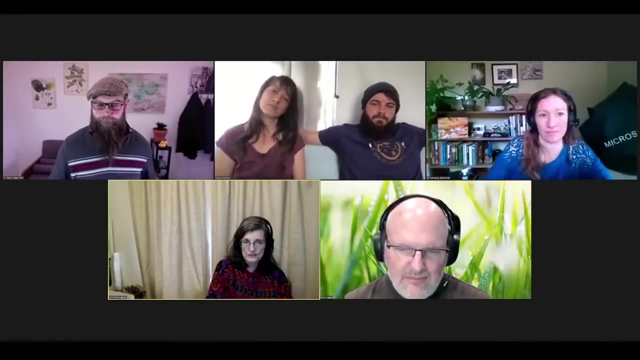 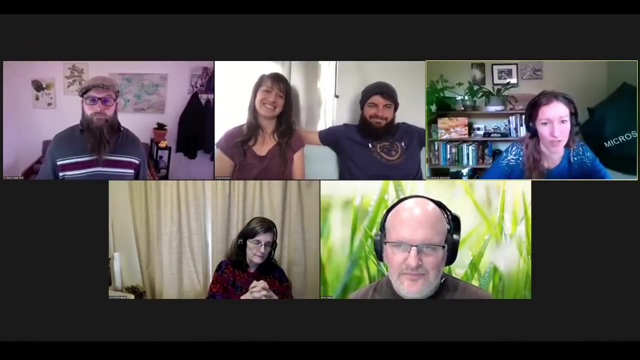 aerobic. so you apply the kashi and it has its direct, immediate effect. and then, because of too much oxygen, those facultative anaerobes have to go to sleep because they're being out competed by the aerobic organisms. hey, that's perfect. there we go. that's the full story. thank you for putting. 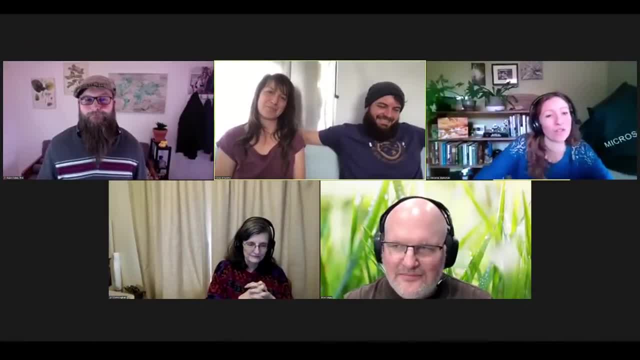 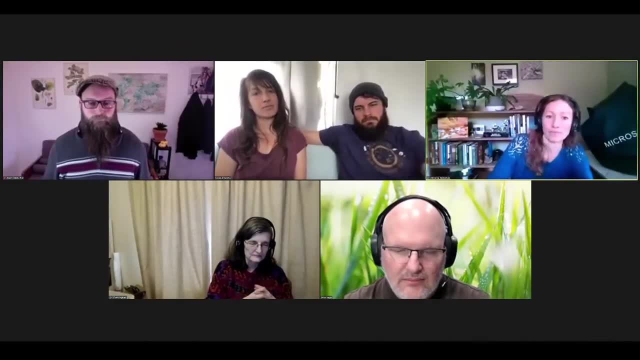 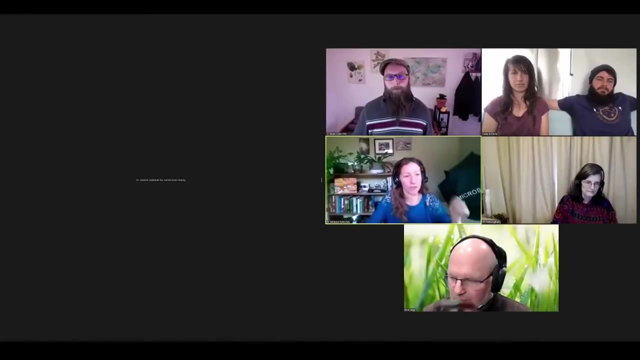 those dots together, elaine? um, so in order for folks to be able to have access to healthy uh compost, we also, um, we also need to help, you know, more folks have access to this good compost. so one question that we got is: do those rotating black bins work for people who don't? 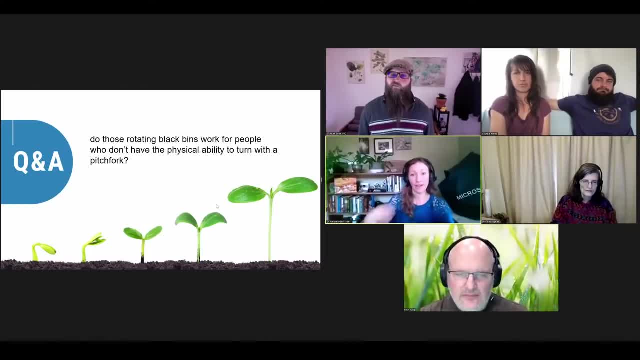 have the physical ability to turn with a pitchfork? and if yes or no, what else do you recommend for compost accessibility to make this a possibility for anyone and everyone? adam hit on that earlier. no with uh, adam, didn't you say? the best compass you've seen so far is from a teeny little, a teeny little worm. 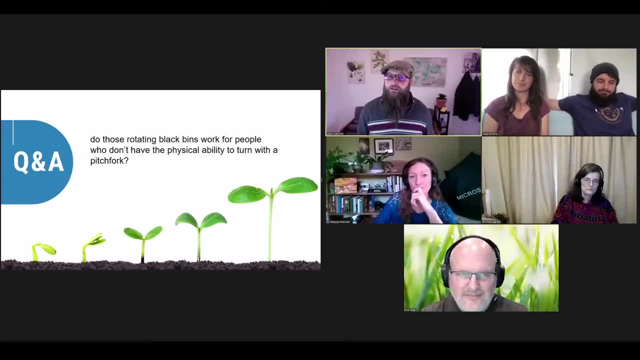 bin, yeah, but you can get great results out of that. um, but i i think that these are pro. is this question about the tumbler system? i think this is a tumbler system. yeah, you know, and i've used those before, but i i worry about the materials mixing so much that you can. you have the potential to get. 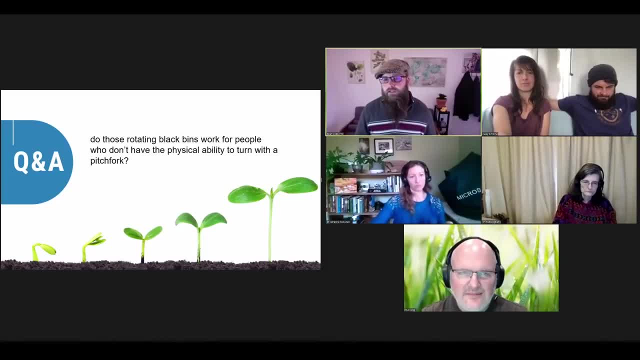 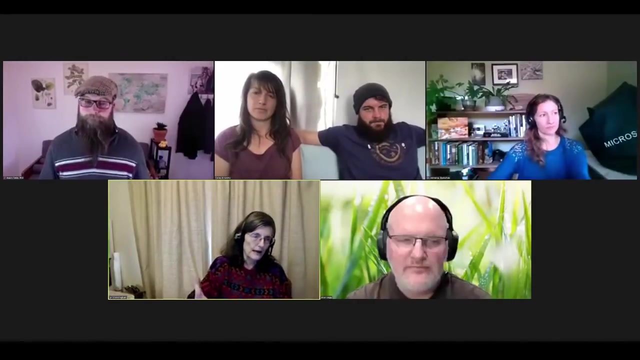 materials not heated up sufficiently, especially for weed, seeds and um and uh. you know, like i, i don't think they don't provide the same use for environmental purposes as the big pots. do you think that's good for people who don't know how to use them? and you're just being. 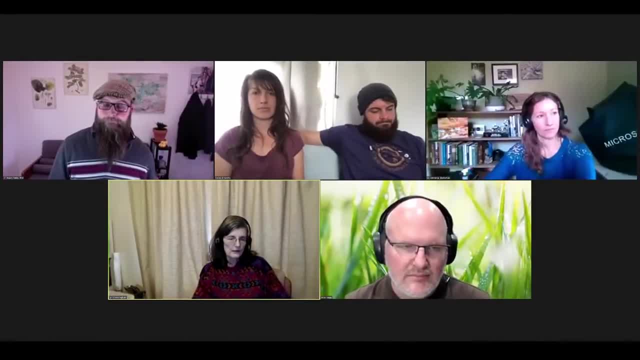 like you're just trying to dig new holes right, it's hard to find the right material for them. um, yeah, sure, sure, sure. so i think it's really important to make sure that the material that's going to be put in those bags is going to be kept in that bin, because otherwise you're just you know. 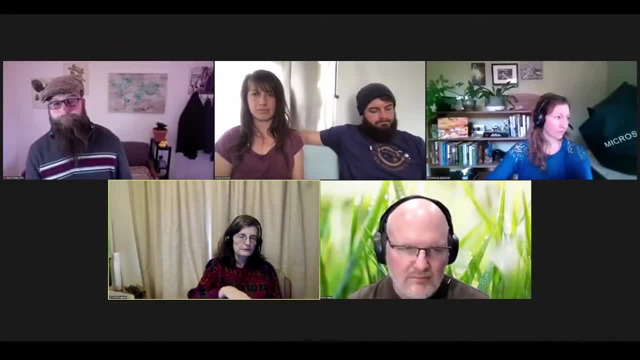 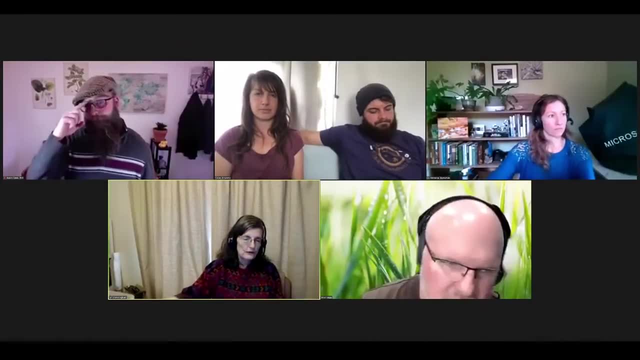 taking all the trash out of the bin, and you can't probably- uh, you know you're not going to be able- to wait until the worms have completely finished incorporating the last set of food that you gave them into the worm bin before you give them more. uh, people always have such horrible problems with 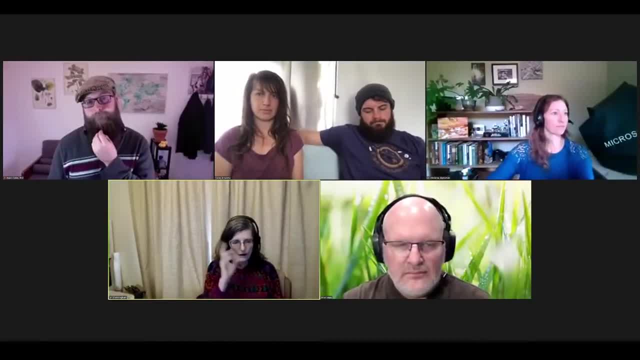 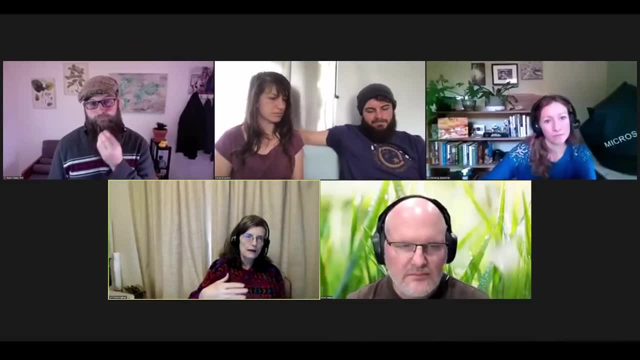 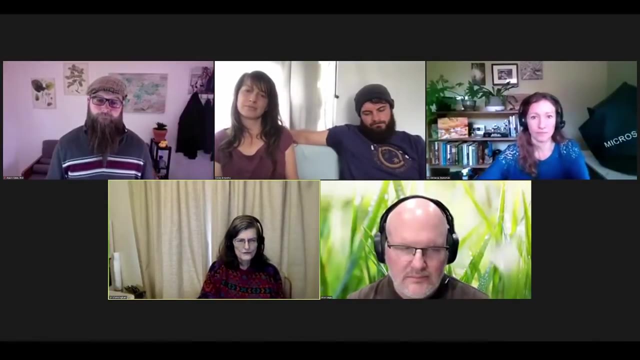 the white flies, um the. you know all that, yeah, all those guys that, um, you've got to let the worms do their job on their last increment of food before you give them more. so, and i i've also heard the mythology of you can't let worms go back and eat their own, um, worm. 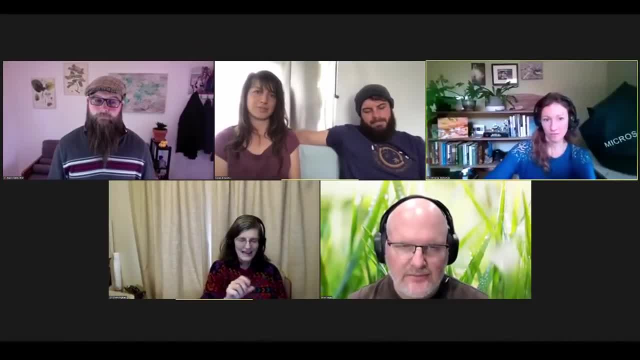 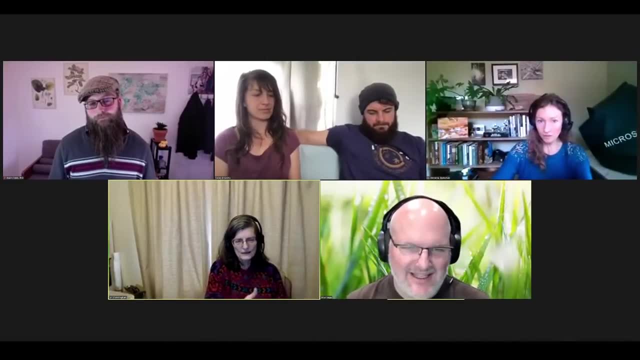 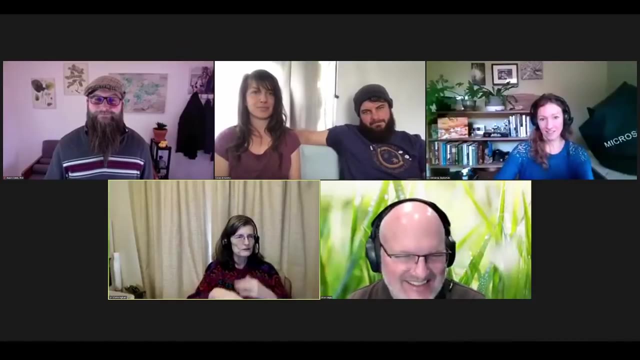 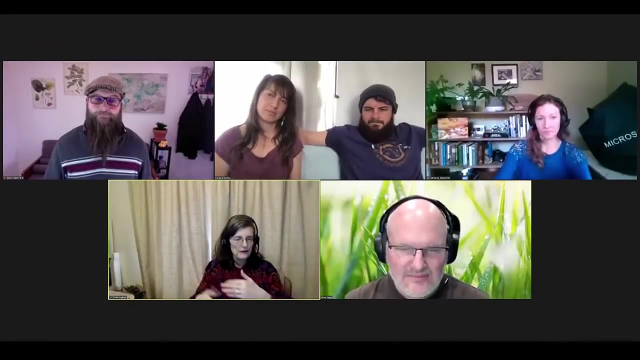 castings. thank you, um, you can't let them do that. that's why not. yeah, it's ridiculous. yeah, because i've. anyways, i leave when i go on vacation. i just leave my worm bin doing its thing. you know, the worms are perfectly happy. they just keep rerunning through all of the old compost that's in there and the 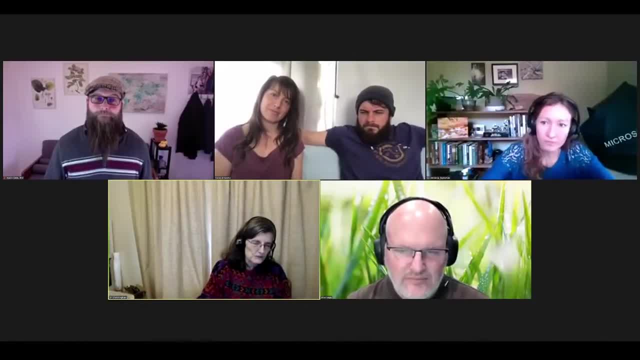 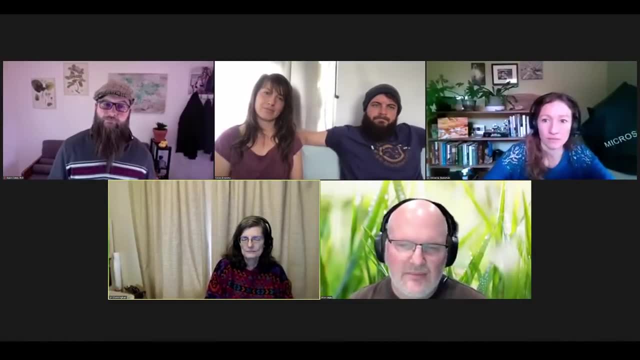 castings that are in there. come back, they're fine. just feed them as soon as i get home and life is wonderful, so i just can't buy that. um, you know, maybe the person who who wrote that up you know their worm compost went anaerobic. 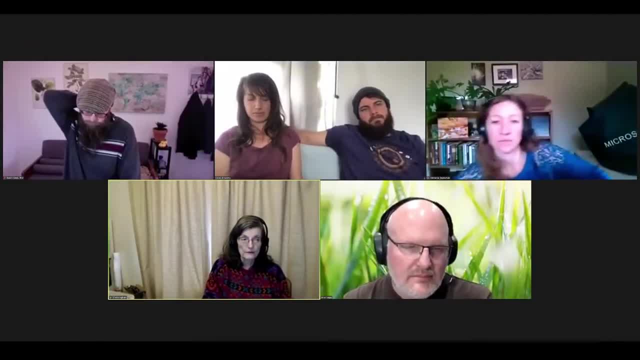 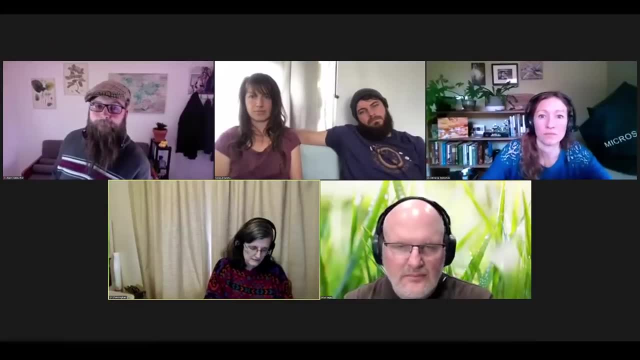 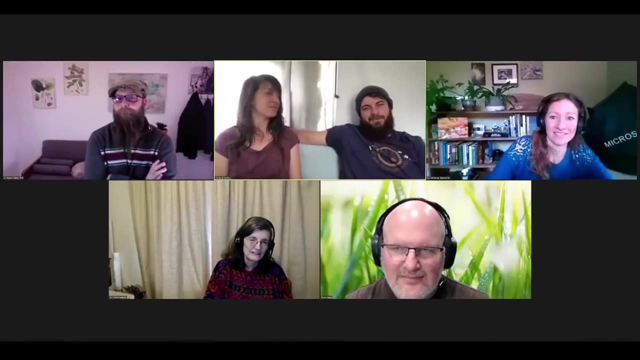 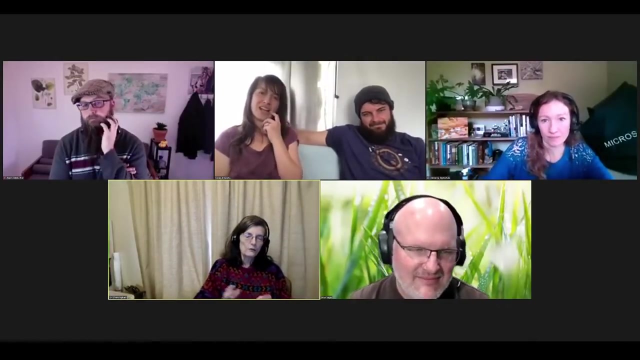 it was too wet. um, okay, that'll kill them. uh, not, it doesn't harm them to be reusing their own castings. maybe it's running out of food and i was like there. you know they can't run out of food eventually, but yeah not. yeah, well, if when i forgot and didn't feed the worm bin all the 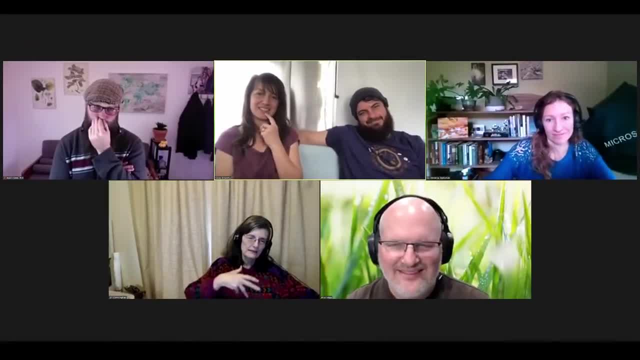 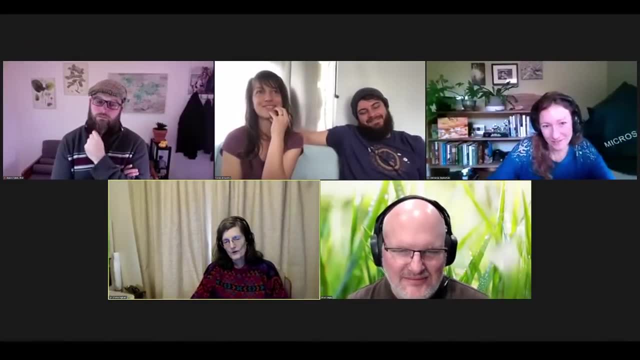 worms would just crawl out of the worm bin and get into my, my beds that are right there and next to it, you know so, oh good, the worms moved themselves over. i can start a few more. what i have noticed with a worm bin too: that it can take a minute to get it started. you just start. 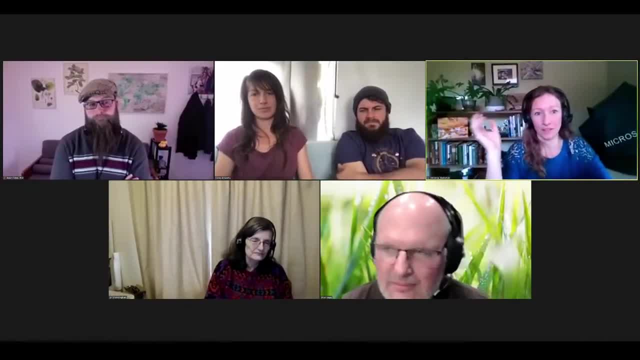 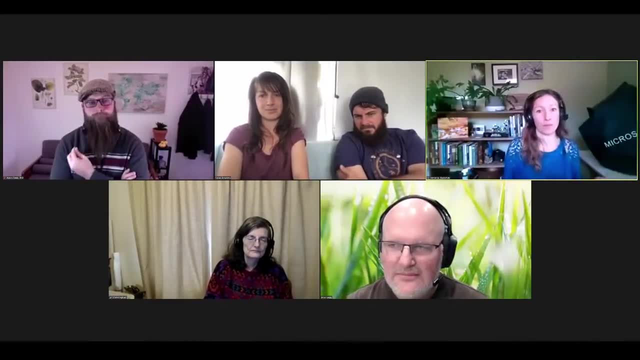 with, you know, some bell peppers and banana peels and you put some worms in there. it's not going to necessarily immediately have rapid decomposition until you have a solid microbial community built up there as well. so it is. i mean, one possibility would be to make a static file in your yard, or 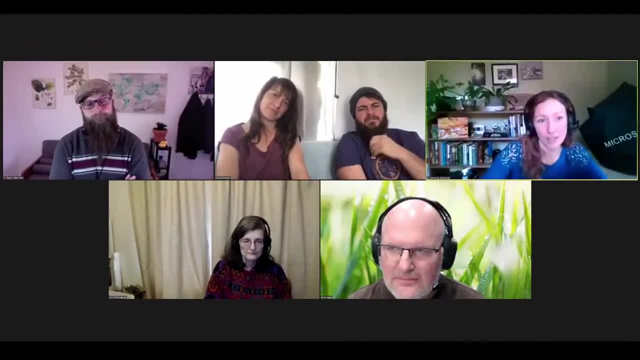 like a tub somewhere and then you can just put it in your yard and it's like, oh my god, i'm gonna. and then use that static pile that's had some decomposition time as a starter, because as soon as i started adding thermophilic compost, that was finished to my worm compost, my vermicompost. 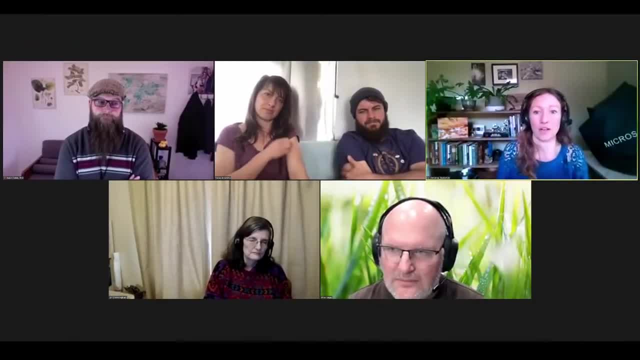 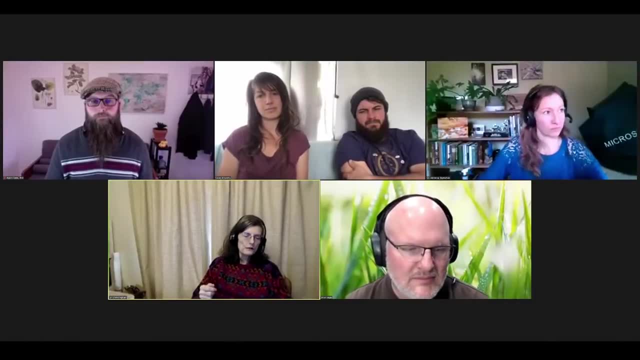 that's when i saw really rapid decomposition and a solid microbial community. yep, and then like, if you're gonna do some composting in a tub, poke a lot of holes in the bottom of the tub. go put that out someplace, you know, like on a bed or something, and pretty soon you've got worm compost. 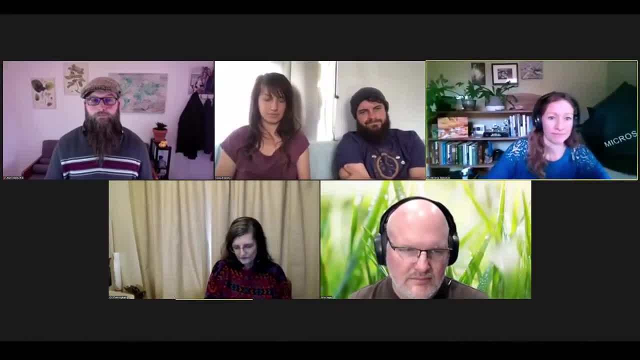 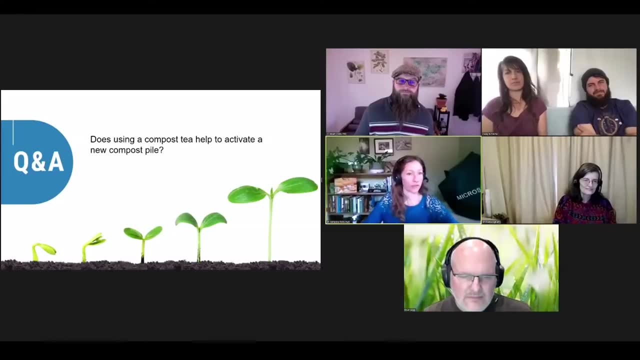 mm-hmm, because the worms will come and join you. so have fun, all right. one final, final question. we had a lot of wonderful questions. this one is: does using a compost tea help to activate a new compost pile from doug or an extract? it's easier, or an extract would be easier? how? so tell me about it. we do that. 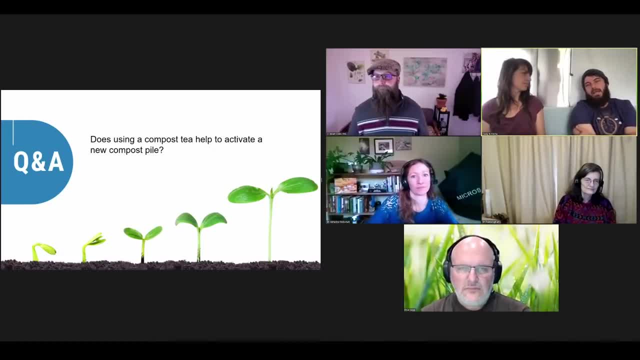 often where, uh, if we have a good compost pile, we can extract from that compost pile and i'm going to actually spray it onto other ones that aren't doing quite as well, just to inoculate them back up. um, go ahead. you just never know what, or you know what organisms are coming in, especially in the 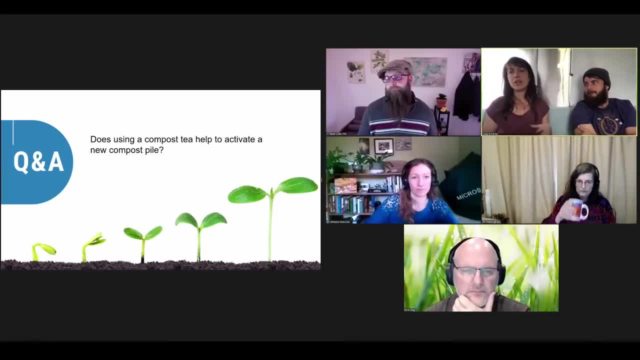 beginning, when you're collecting all of your diverse input materials, you're hoping that they're covered with microorganisms. unfortunately, some places on this planet are not as diverse as they used to be, and so if you have a verified source of compost that you can make an extract or tea. 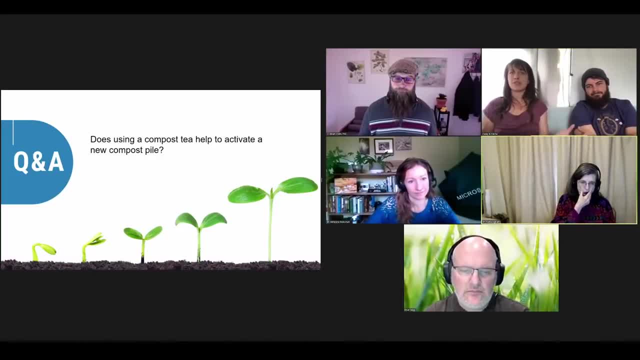 out of it's. it's just like getting your livestock in place if you're thinking of it as a farm. so it's. it's not a bad idea, that's for sure i was. this technique of extracting, um, some of my farmers don't buy a lot of bulk. 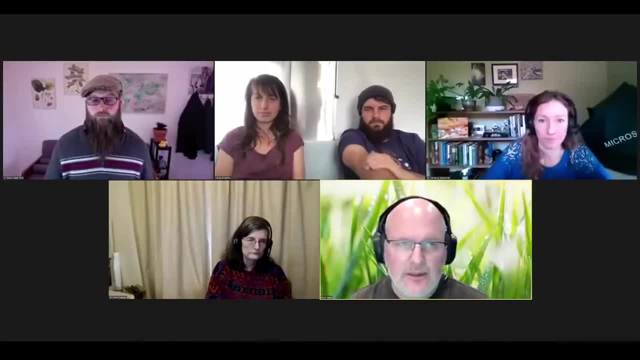 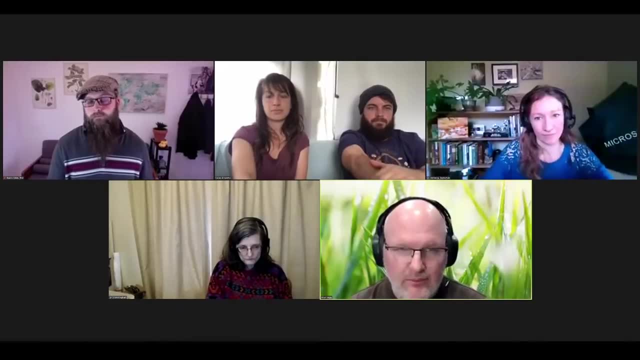 compost. you know, because we're going to put six tons or ten tons of the acre type of thing and you got thousands of acres to do and the microbial communities in that bowl compost are horrible or not, they're not present. so we'll do an inoculation with an extract into that compost, maybe with a. 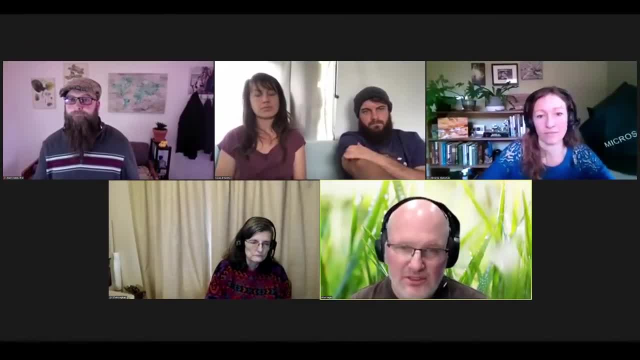 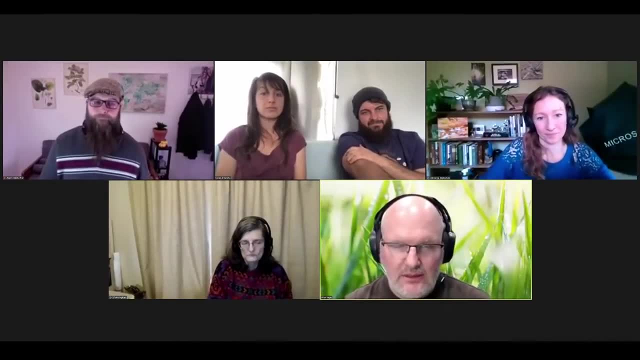 little bit of food source too, to try to get them to establish, start doing a little bit of growing. it's never going to be, you know, as good as the biologically complete compost that, uh, like you're, you're having to start with, that's for sure. but that part again, i'm curious a lot about the 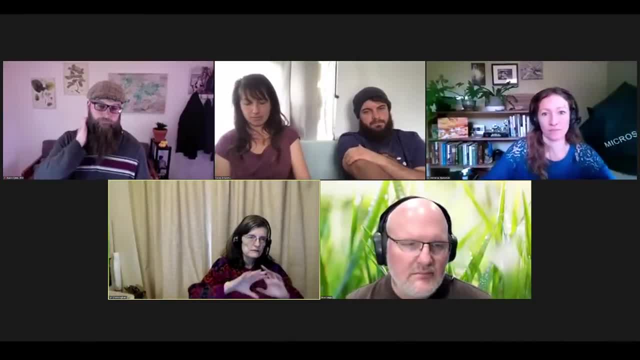 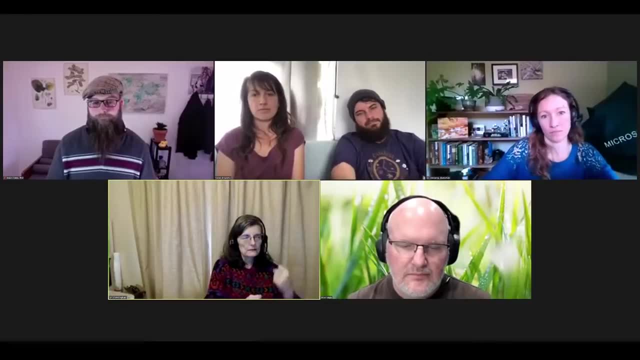 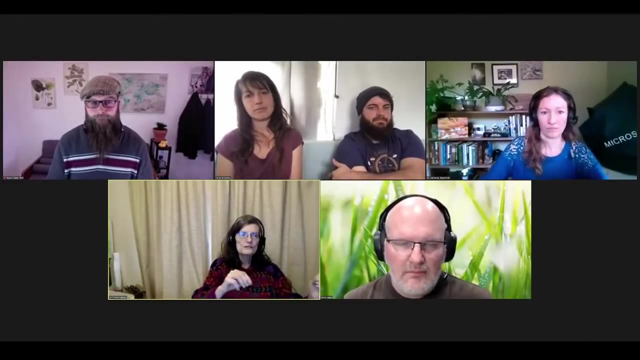 quality of it, how it's. it's a part of the process of doing a compost a lot of the time, like you guys make, but at least it helps it along. and the only reason to use a compost tea, in my opinion, is if you need to spray the biology onto the foliar surfaces so that they will stick. 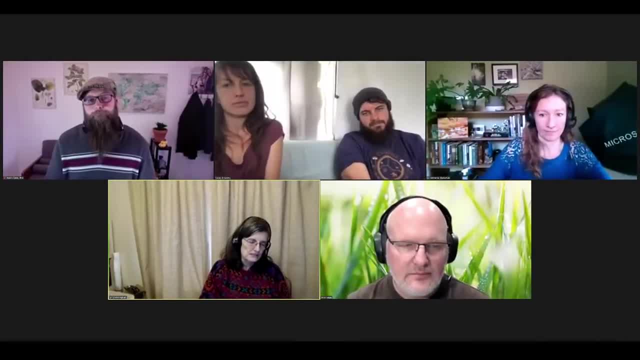 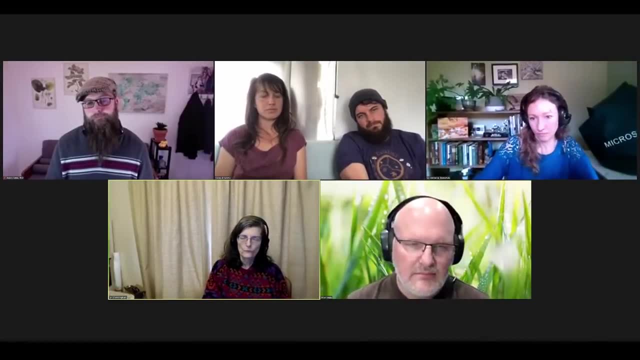 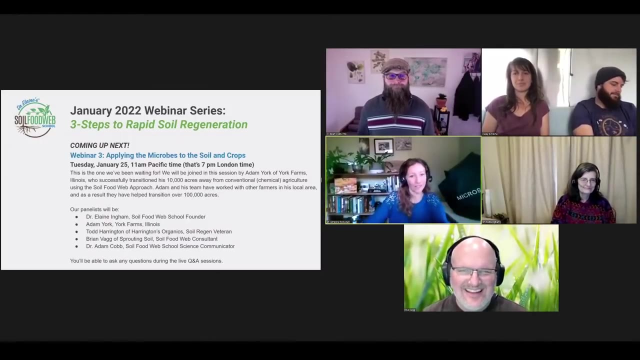 that little bit of extra food that you put into a tea is going to get the bacteria and the fungi. really, the only time where a compost tea is is worth making, in my opinion, otherwise extract. thank you, we're going to learn more about how to get those microbes out onto a field. 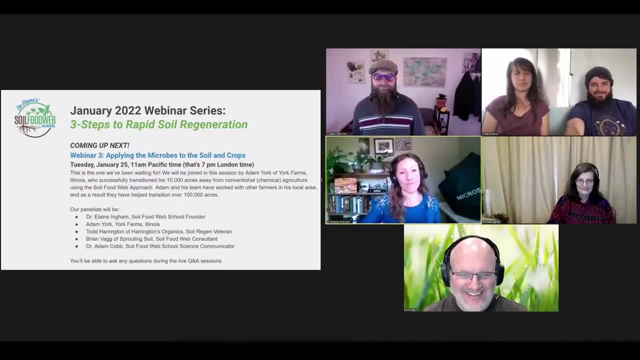 so applying the microbes to the soil and crops um on january 25th. so for all of you, if you enjoyed today, please come. you'll get to see a little bit more about some of the same things, some of the same videos, some of the same people, but new ideas, new concepts and sometimes, when you hear things, 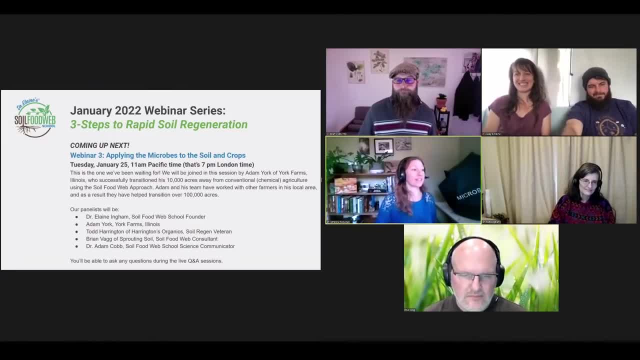 again, it can just click that extra, extra little bit. plus, we get to hear from adam york, todd harrington, brian beg, dr adam cobb and, of course, our one and only dr elaine ingham. um, and so i'm very excited for this next webinar as well. but before i leave us today- and we are at the top- 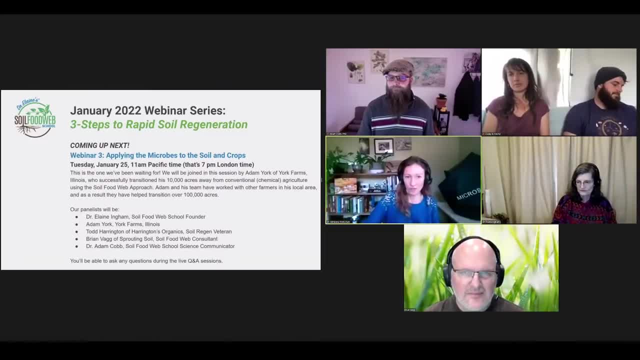 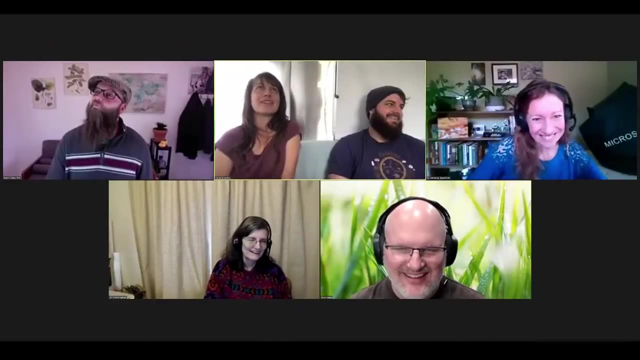 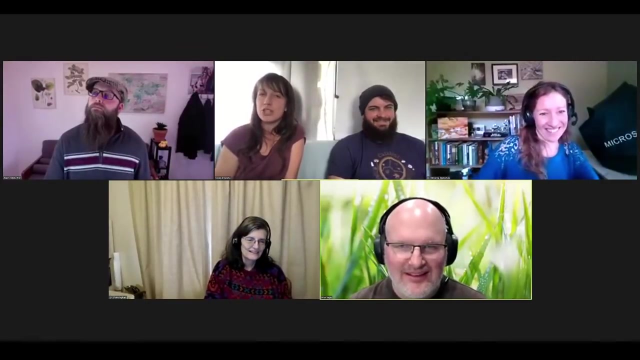 of the hour, but i would- i'm curious to hear from each of you what is the strangest or most fun ingredient you've ever gotten to work with in a compost pile fun spot earlier, i probably would have had a really good answer right on the spot. we found a chainsaw one time in a pile of wood chips. oh wow, that is probably. 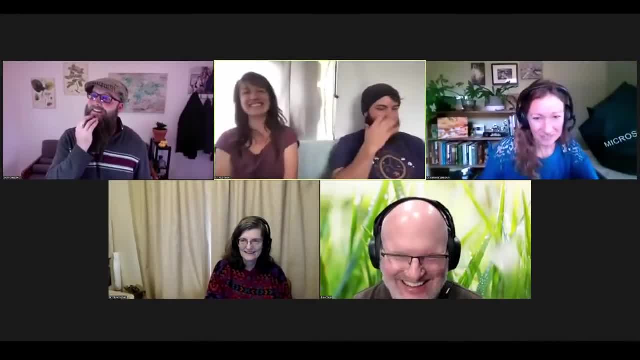 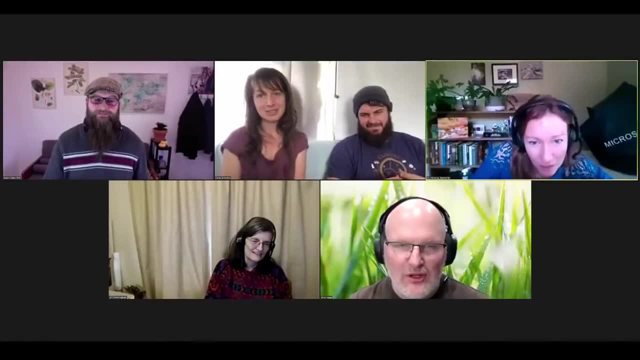 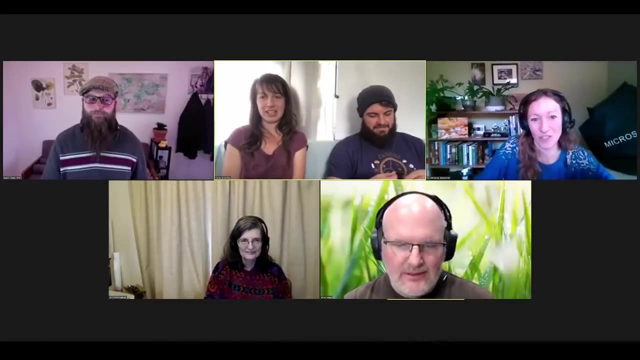 compost. well, i love that other folks are contributing as well. we have some um the strangest i've used pond material, so material zola that grows in ponds, things like that. oh, dog hair. yeah, this is great than we do. i know. yeah, exactly, yeah, what else? 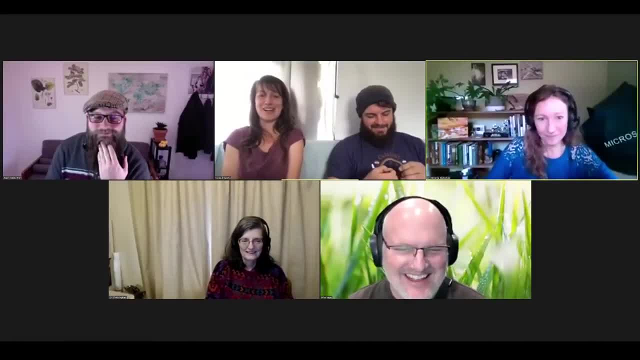 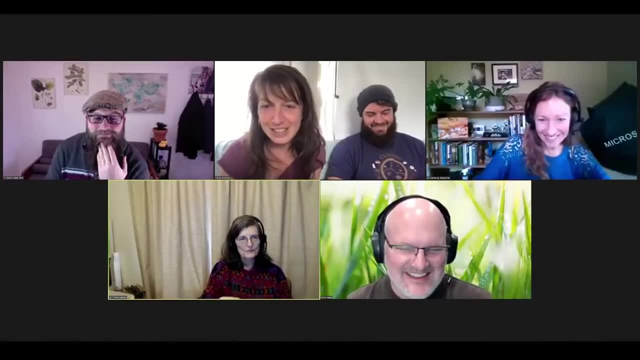 then rats. yep, that's you guys, here you go, especially when you get materials from the city, for example, they, you know, they'll bring out all of the leaf material and they'll bring out all of the leaf material and they'll bring out all of the leaf material. 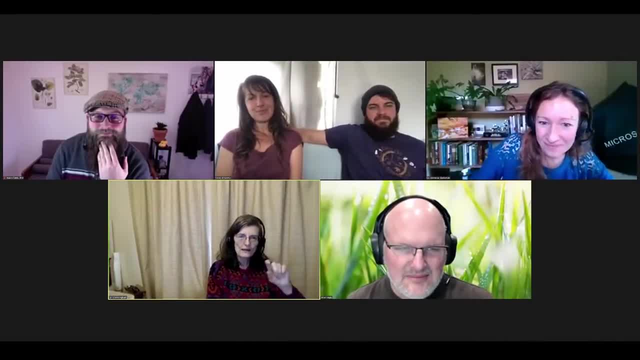 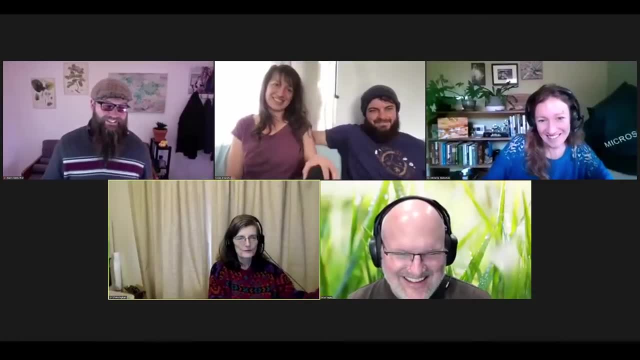 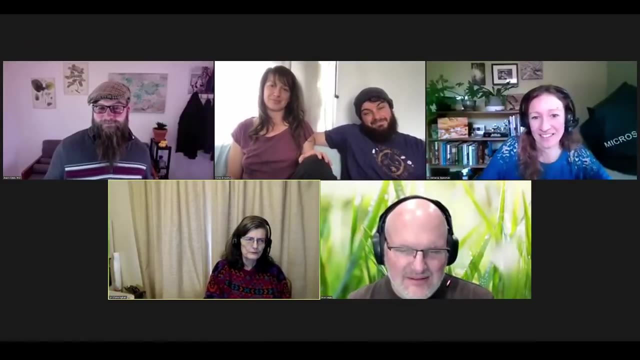 and dump it on your property. and we have. i think we had a whole set of the star wars figures- oh my gosh- and mickey mouse and minnie mouse, all from stuff that came out of the, come out of the, that, that kind of material. it's just, it's astounding what people throw away and and they 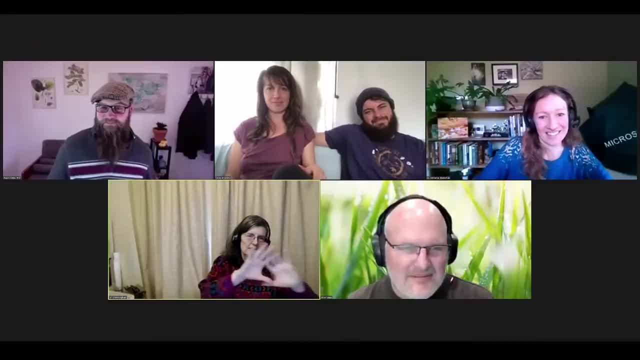 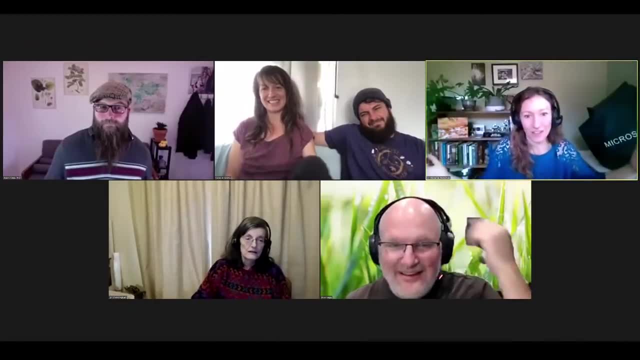 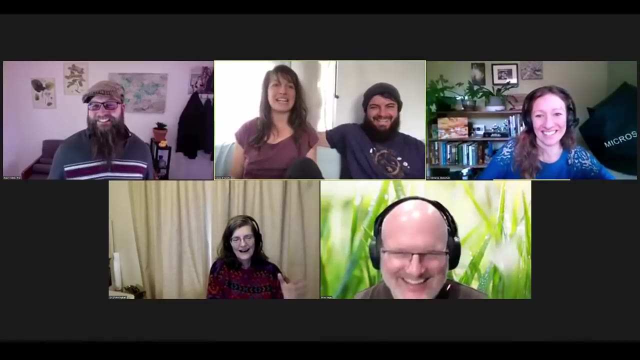 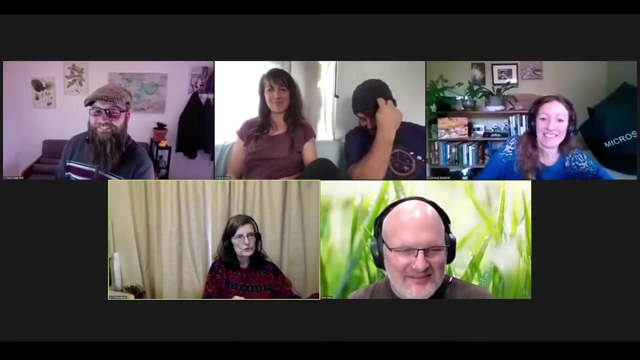 they obviously cannot read because you know the the container says brown leaves only. hey, but you won. you got the star wars characters. that's great. yeah, i was going to ask if i could come get those from your attic, dr elaine, we're less money now. i, i left them in at rodeo, sorry, yeah, the other. well, we would sort materials. 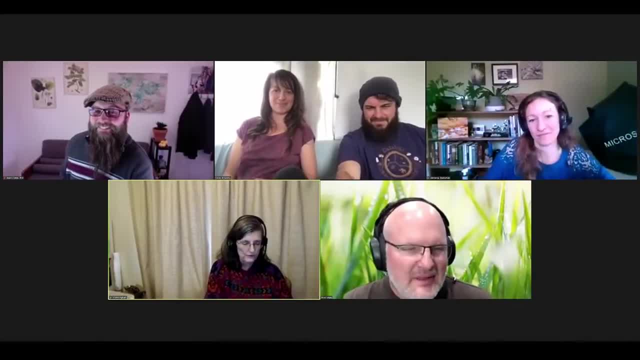 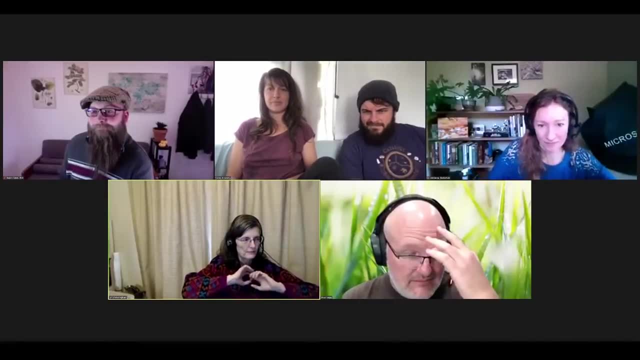 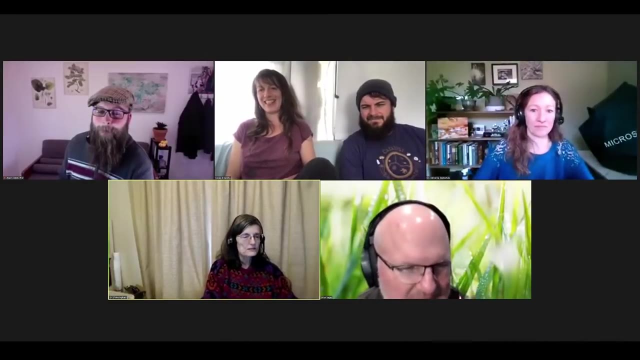 for a worm composting operation or they would sort things. and, um, when we were there one time, um, all of a sudden there was this: uh, you know the, the danger sound went through the, through the building. we all had to evacuate because two of the guys um picking the garbage out found two um grenades. 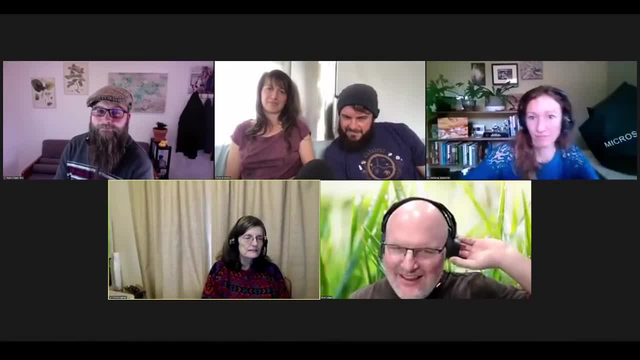 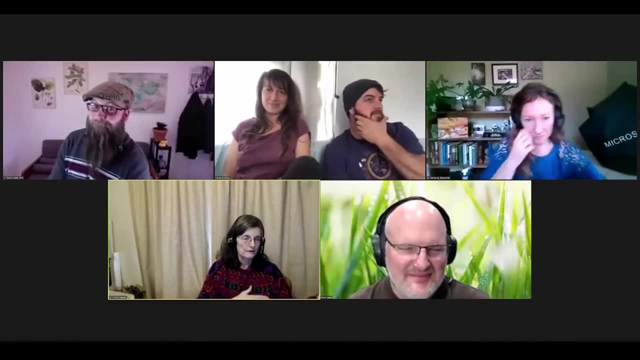 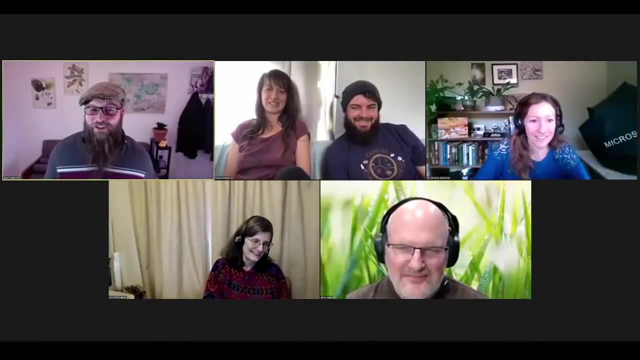 pins still intact, thankfully. but in those, in those conditions you fall, you have to fall. call the bomb squad. that's intense, yeah, yeah, don't mess up with those. so you're saying that hand grenades are not a recommended method of turning a compost pile? that'd be a green material. 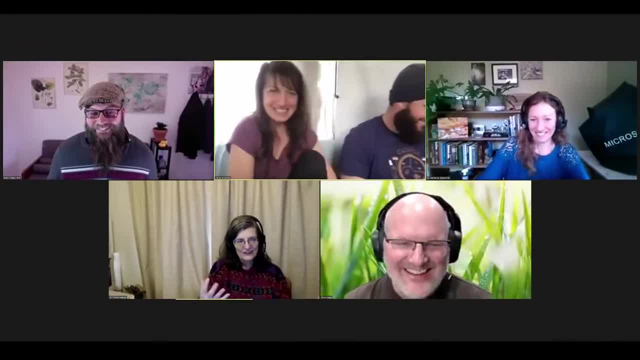 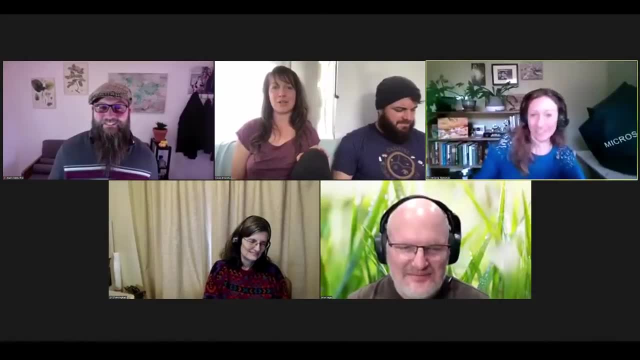 or it kind of ignites all your organic matter. you have none left after these. yeah, that's too much birthday right there. yeah, all right, well, let's. we're gonna wrap it up here. thank you all for sharing the fun and wild things you found in your compost piles or 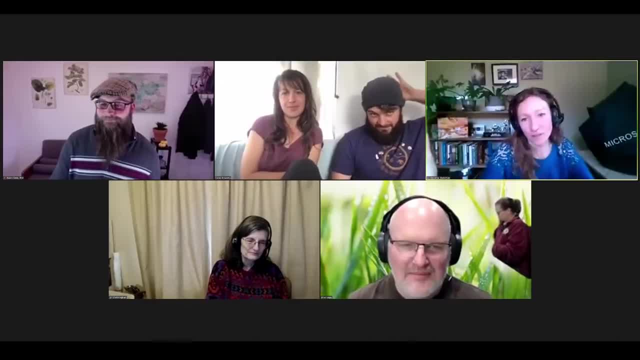 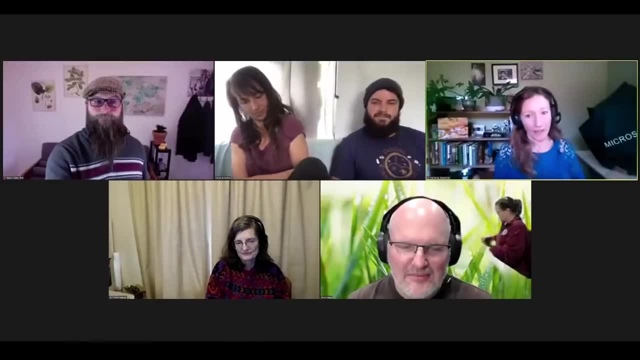 composted, and thank you for wanting to be out here and help us to regenerate soil. it really makes a difference. the more of us that we have helping to communicate what healthy soil biology is and how to grow these organisms, the more the better it's going to be for us. 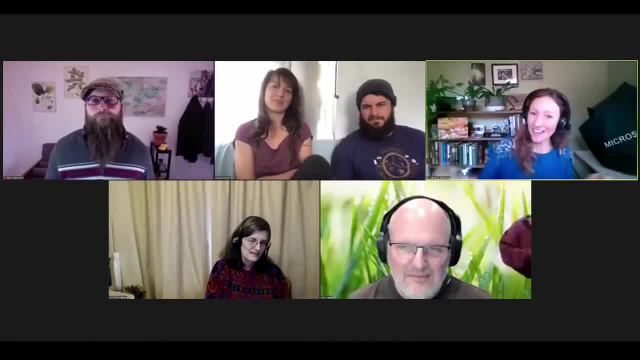 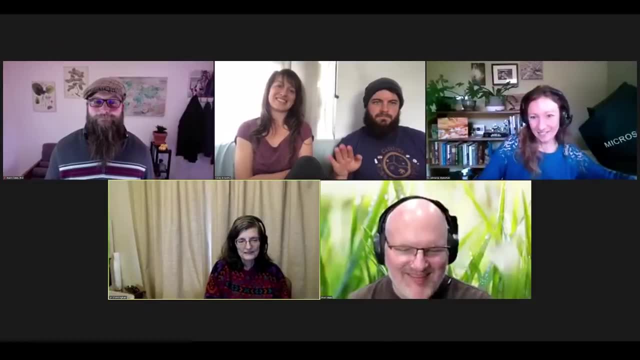 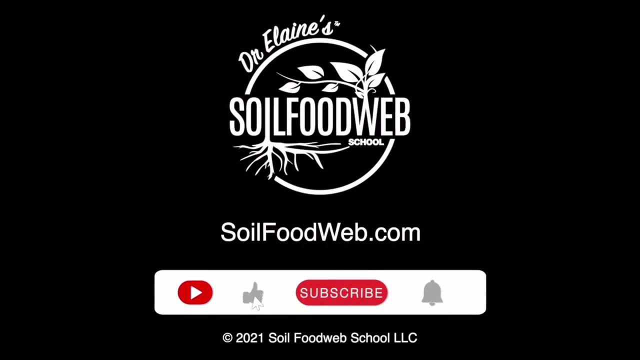 so we can make a difference all together. so thank you for being here and we'll see you on january 25th, and please come join us in learning more about the soil and all of the organisms that are there. don't forget to click that like button. subscribe to our channel. 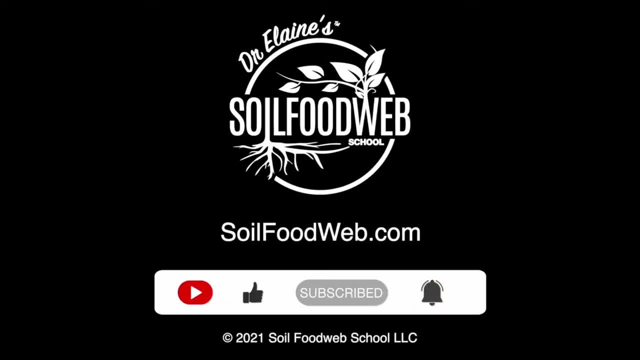 and ring the notification bell to stay updated with all our new videos. you. 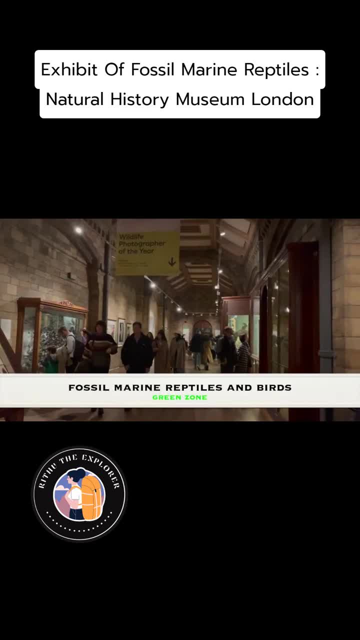 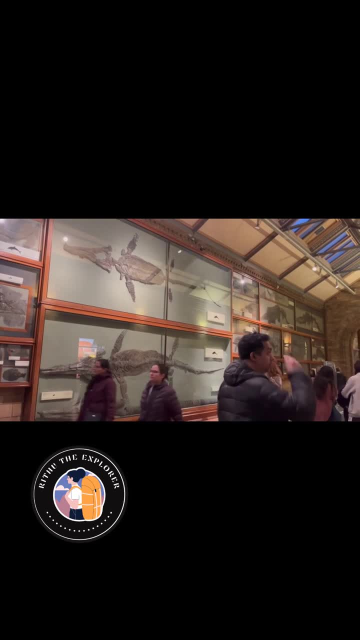 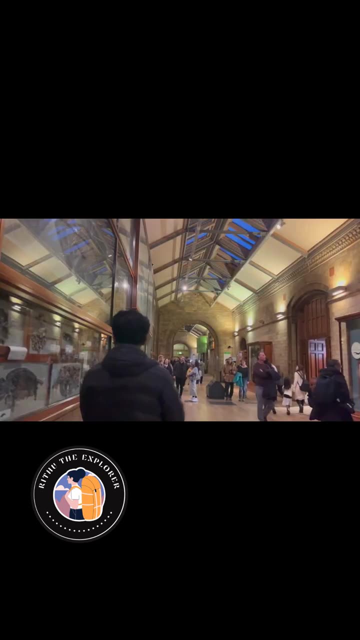 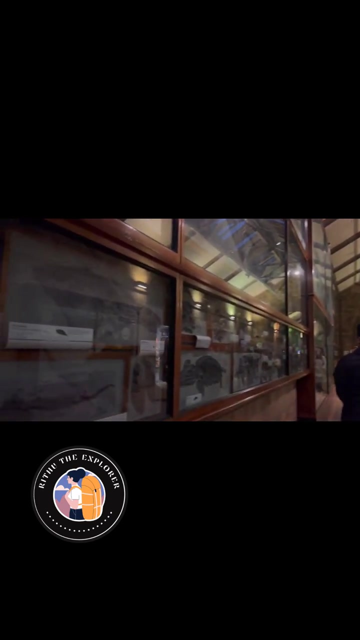 We proceeded to the Green Zone, where we encountered the exhibits of fossil marine reptiles and birds. The Fossil Marine Reptiles and Birds exhibition in the Green Zone of the Natural History Museum in London offers a captivating journey through time, showcasing the ancient inhabitants of Earth's seas and skies. This area is dedicated to the fascinating world of 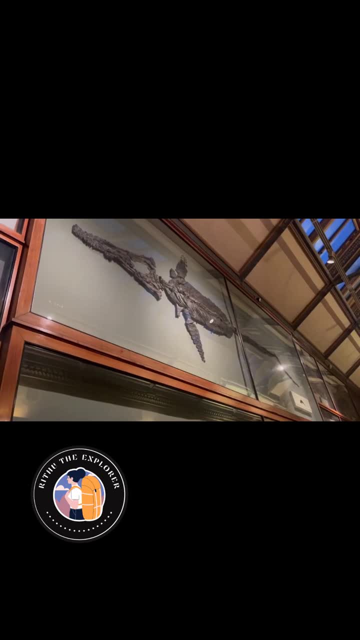 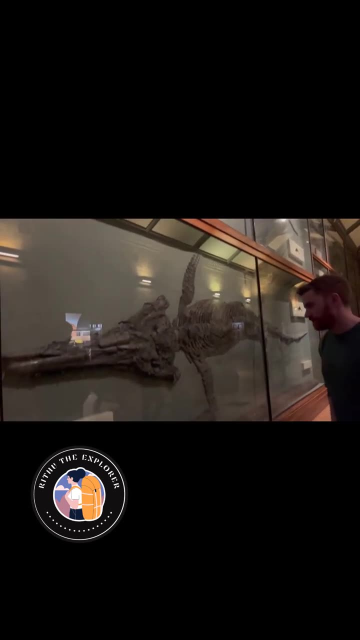 extinct marine reptiles and the diverse history of avian evolution, providing visitors with a deep dive into the prehistoric past. The Marine Reptiles section unveils a collection of fossils that trace back to the age of dinosaurs and beyond, including ichthyosaurs, plesiosaurs.